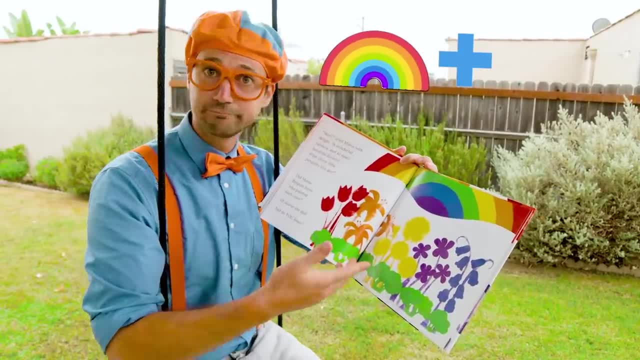 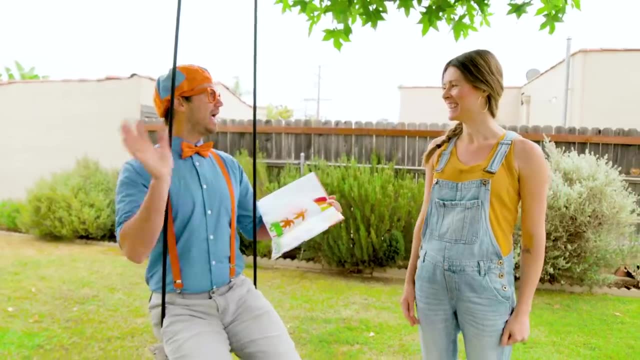 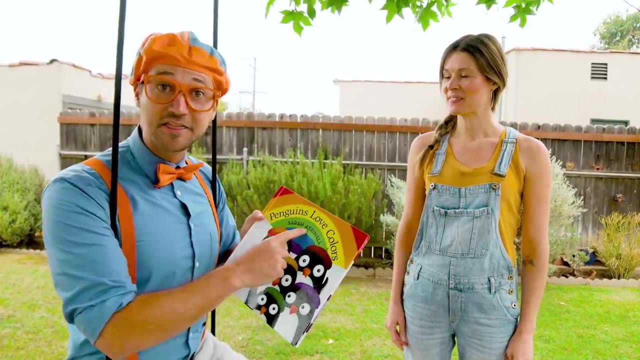 Hey, Rainbow plus garden equals rainbow garden. Hi Blippi. Oh hey, Who are you? I'm Sarah Aspinall, Sarah Aspinall, Sarah Aspinall- Wait a second. Like the author and the illustrator of this book. 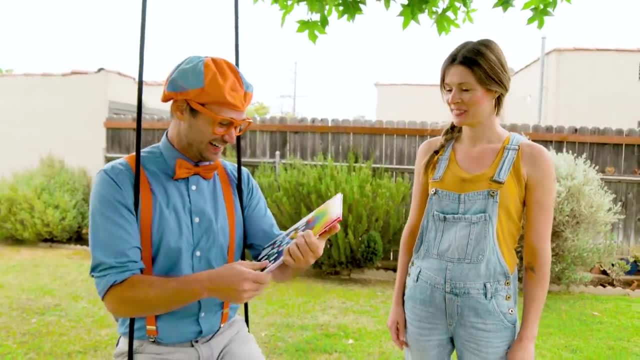 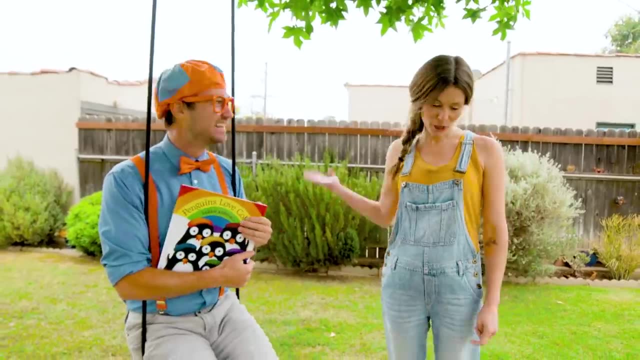 That's me. Whoa, That is so cool. Would you like to make a rainbow garden of your very own, Blippi? Yeah, I think that would be so much fun. Well, come this way. I've got all of the things you need. 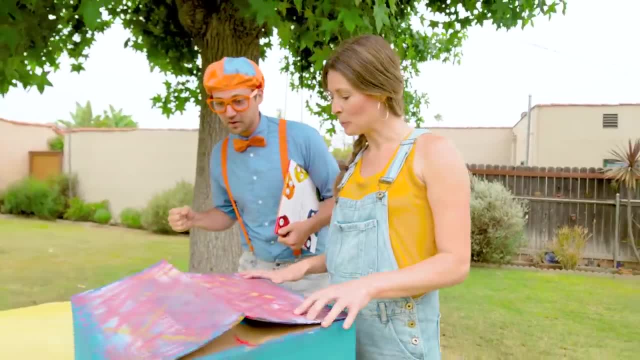 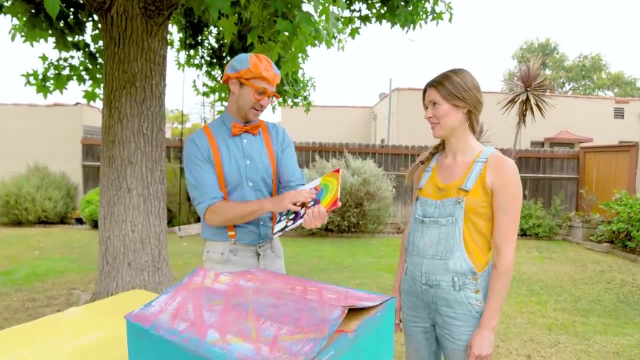 Ooh, All right, Here is a box full of lots of fun art surprises for you to have your very own art adventure. Wow, Well, thank you so much, and we are very excited. Thank you, We are very excited to make our very own rainbow garden. 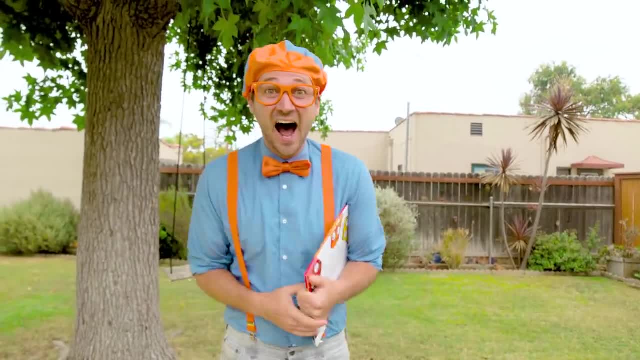 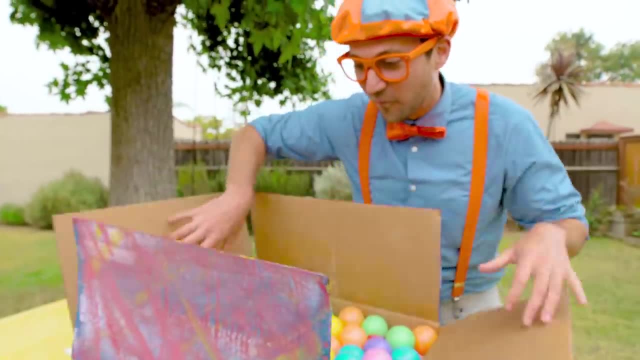 Have so much fun. Blippi, All right, See you later. Bye, Are you excited? Yeah, I sure am. Let's do this. Whoa, All right, Let's find all the things that we need inside this box. 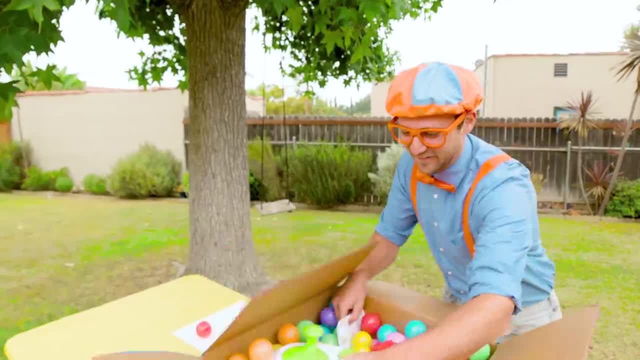 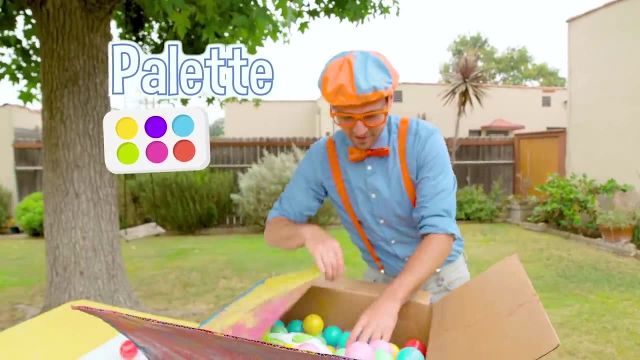 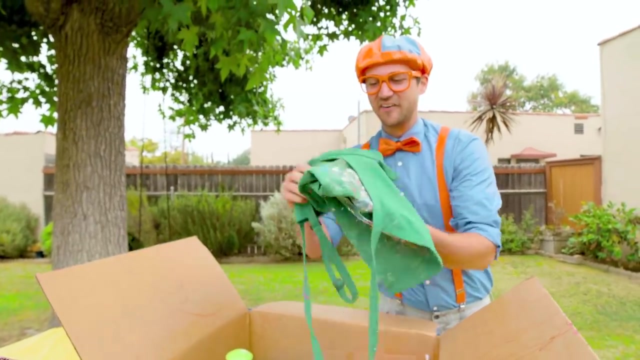 Whoa, Yay, Oh, wow, Ooh, It looks like we have a white palette. Okay, That right there. Wow, Wow, Whoa, Oh, Wow, An apron, Yeah, a green apron. It actually has a lot of paint on it. 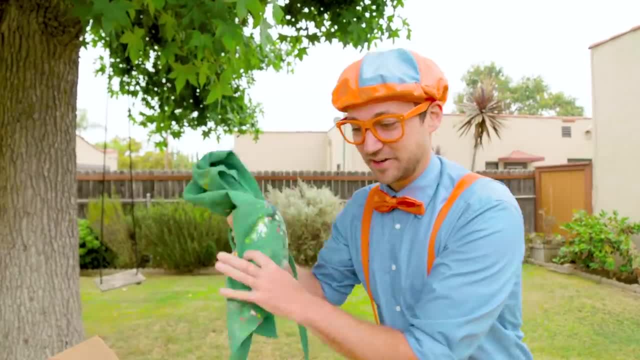 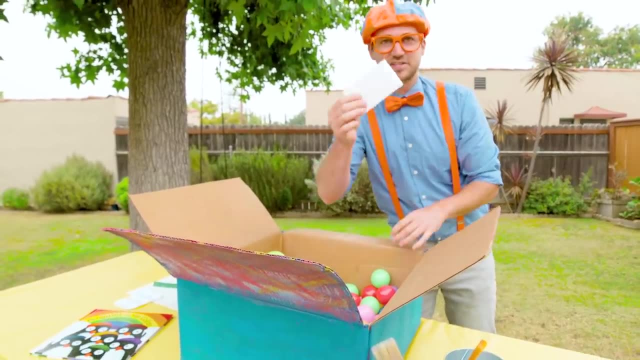 I'll set that right over here and we'll put that on before we start using all of the paints. Whoa Hey, A sponge. Okay, Put the sponge right there. Ooh, A salad spinner. Whoa, Wow. 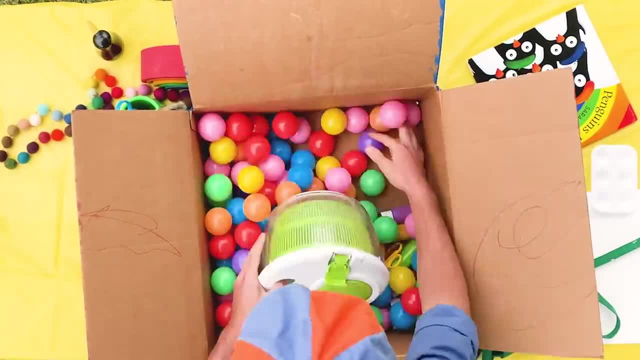 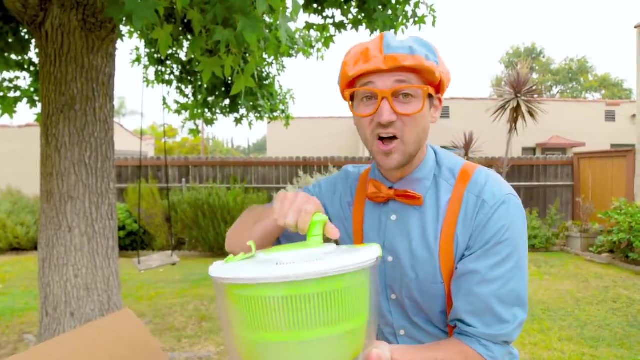 Let's see what we've got here. Oh, What is this? Oh, A little bit of a sponge. Oh, I love it. Oh, Oh, I know what this is used for. I'll show you really soon, Okay. 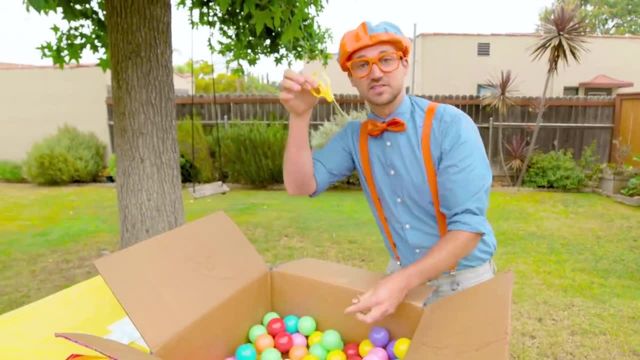 And we have some scissors, a little paintbrush and, of course, a lot of paint. All right, I think that's all. Let's see. Yep, That's all. Okay, Let's put on this apron. So then we're ready to go. 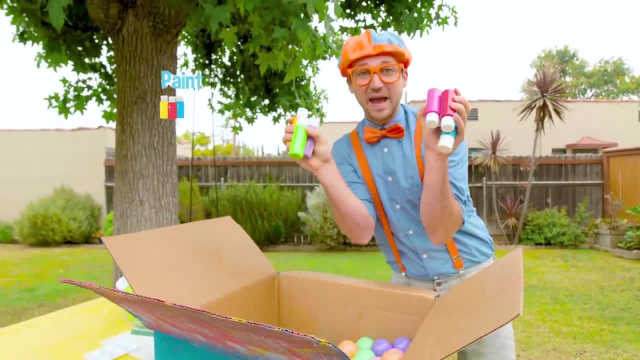 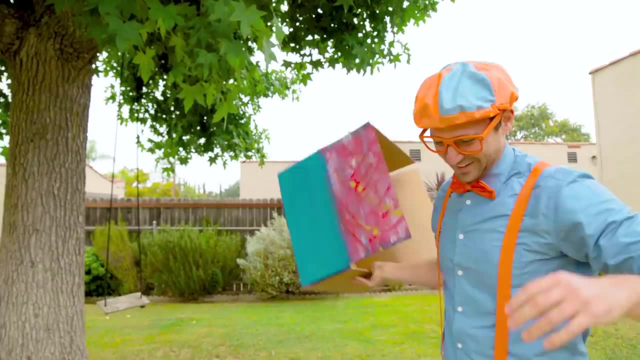 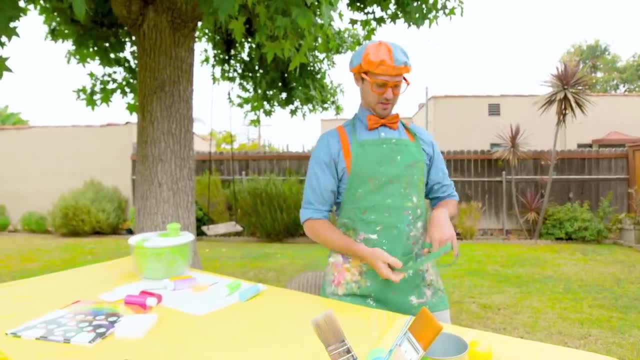 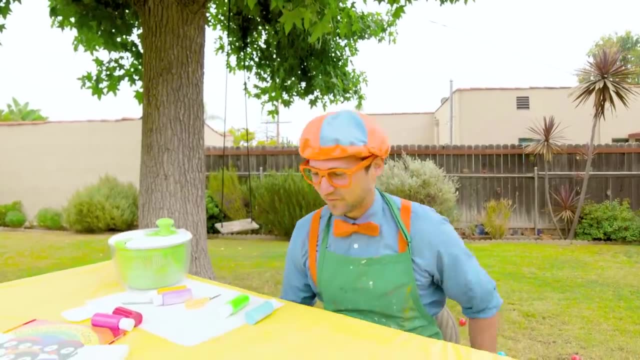 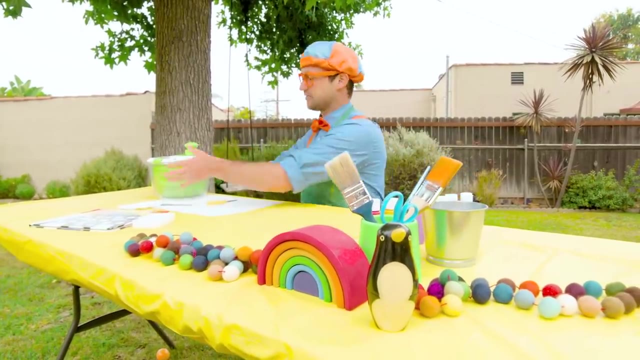 All right, I don't get dirty. All right, Here we go, Tie it nice and tight, Perfect, There we go. All right, Okay, Let's organize a little bit. Whee, All righty. Okay, So we have our paint over there. 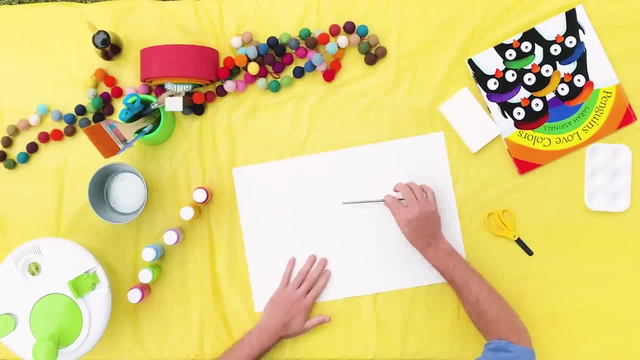 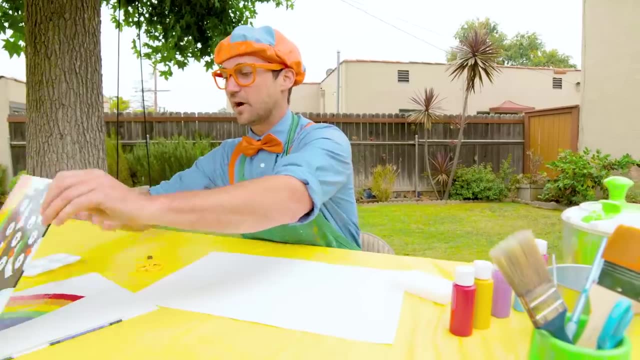 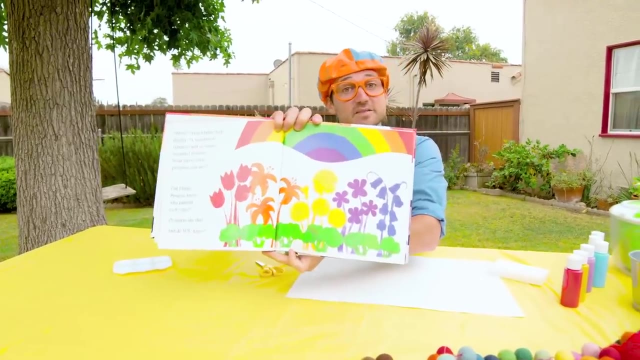 Salad spinner. right there, Big piece of white paper, little tiny paintbrush. Put that in there. Can't forget about the book, so then we can reference what we're making. How about that? Yeah, perfect, Yeah, remember, We're making this picture. 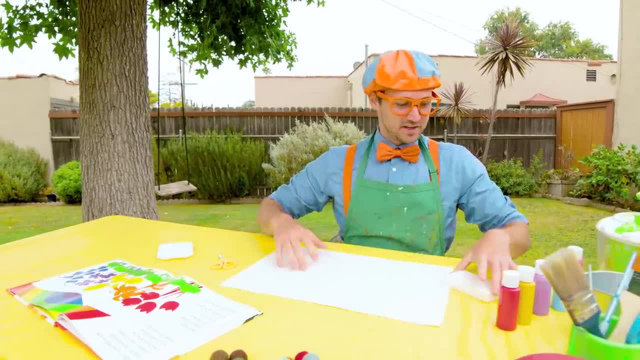 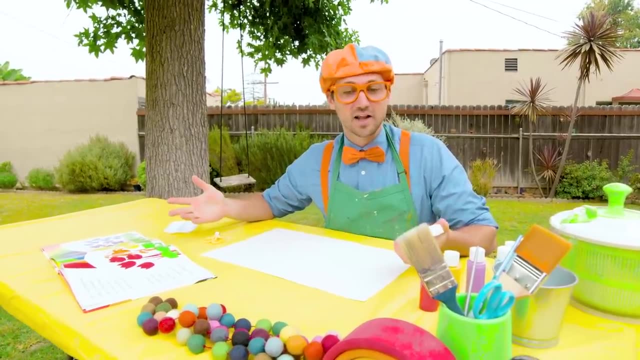 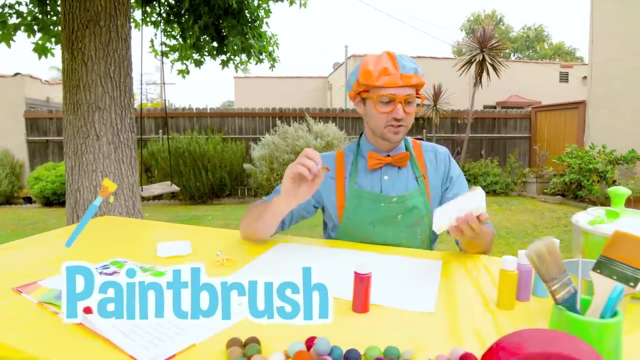 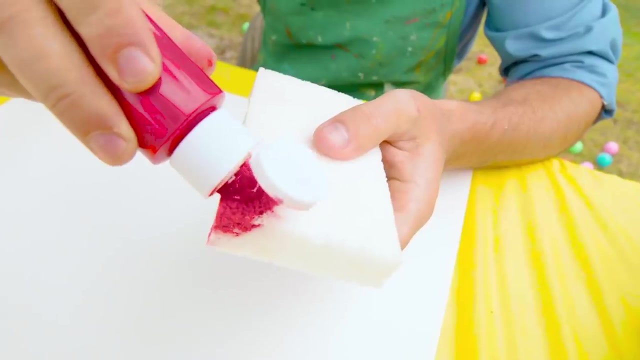 A rainbow garden, All right. So first we need to make a big piece of paper of rainbow colors. So let's take a little bit of red and a paint brush And we're gonna put it on the sponge, okay, So let's actually just squirt it right here. 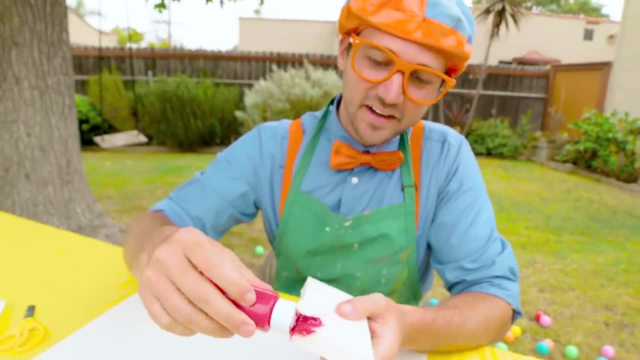 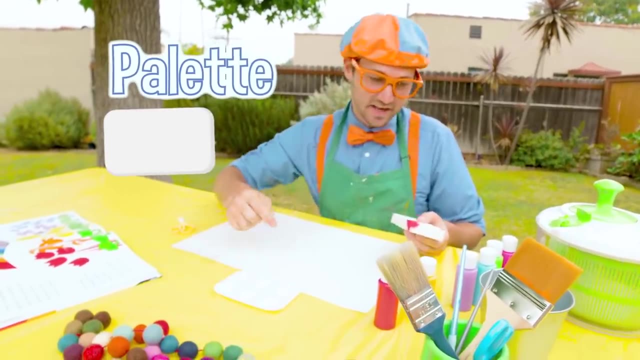 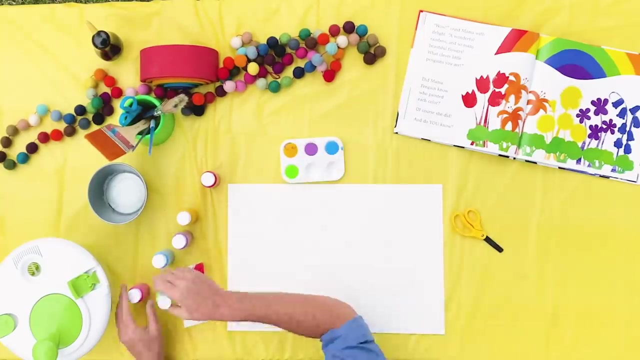 Okay, And now that we have a lot of red right there, we need to do all the other colors. But I actually have an idea. I think I should use this palette and fill it up. Might make it a lot easier, Perfect. 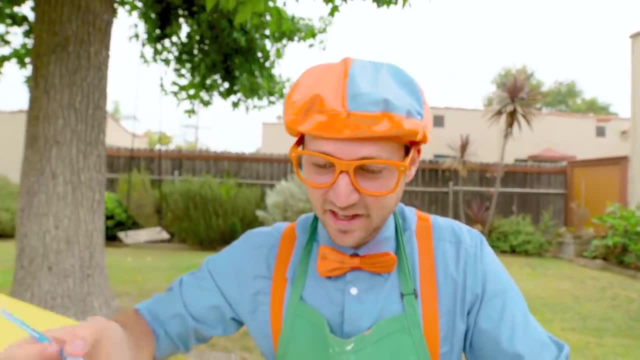 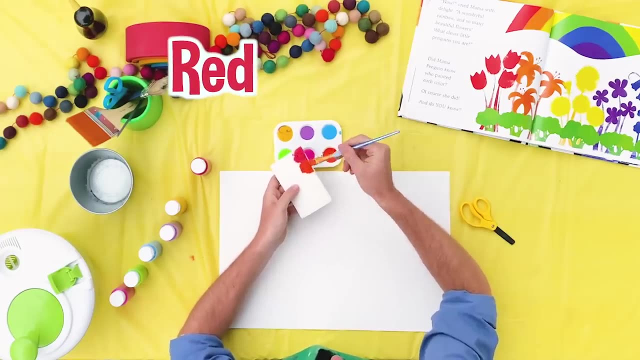 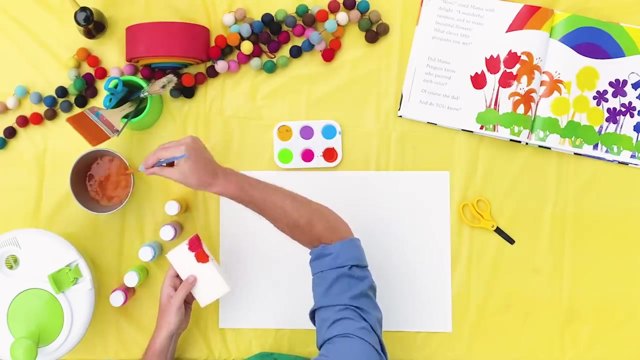 Okay, now let's take the paintbrush and put it on the brush, All right, And let's put some orange right here. Yeah, So now we have red and then orange Wash off our brush, Perfect, And we need some yellow right here. 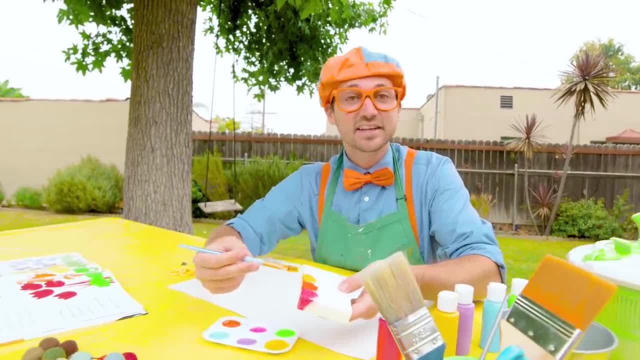 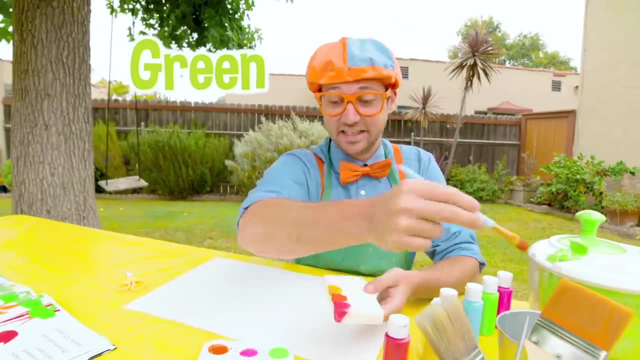 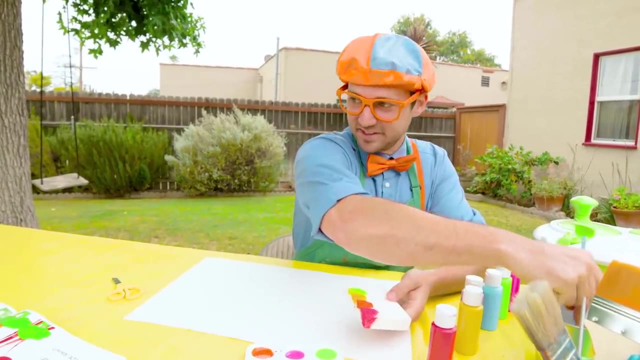 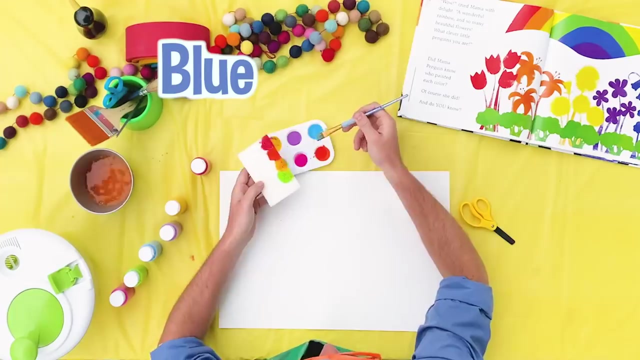 Wow, Yellow is so pretty. It's like the color of the sun. Okay, Lots of yellow right there. Now we need some Some green. Okay, Whoa, Green Perfect. After green, we need some blue, Yeah. 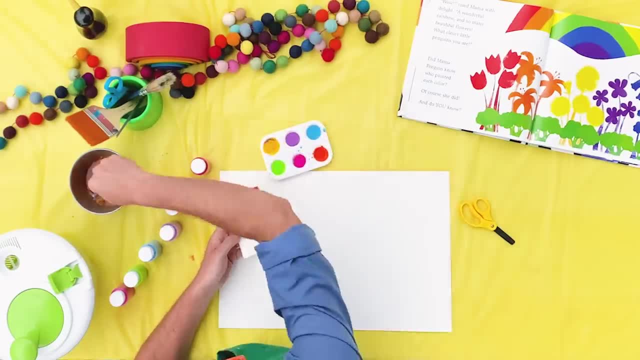 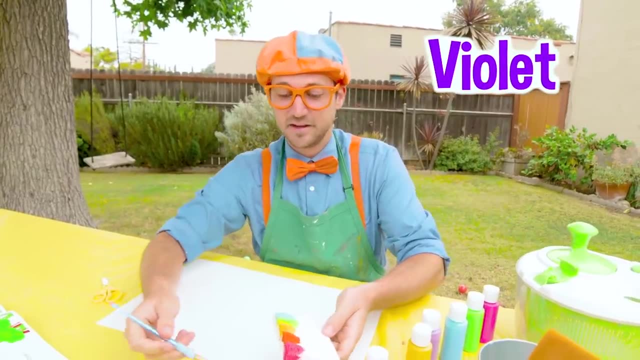 Perfect, Good amount of blue right there. Do you see this? We're almost done And now we need some violet or purple. They're very similar in looks. Wow, There we go. How does that look? Yeah, Like a rainbow. 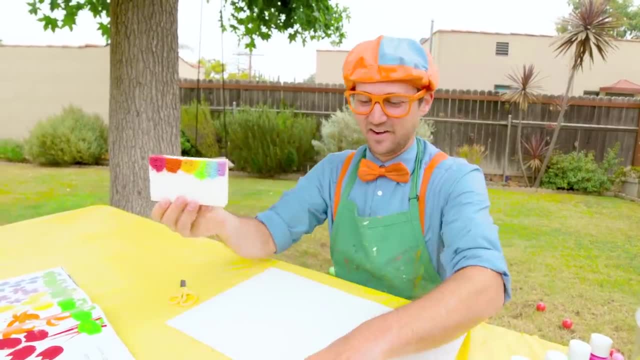 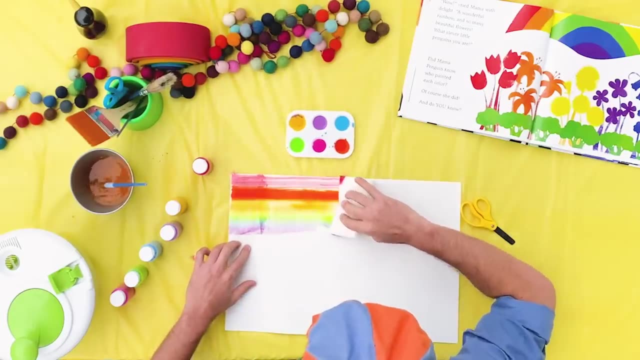 All right, Now for the fun part. Push it down right here. Yeah, Whoa, Look at that, Wow, Yeah. And you do that same thing many times in a row, All the way down. So I'll do that now. 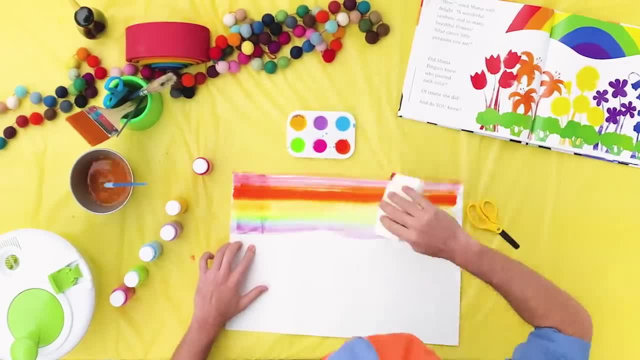 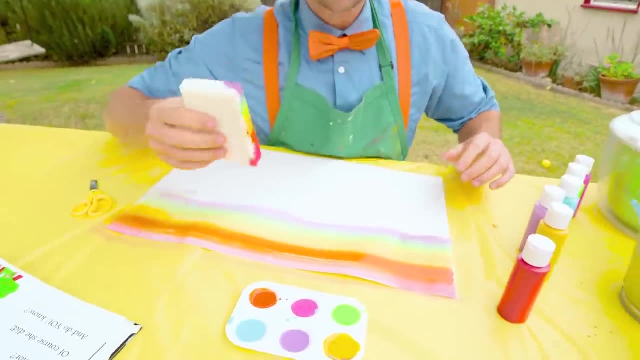 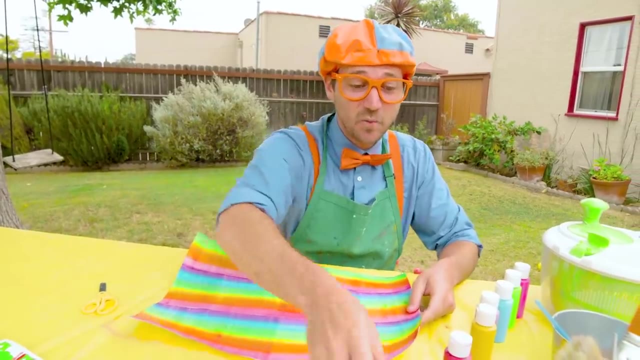 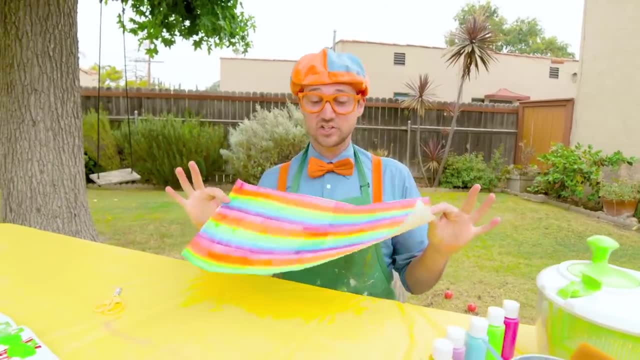 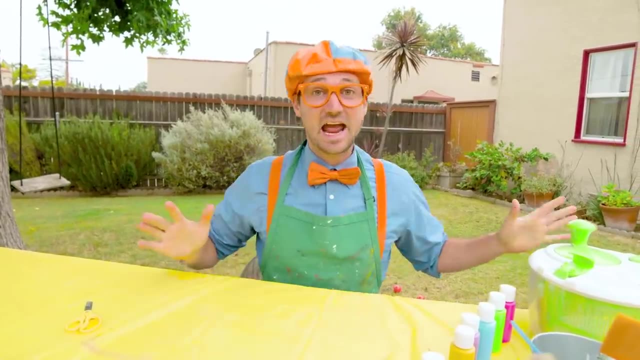 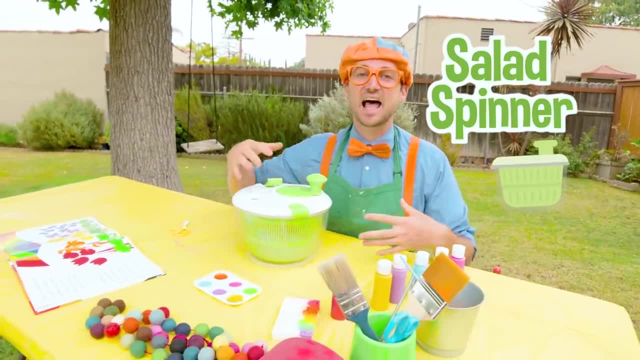 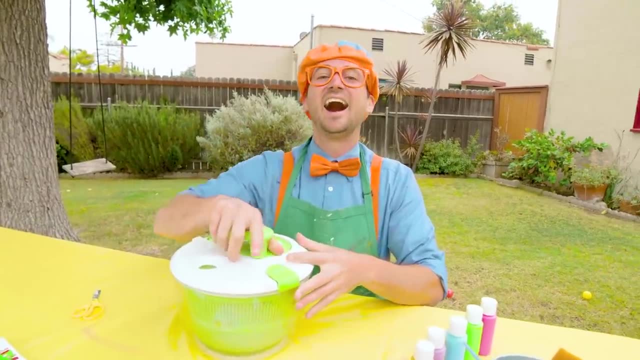 Perfect, Okay, Now what we need to do is take this salad spinner. You normally put salad kale, romaine lettuce inside here And you spin it around And it flings all the water off of it. And now? 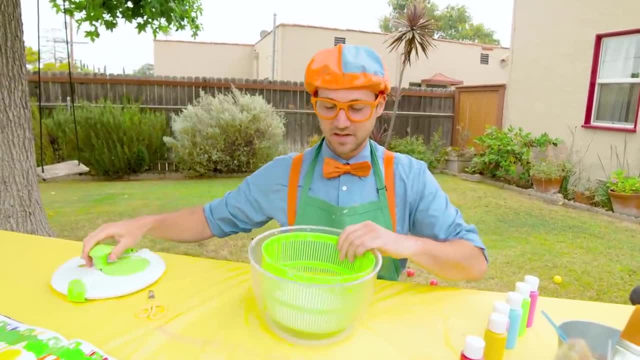 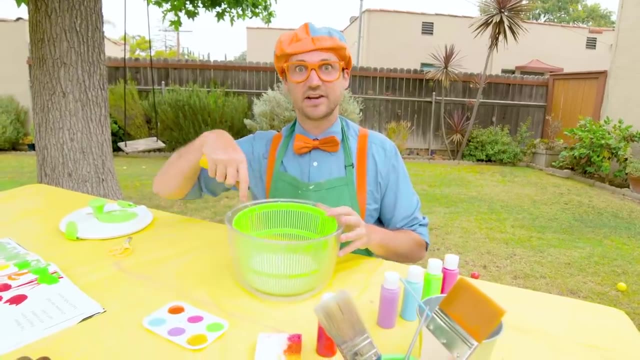 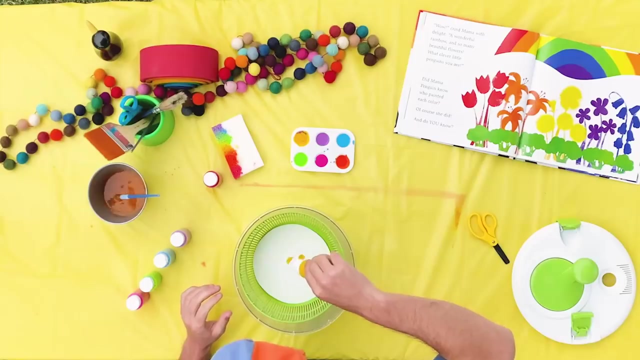 the water off of it. but today what we're gonna do is we have a white piece of paper right there and we get to put some colors in here and then spin it and then it pushes all the paint off to the edges. ready, we'll put some yellow. yeah, that. 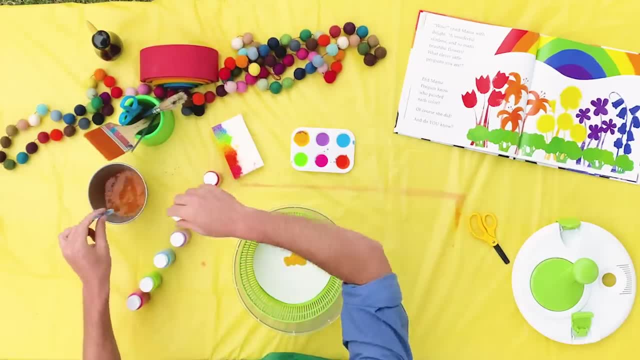 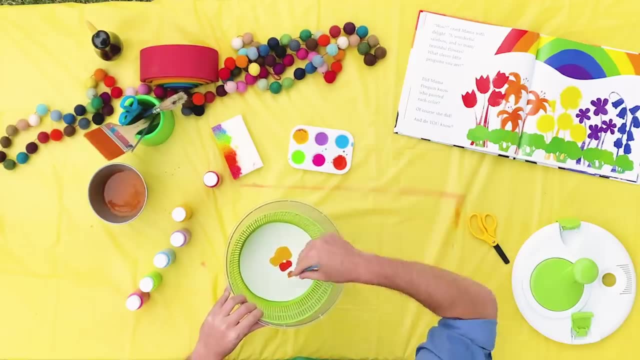 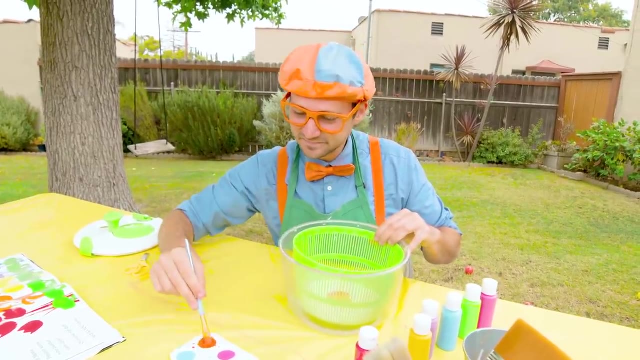 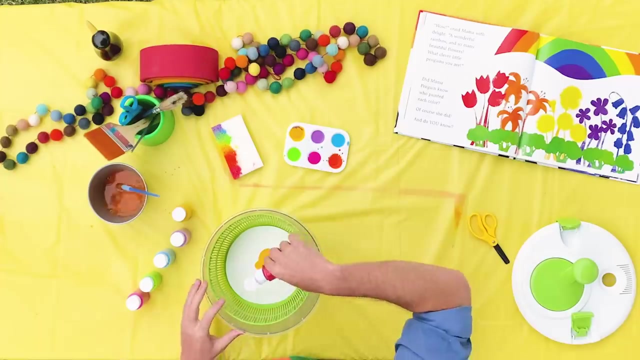 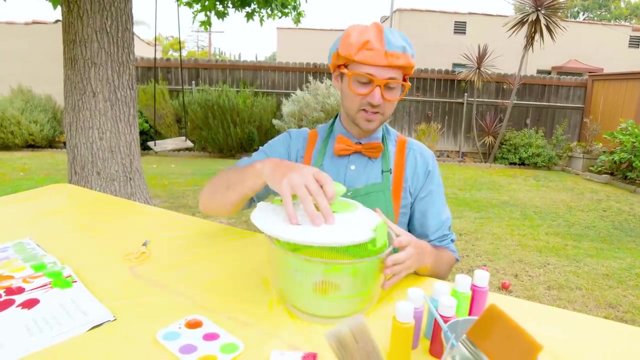 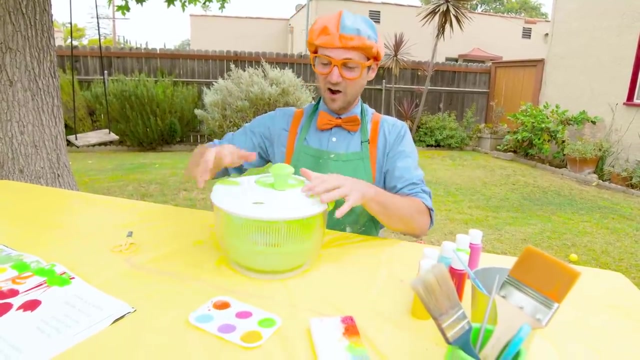 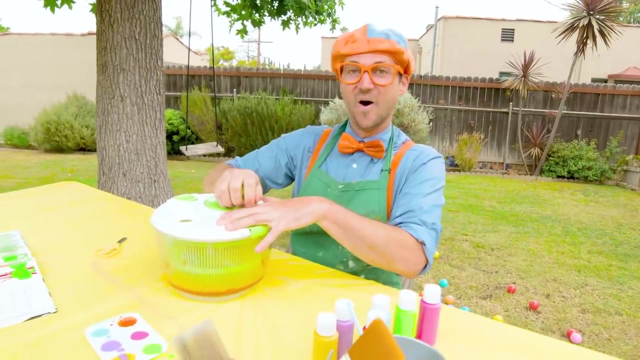 looks really good. and then, how about we put some orange? I love orange, yeah, just like that. Wow, yellow and orange. and how about a few drops of red? yeah, how about that? just a couple, there we go. perfect, all right, now let's put the top on. it's all sealed, here we go. that was awesome. I. 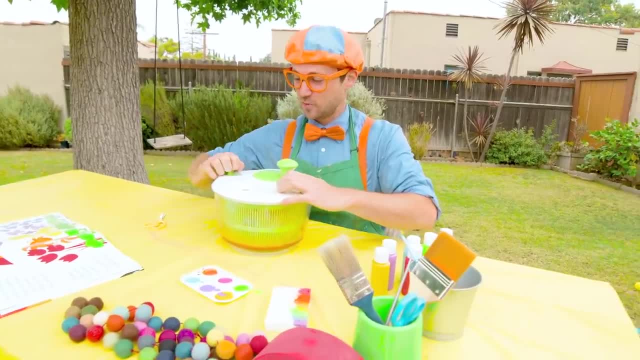 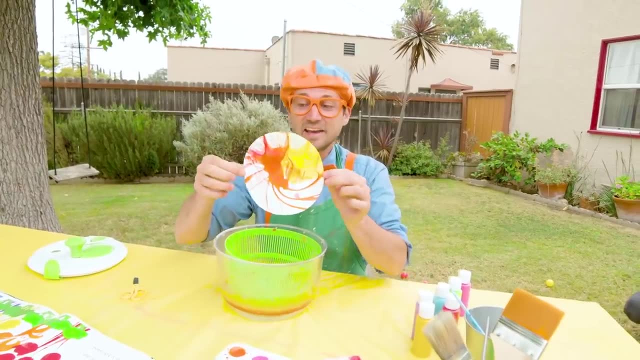 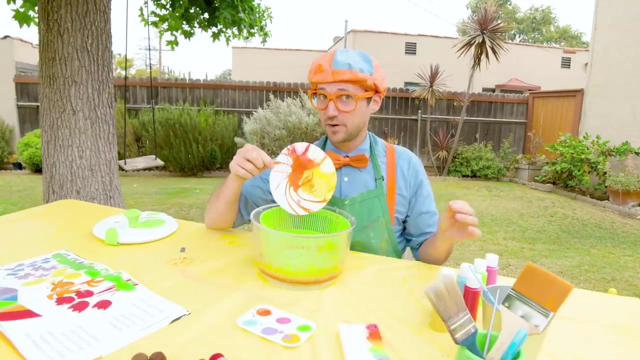 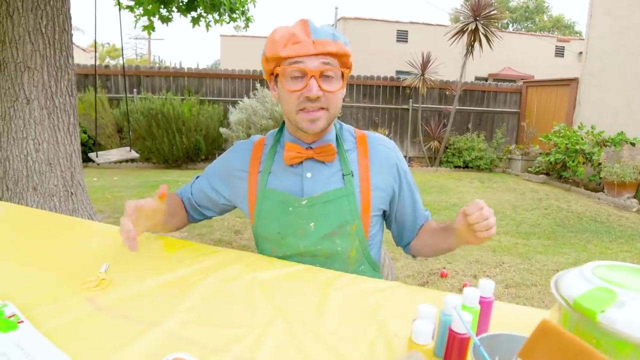 just spun it so fast. let's open it up and see what we have inside. wow, that is amazing. we just made that by spinning this around really quick. okay, it's pretty wet, so let me put it off to the side, so then it can dry. okay now. 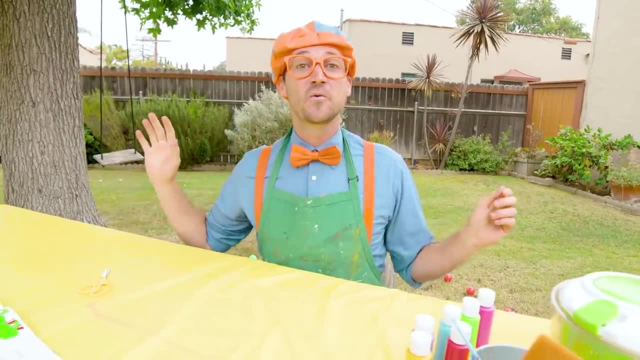 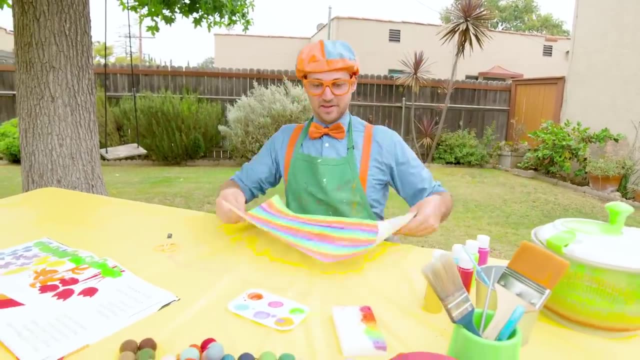 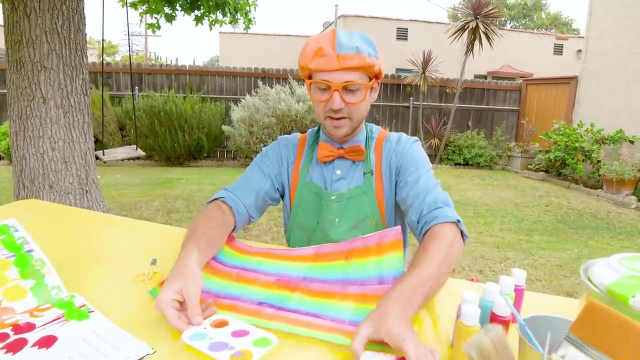 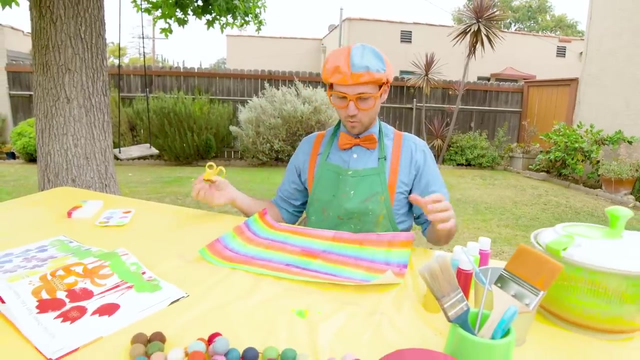 that I put that off to the side to dry the original rainbow. it's probably ready to use, so let me get it. yep, it's nice and dry, all right. so now what we need to do. let me organize this paint. I don't want it to get all over me now that we're all done painting. so what? 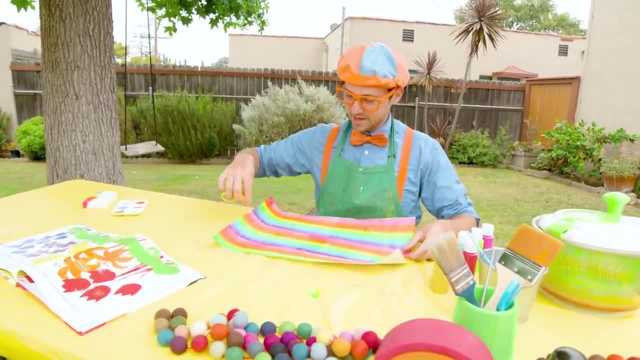 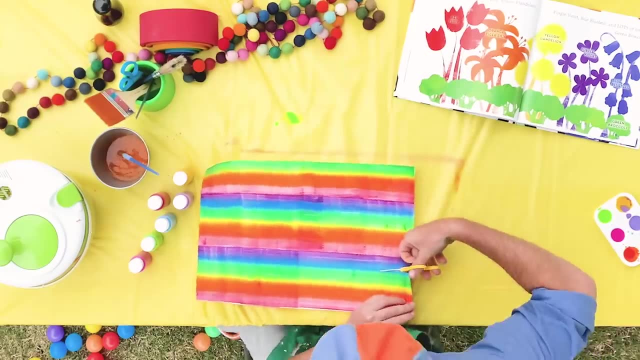 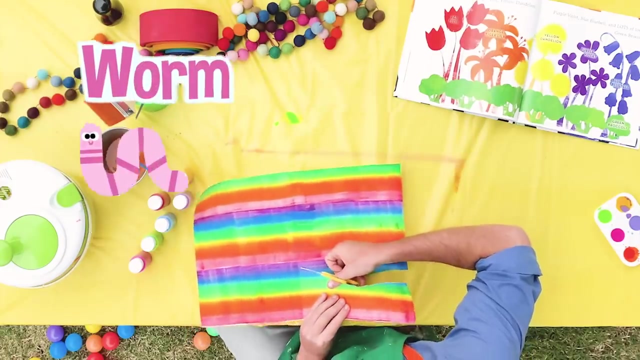 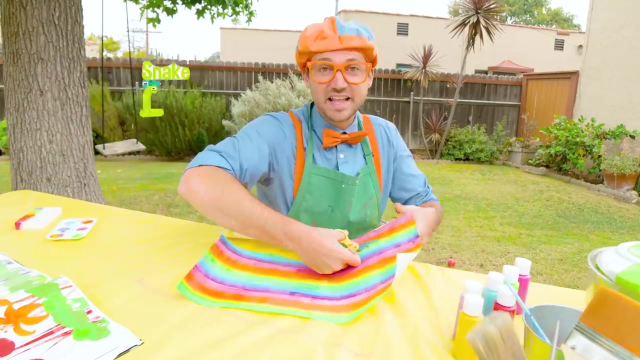 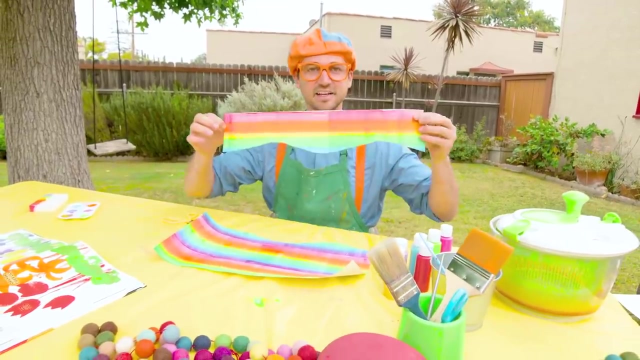 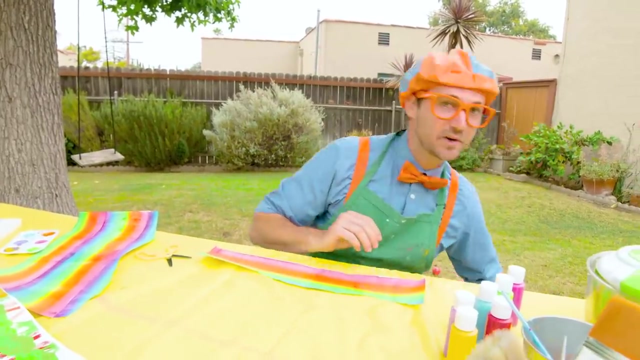 we're actually gonna do is take this and make a little squiggly line while we cut ready. yeah, just like this, oh, kind of like a worm, worm squiggle around or a caterpillar or a snake. see this, yeah, check that out. okay, now what I need is a white piece of paper. I have one. 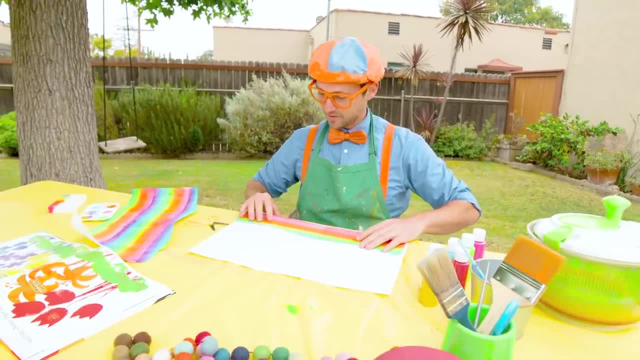 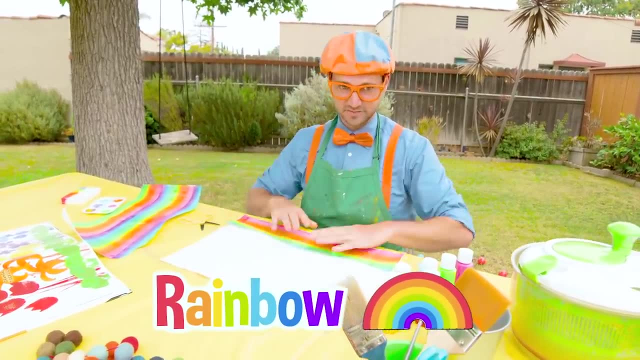 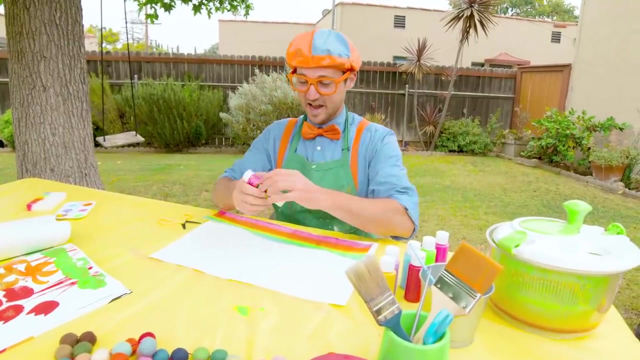 right on the ground over here and then I put it on the top. do you see that? yeah, it's like a rainbow, just like in Sarah's picture. so let me get some glue right over here, all right, now that I have this glue, I can glue it down. have you ever used a? 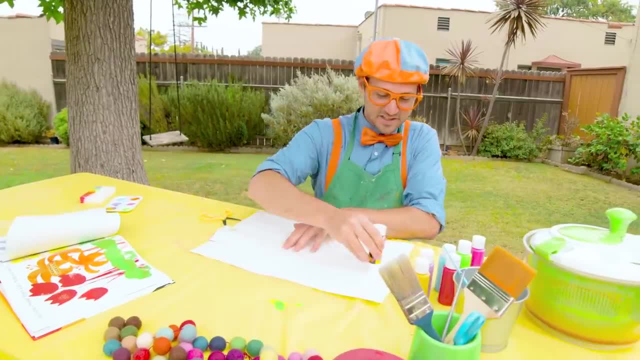 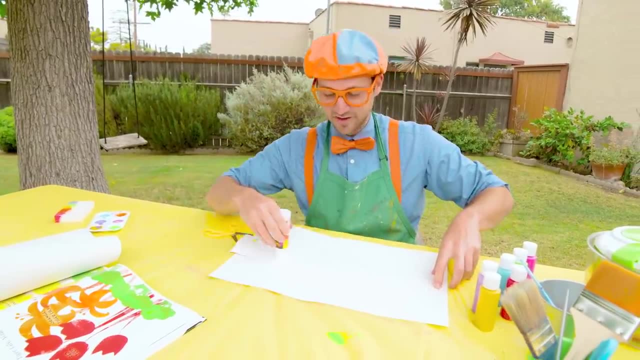 glue stick before. hmm, it's kind of fun. yeah, it's not all liquidy like the normal type of glue. this is a glue stick. you just kind of like color it on what. it's no color, sir, member어를. Yeah, there's no color to it, It's clear, Perfect. 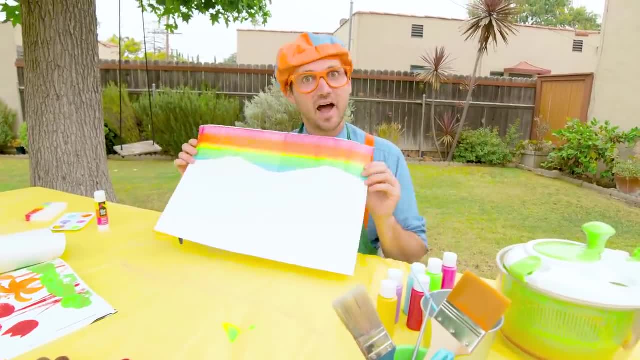 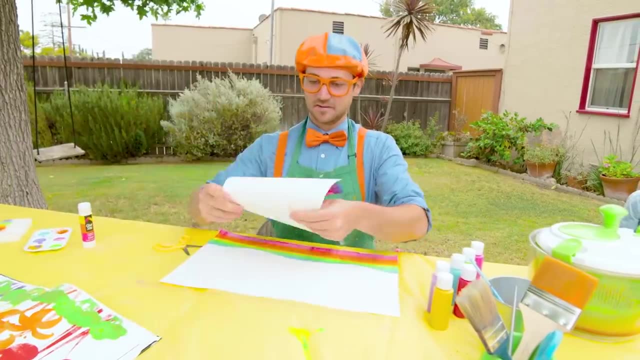 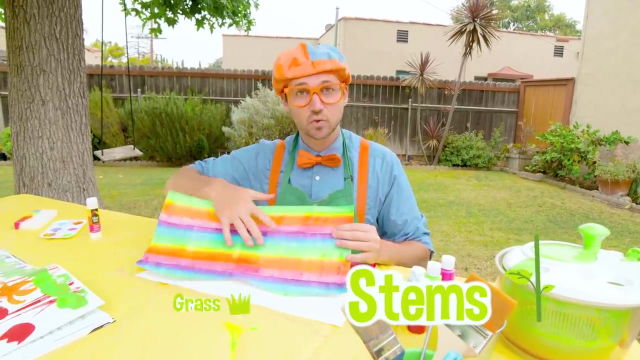 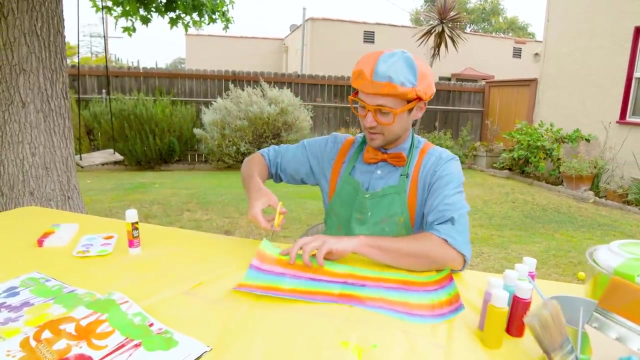 Wow, this looks amazing. You and I are doing a really good job. Alright, next step is to take this: remember The rainbow- And cut out some stems and grass from the other side. I'm going to set this down right over here, so then I can start cutting. 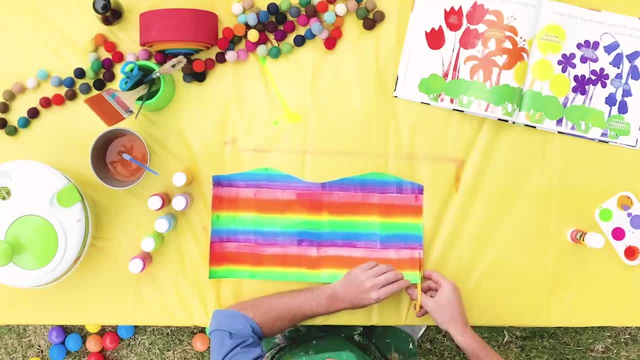 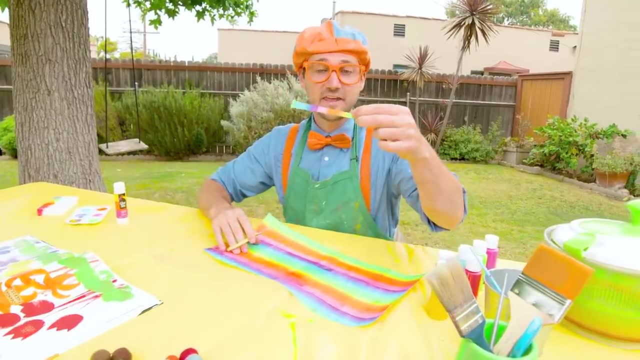 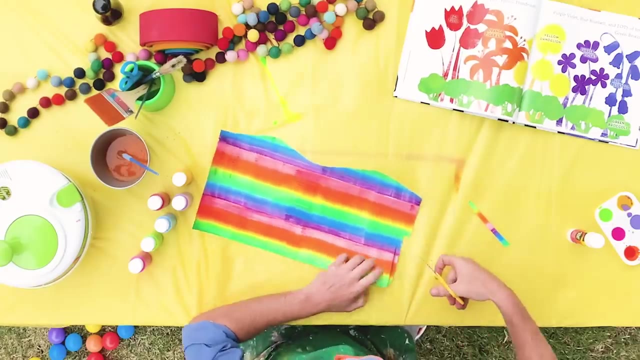 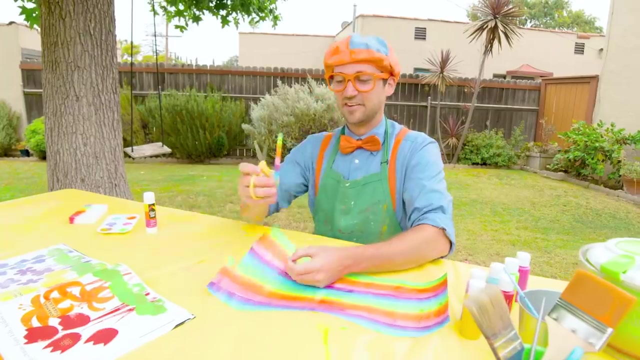 Okay, let's cut a nice long stem. Yeah, just like that. It's like a really thin, long rectangle, Perfect, Let me do another one. Yeah, I'll start with two. How about that? Yeah, oh, whoa, There we go. 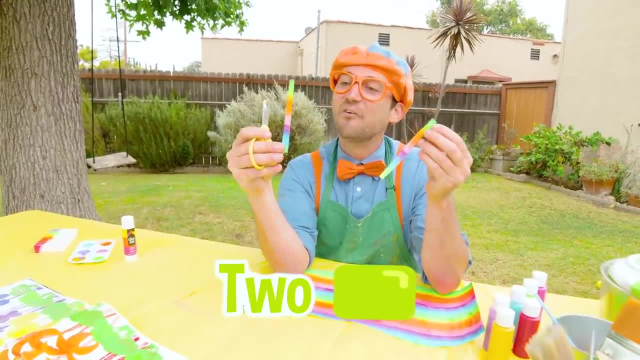 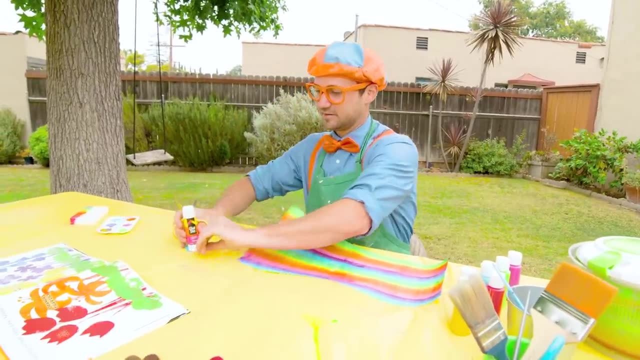 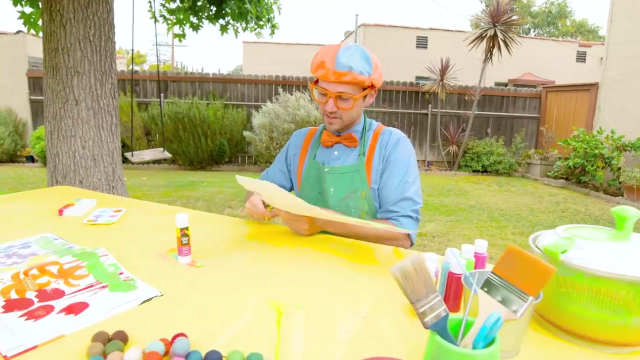 We have two long rectangles- Yeah, one, two- And these are going to be the flower stems. Okay, put them right under there. Perfect. Now we need some blades of grass, So what we're going to do is some triangles. 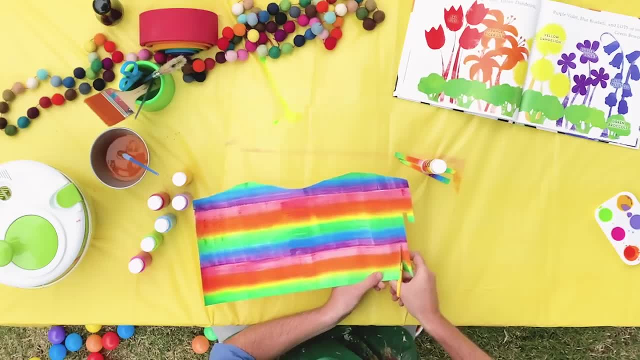 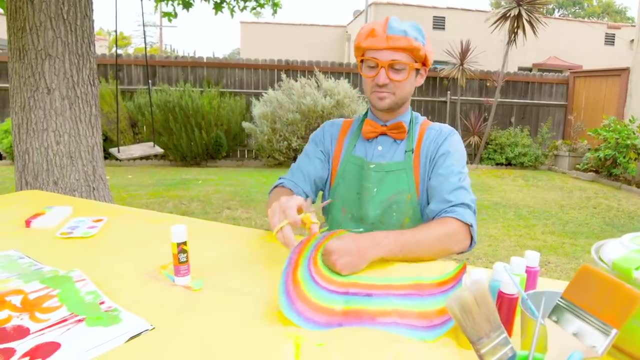 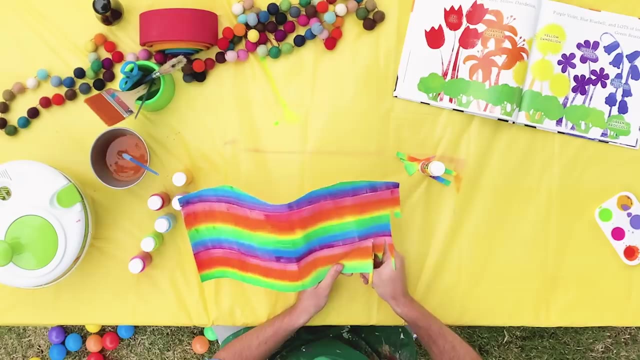 Just like that, Some nice tall blades of grass, As if you might need to mow your lawn. Yeah, and these blades of grass I'm cutting are triangles, just like I said. Whoa, How does that look? Do you like that blade of grass? 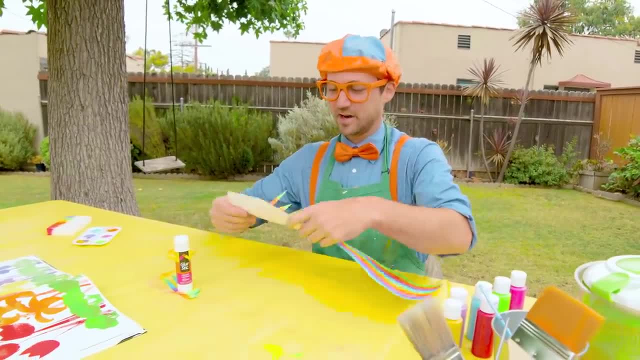 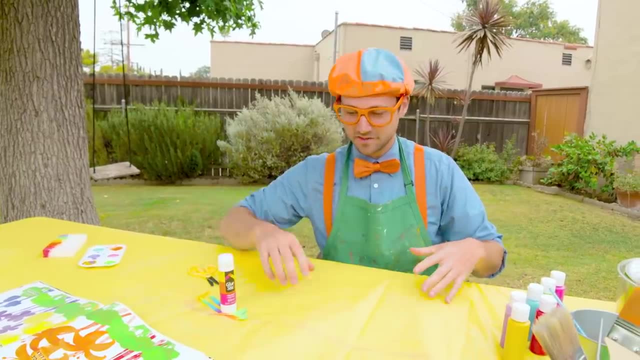 I sure do. All right, let's put those right here. I'm going to set this aside and grab my piece of art that had the rainbow on the top, And then here we go, I'm going to be able to put these on the bottom. 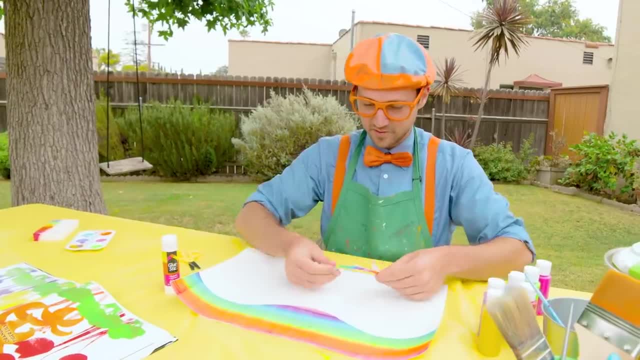 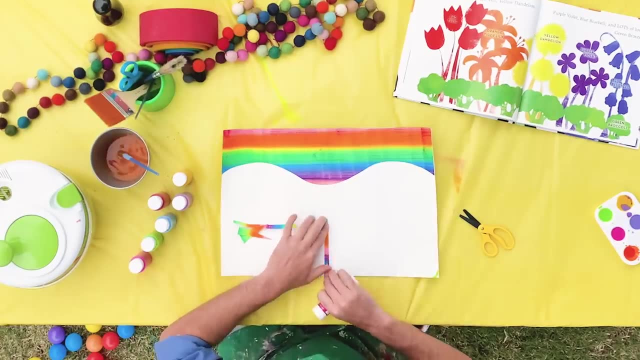 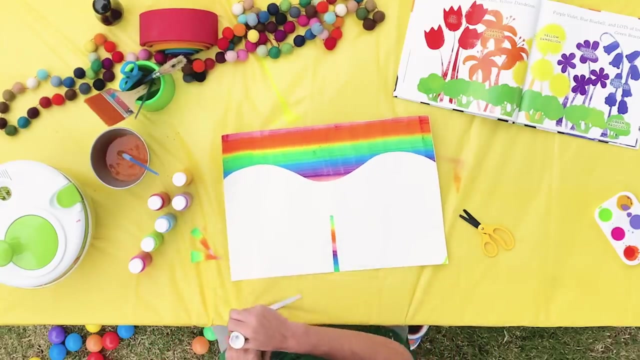 And I'll actually cut some more. But let me flip this around And take my glue stick again. Whoa, One right in the center. How about one to the side a little bit? huh Yeah, there we go. I love doing art. 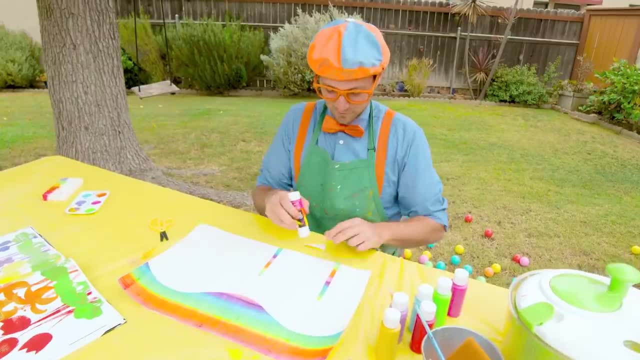 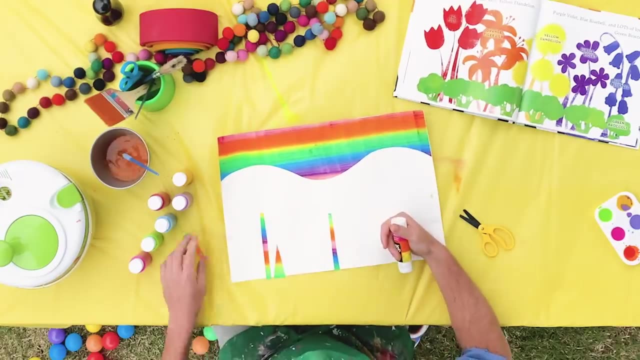 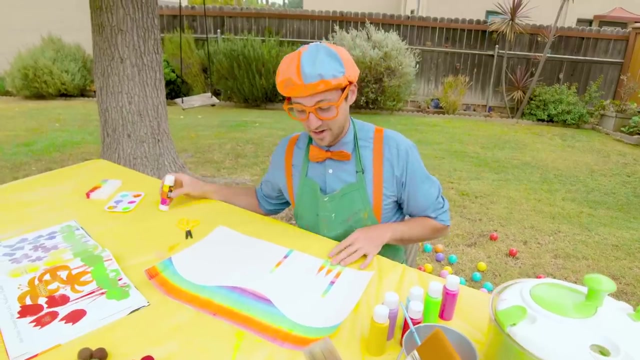 Yeah, how does that look? Yeah, and we'll do the blades of grass too. It's so colorful. Wow, Here we go, All right, Okay, All right. Looks like I need to cut some more and then glue it all down. 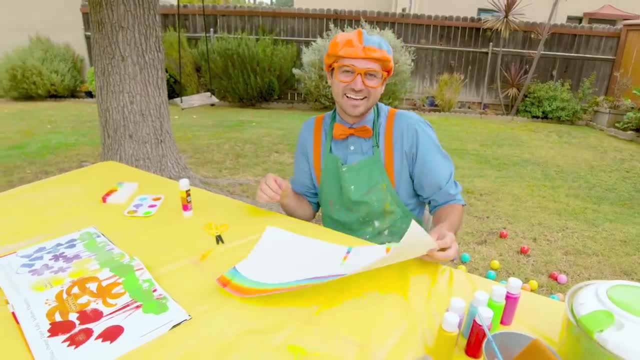 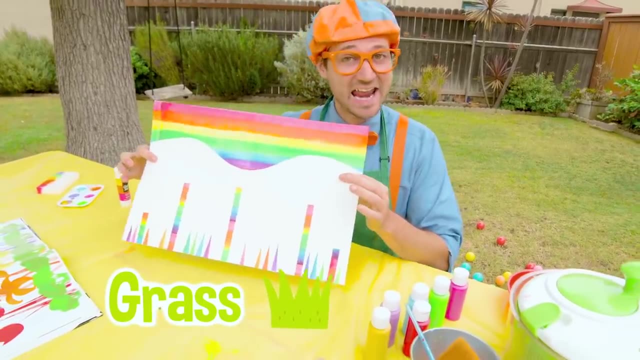 So let me grab the piece of paper and I'll cut a bunch. all right, Whoa, Check it out. All right, I did all the blades of grass and all of the flower stems. Now we need to do the tops of the flowers. 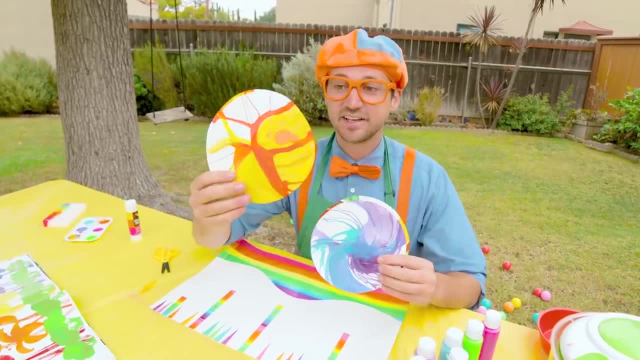 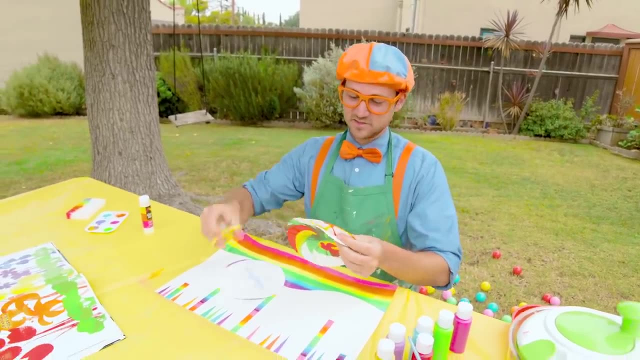 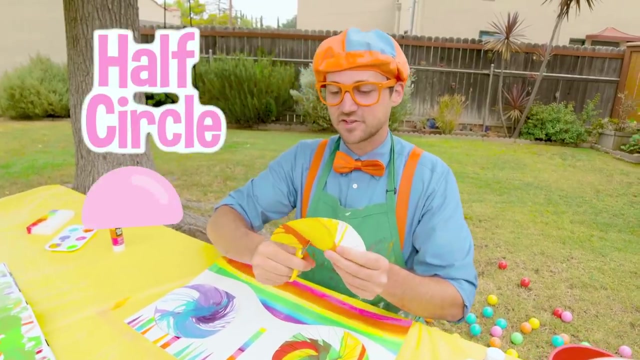 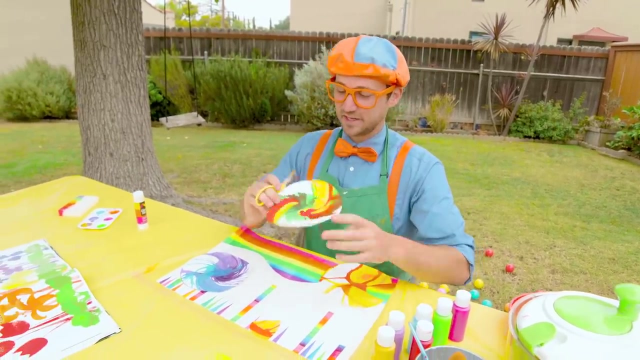 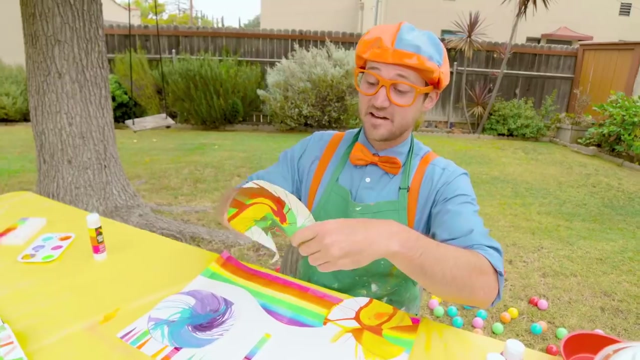 So remember, earlier we did the salad spinners. yeah, look at all these other ones that I have, okay, so let's cut them up so then we can use them for the flower petals. let's do a half circle, yeah, and then we can also do, yeah, something really big, because this one is gonna be a very big. 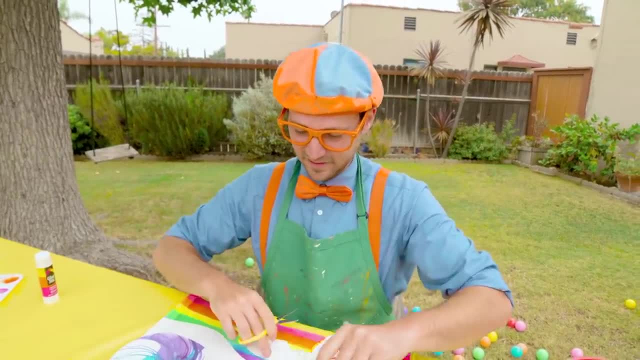 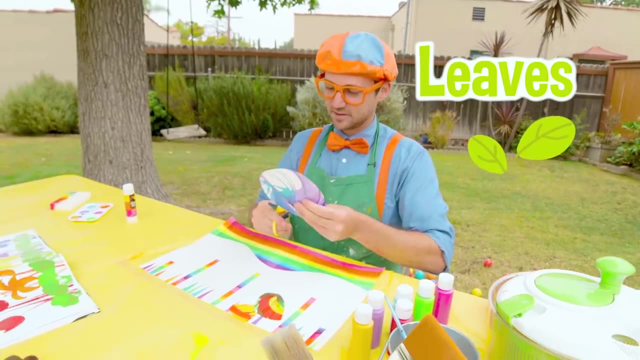 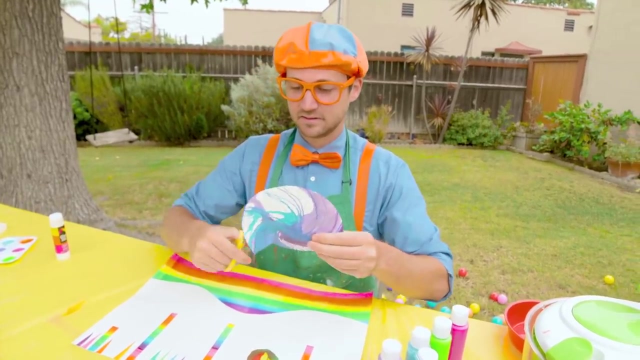 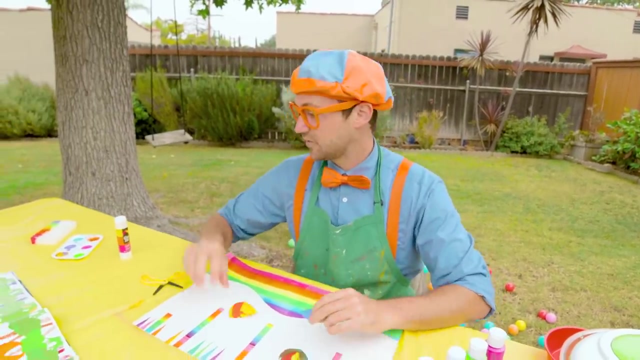 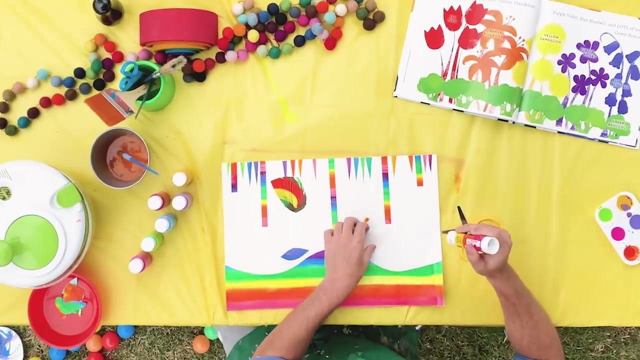 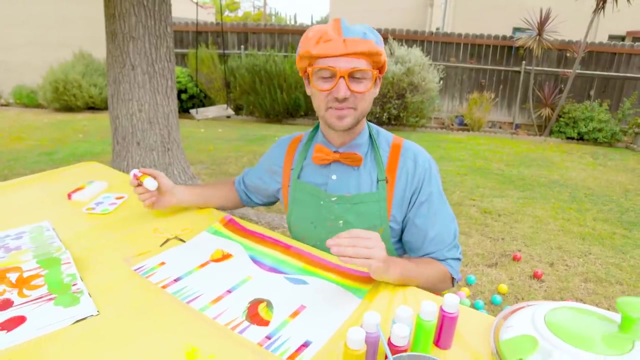 flower? yeah, perfect, that look all right. and then we need some leaves on this one. so let's go like this. yeah, just like that. then we can start gluing them down and making our flowers. so let's go like this: what is this look? yeah, that's a beautiful flower. I love the smell of. 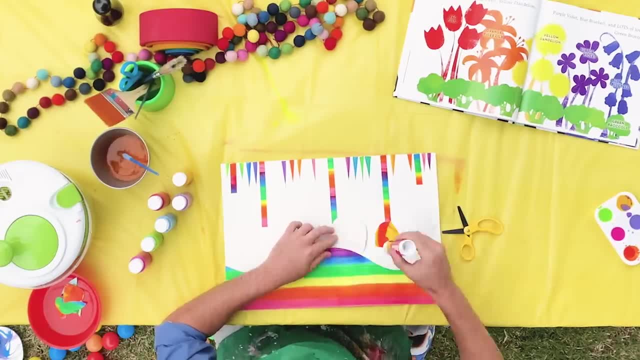 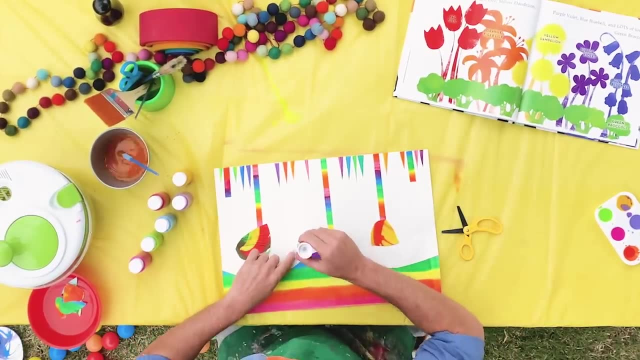 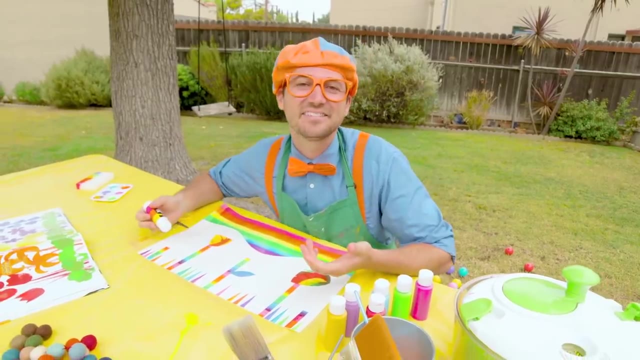 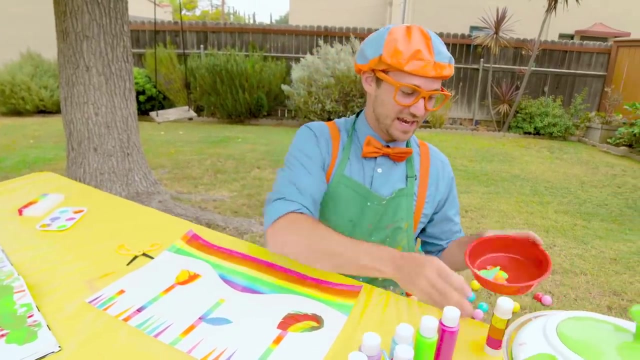 flowers, then this one will be another flower, yeah, and the stem. okay, let's do this. actually, you're not a stem, a leaf. we already have the stems right there. it's a leaf right there, right in the center of the flower leaf center. okay, I'm gonna cut some more and continue to glue them down. here I go. 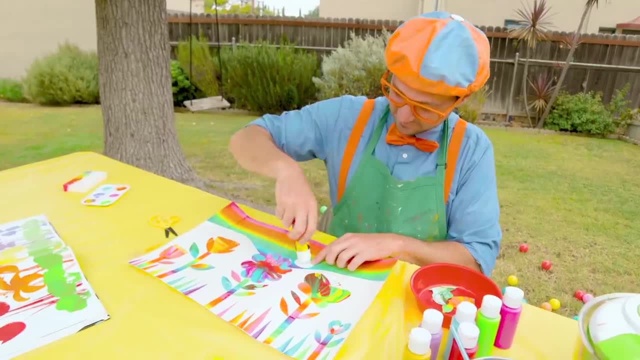 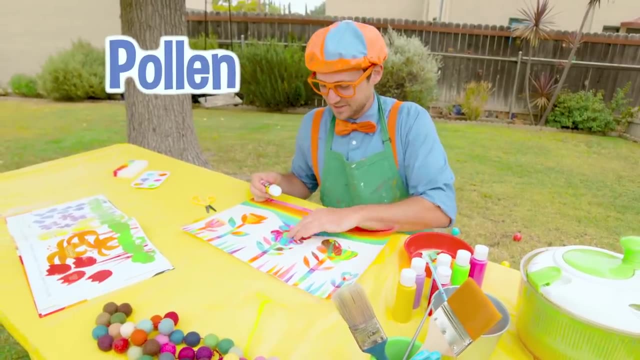 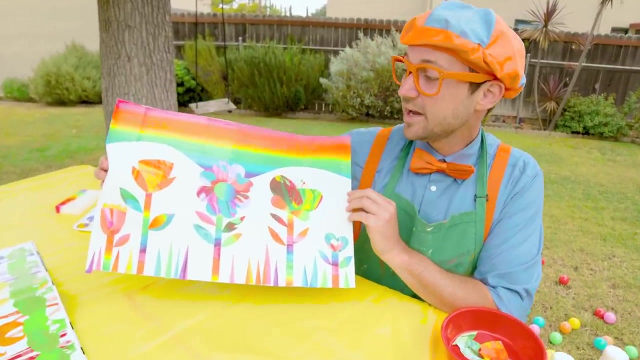 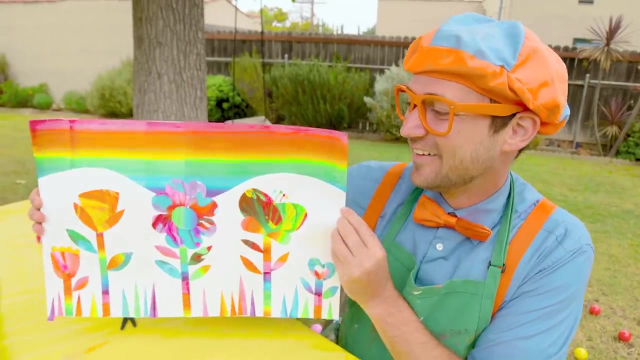 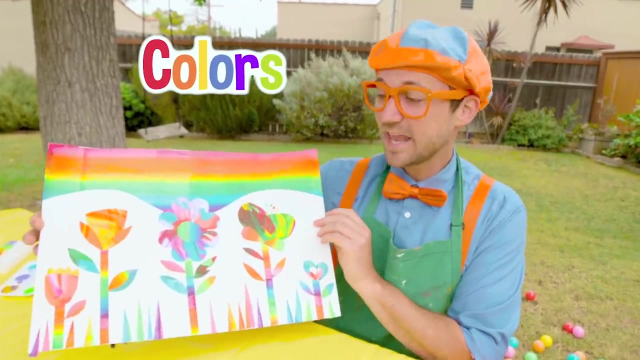 all right. last but not least, let's put the center of the flower. yeah, that's like where all the pollen is all right. how does that look? Wow, we made our very own rainbow garden. Wow, what a beautiful picture. well, thank you so much for learning about all the colors of the rainbow today with me, and about flowers. 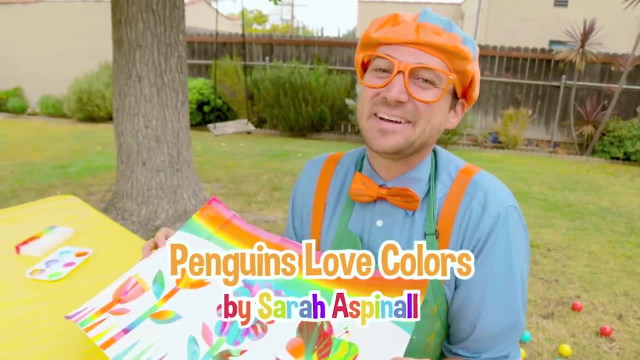 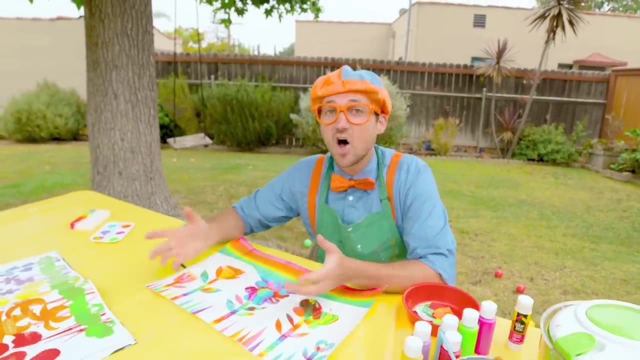 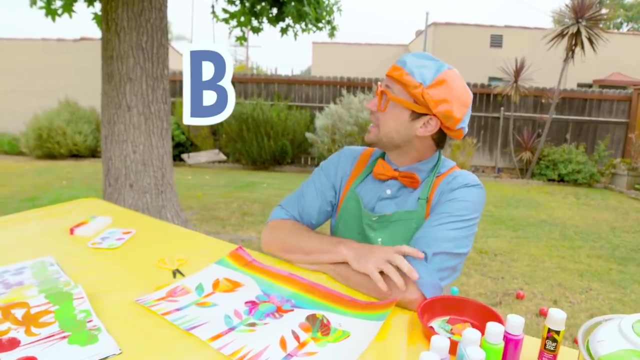 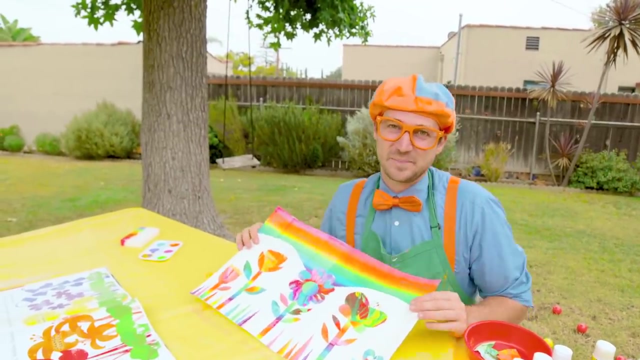 and also that amazing book about penguins by Sarah. well, this is the end of this video, but if you want to watch more of my videos, all you have to do is search for my name. will you spell my name with me? you ready? B-L-I-P-P-I Blippi, good job. all right, I'm gonna go frame this and put. 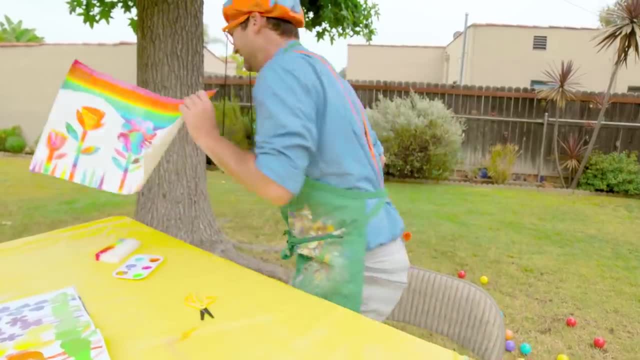 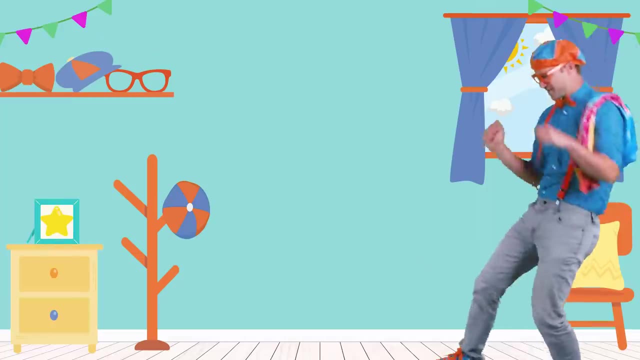 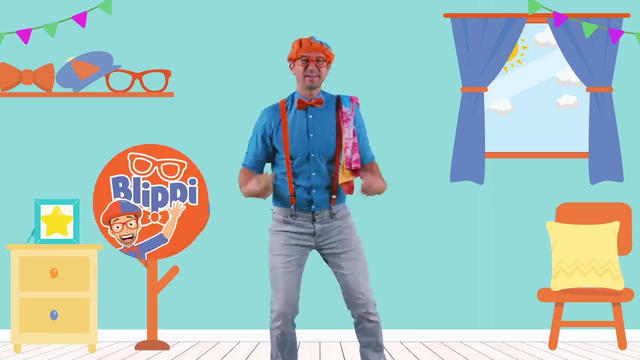 this in my treehouse. all right, see you later. so much to learn about. it'll make you wanna shout: Blippi, yeah, nice music. hey, it's me, Blippi, and I was just grooving to some tunes. Blippi, yeah, nice music. hey, it's me, Blippi, and I was just grooving to some tunes. 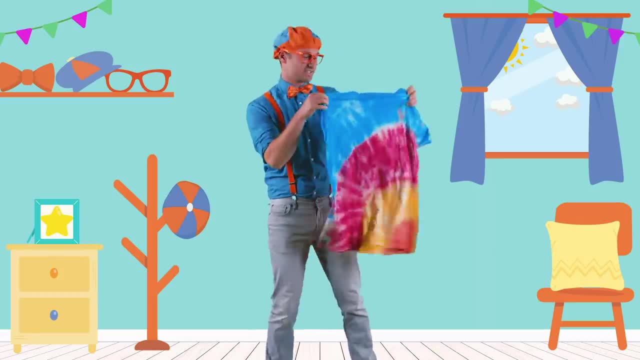 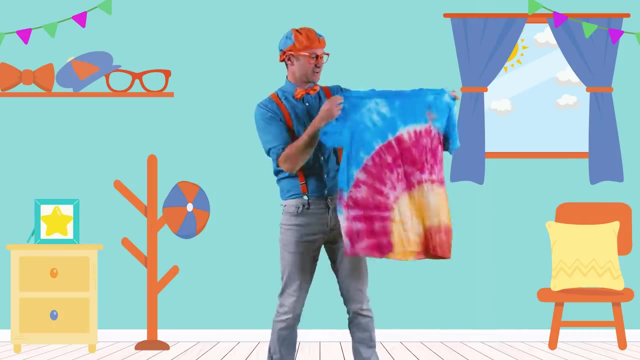 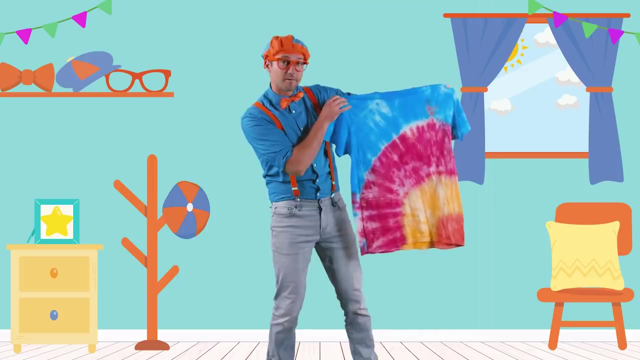 check this out, though. do you see this? this is a tie-dye shirt, and today you and I are gonna make a tie-dye shirt. Wow, it's so colorful. let's list all these colors. top, there is the color blue. yeah, then below that looks like it's the 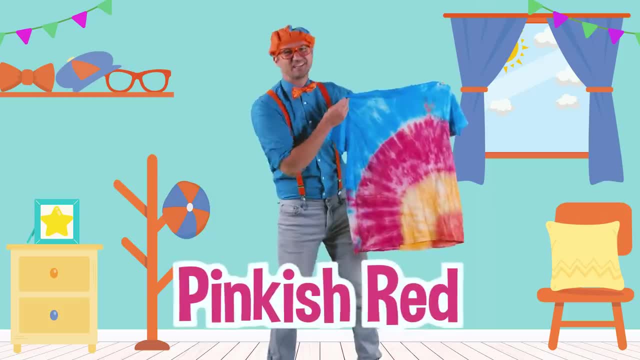 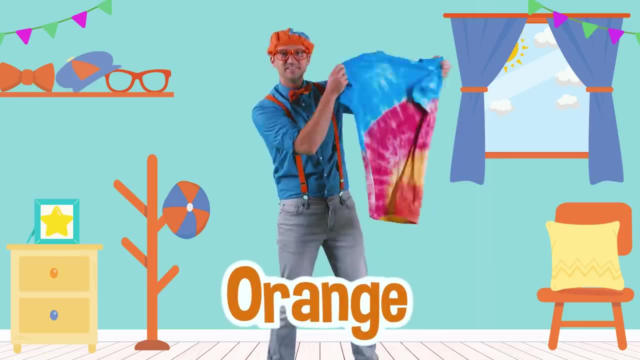 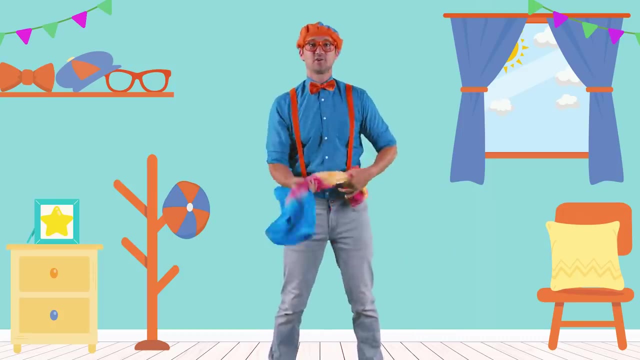 color, pink or red, pinkish red, and then we have yellow and blue, and then we have, like, the color of the Sun. then we have orange at the bottom. do you see it, whoa? this shirt is so groovy. all right, let's go get some supplies and make our very. 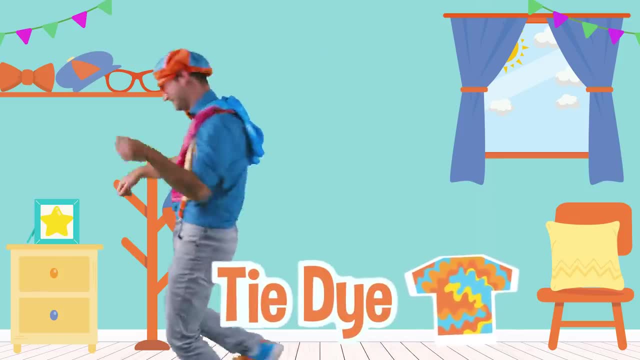 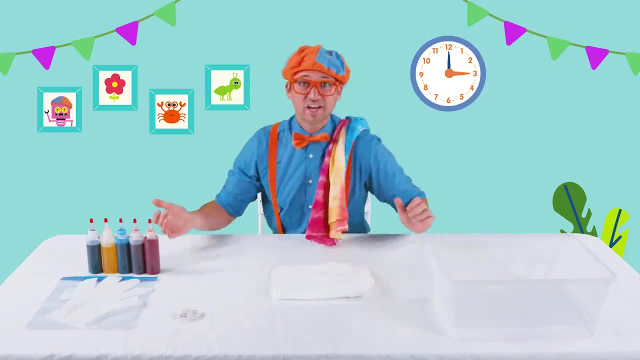 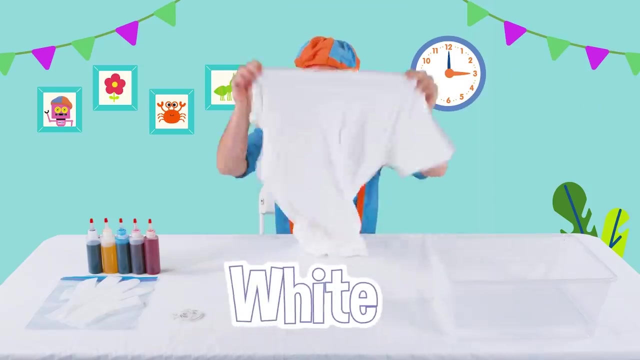 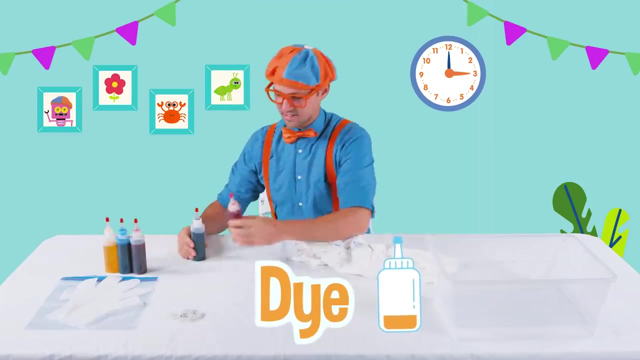 own tie-dye shirt. check it out. we have all the materials and supplies we need to make our tie-dye shirt. all right, we don't need this because we're gonna make one. so first you start with a white t-shirt- yeah, like this, see. and then you take a die- yeah, let's see a. 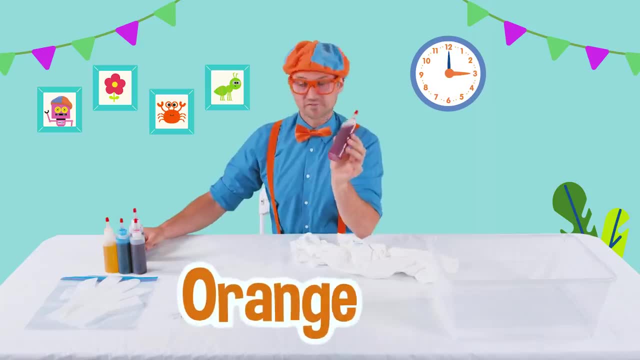 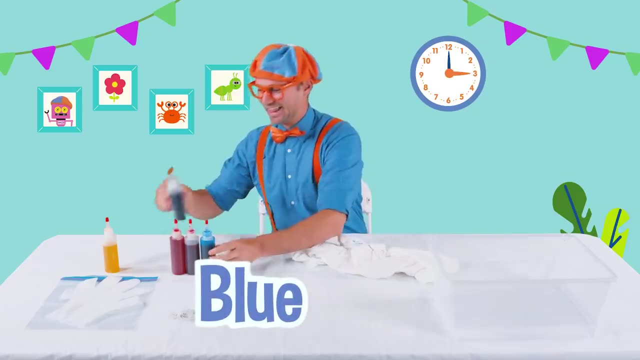 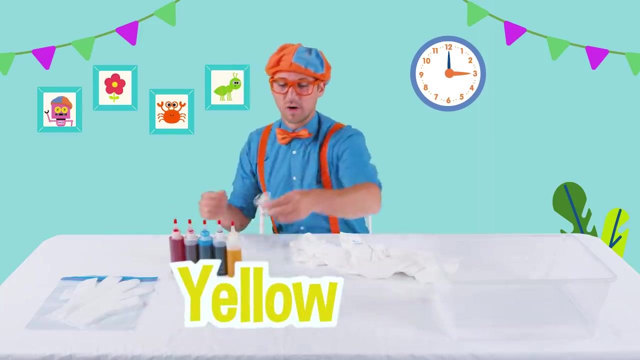 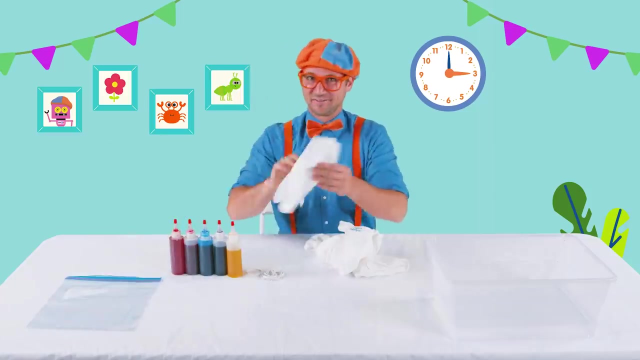 fabric die. this is the orange fabric die, this one is red, this one is blue, this one is purple, is yellow, and then we have some rubber bands and you tie the shirt really tight, then you spray the dye on it, but you have to wear your gloves or else your hands are gonna get stained. 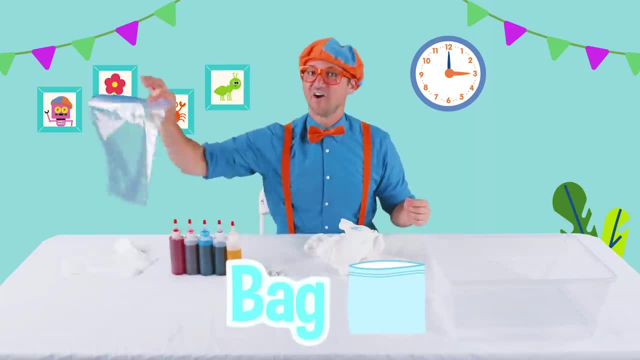 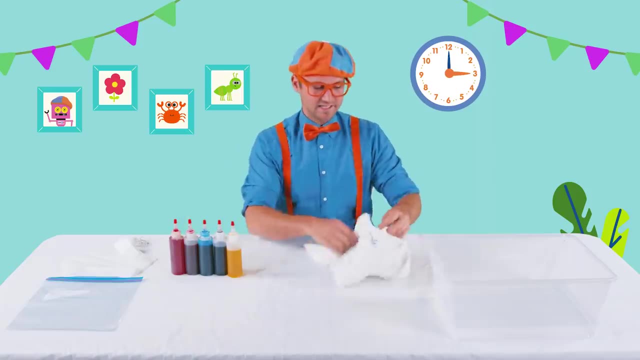 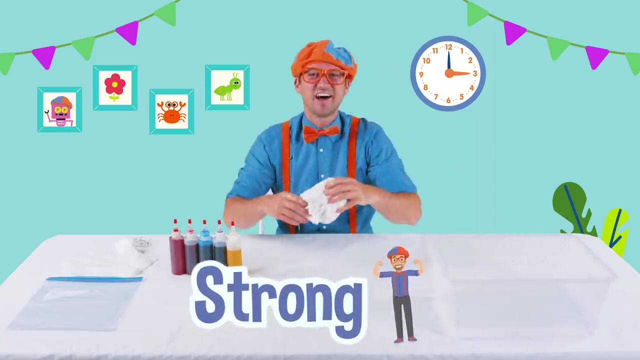 i don't want that. and then we have a bag for later. i'll show you what that's all about. and the water, okay. so first step, we need to get the shirt wet, just like that. let's get it nice and wet. wow, the water's really cold. okay, squeeze out all the water. whoa, we're so strong, all right. 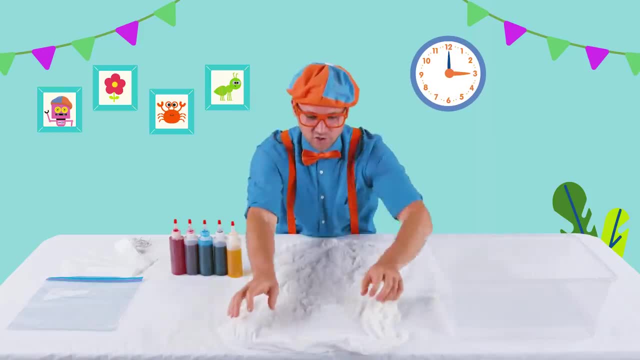 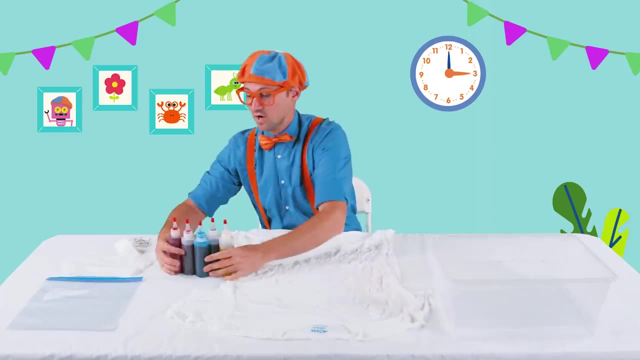 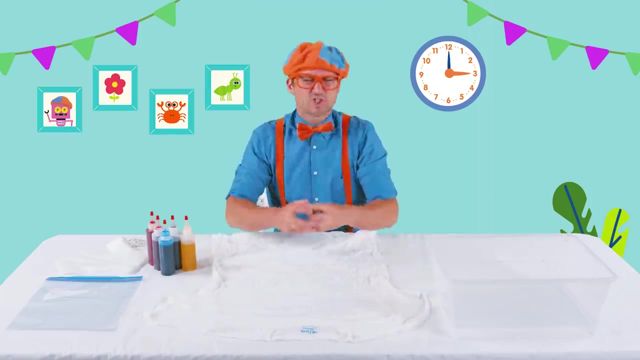 and then let's look at the other side and then we're gonna lay the t-shirt out on the table. yeah, and the cool thing about tie-dye is you can do so many different designs, and it's all about how you twist and crunch the shirt and wrap the rubber bands around it. so let's- uh, let's do. 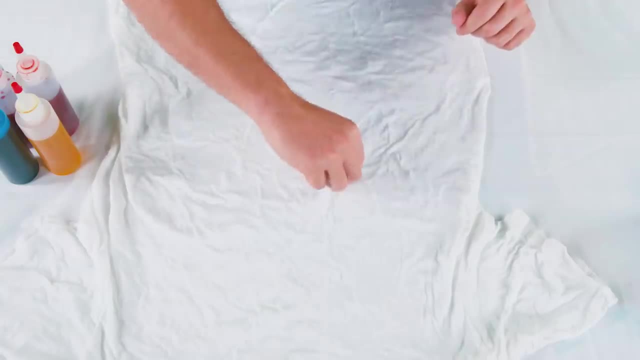 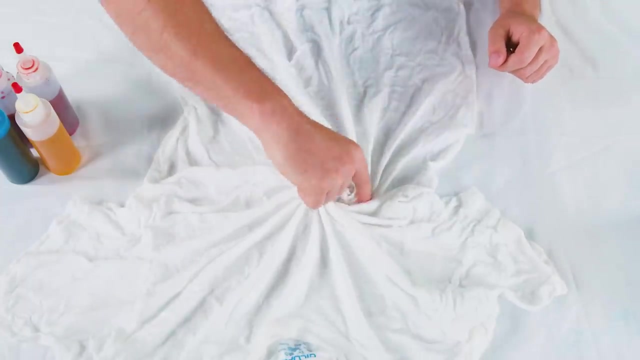 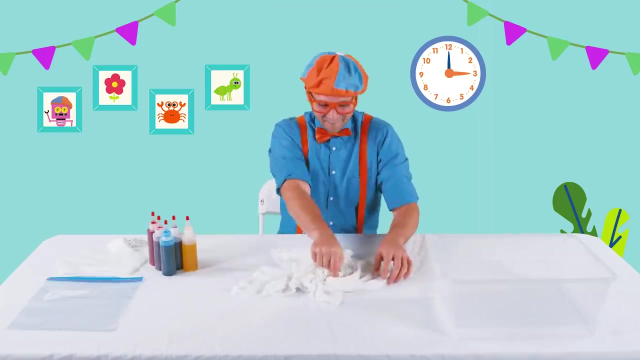 a swirl. i love swirls. yeah, kind of like ice cream swirls. i love ice cream. okay, here we go. so you just twist it, swirl it, perfect. wow, i'm so excited to pick the colors. okay, there we go. and then you have a nice bunched up shirt. you could even bunch it, but i chose to swirl it. then you take these rubber bands. 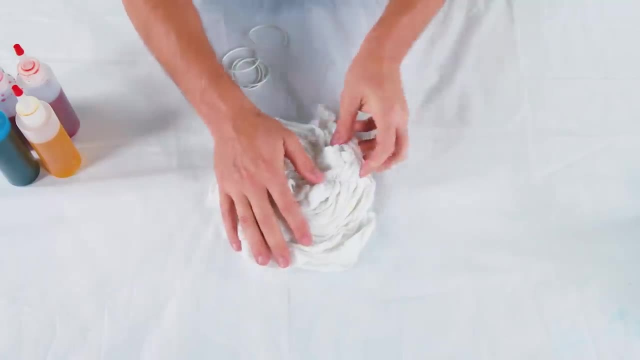 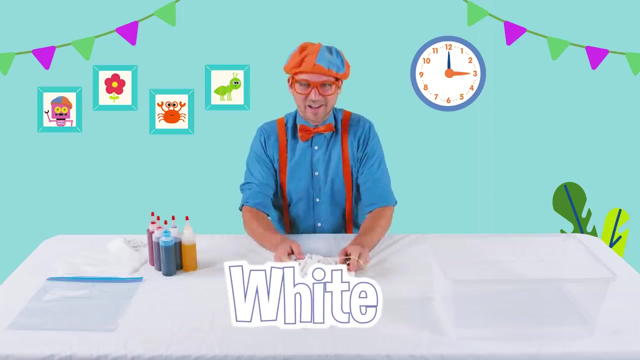 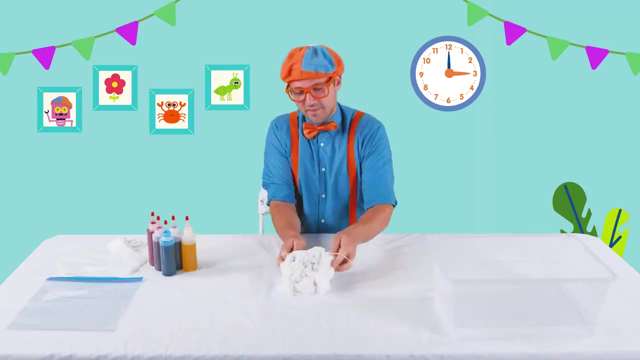 and wrap them around the top and the bottom of the shirt, just like this. yeah, this white shirt is gonna be so colorful. all right, there's two rubber bands. here is three rubber bands- perfect, this is looking so good. and then there's the fourth rubber band. wow, will you count to four with me? 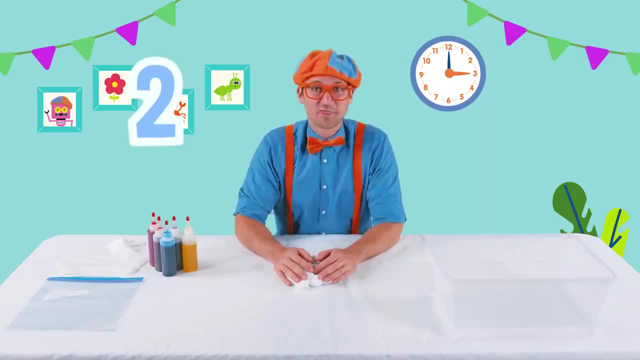 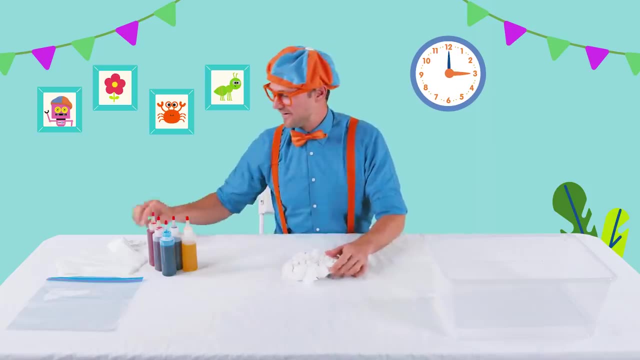 ready. one, two, three, four. good job, all right. now we get to pick our colors. but remember, let's put on our gloves. okay, here we go. one glove, two gloves, one, two. all right, let's see, we have a lot of colors. i know i think i'm gonna choose two colors. 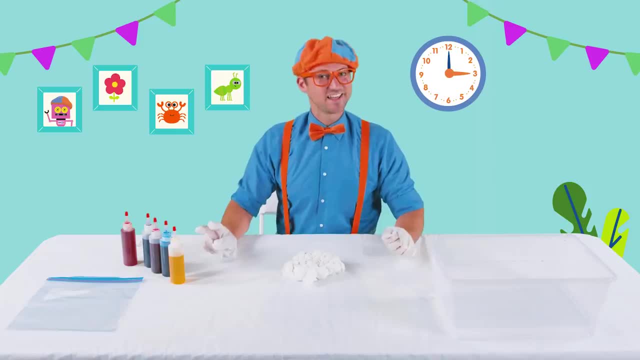 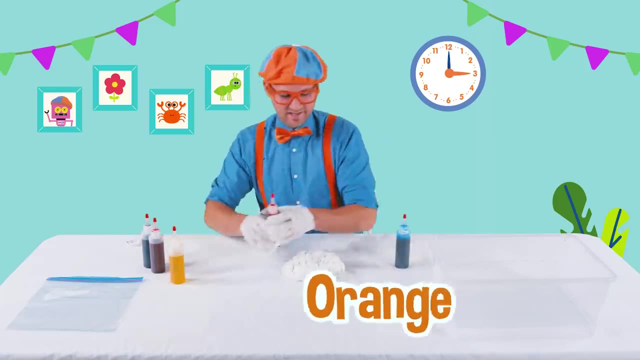 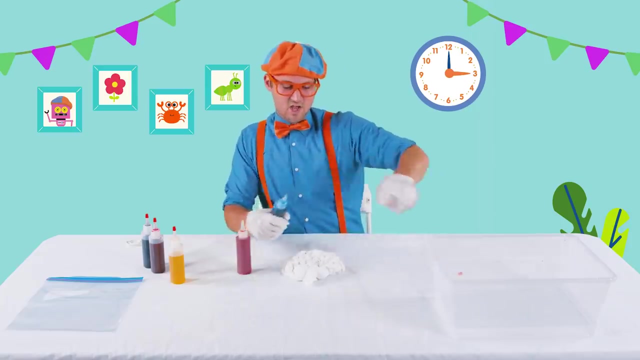 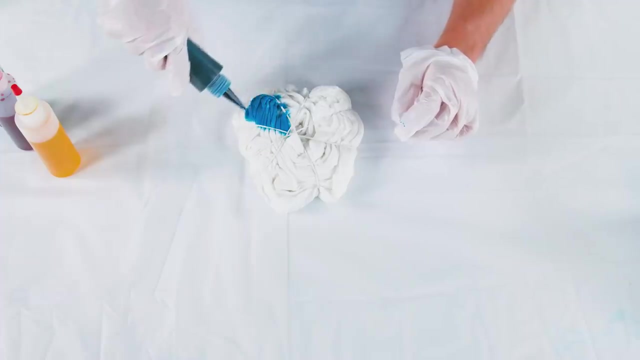 my two favorite colors. do you know what colors they are? yeah, i bet you do. yeah, blue and orange. all right, here's the two colors. and then take the caps off and then you get to squirt the shirt in whatever way you want. i'm gonna squirt some blue, right. 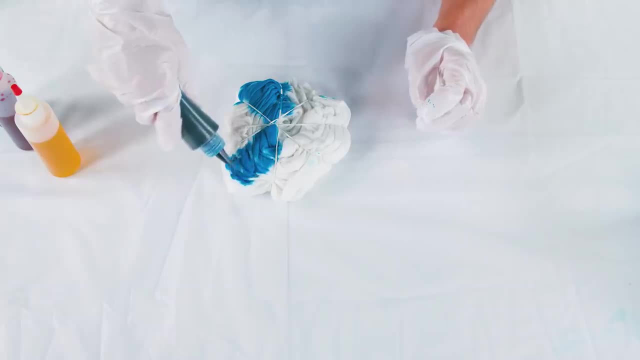 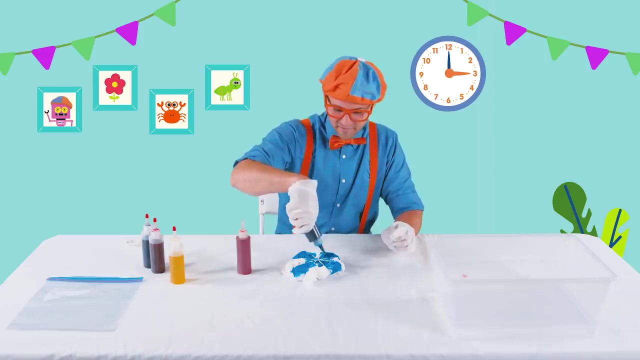 there. i'll skip some and squirt some blue right there. how about some blue right there? it's a blue right there. wow, the shirt was all white, but now what color is it? yeah, there's two colors: blue and white. yeah, all right, let's give it a little more. 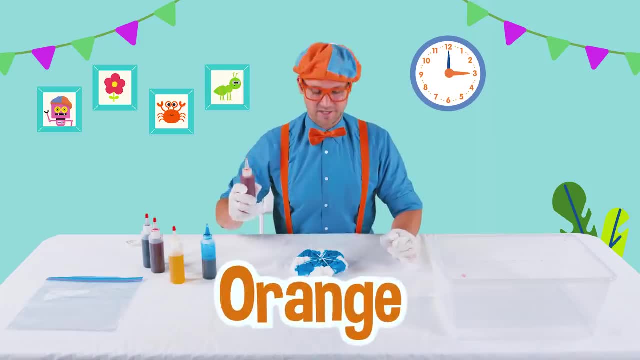 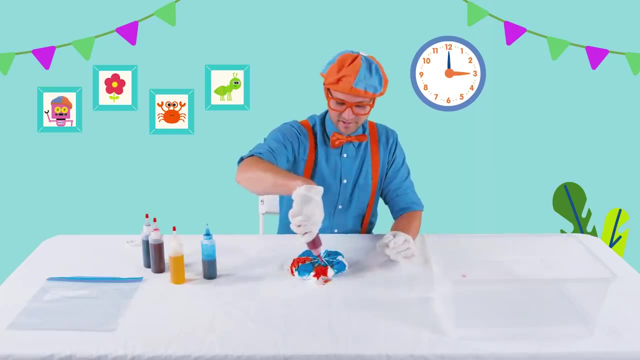 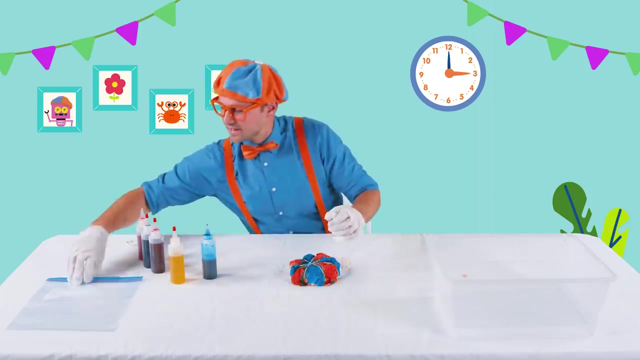 all right. so then the other color, like i said, is orange. so let's squirt that white and get it nice and orange. there we go. wow, we are doing so good. there we go. perfect, wow, amazing, wow. this looks so good, do you see it? we have blue and orange, all right, set that down. and now you take the big plastic bag. 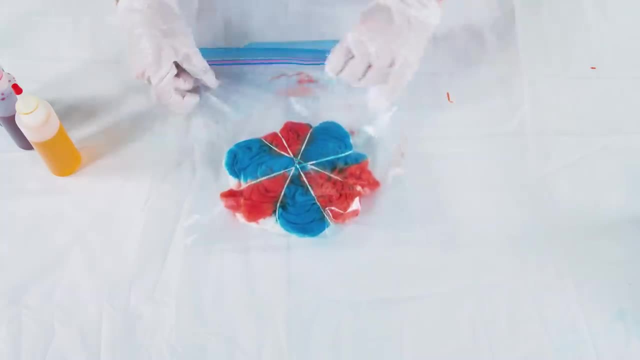 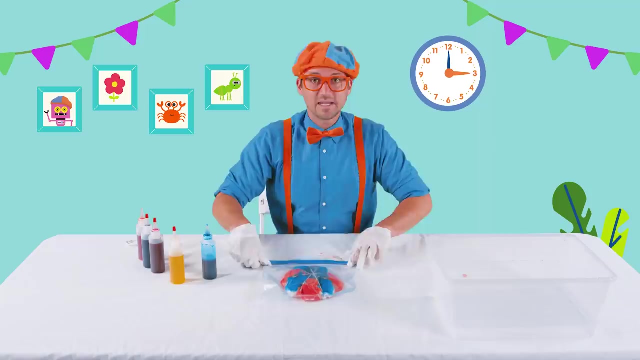 and put the shirt in there and close it up, and now we get a weight. but you have to keep it in here for at least six hours. you can even do it up to 24 hours if you wanted to. the longer you keep it in this bag, the darker and more vibrant the colors. 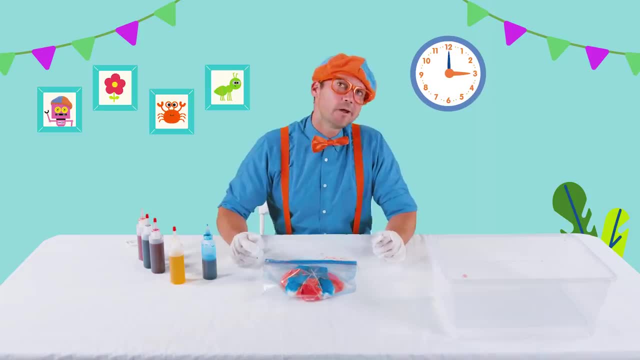 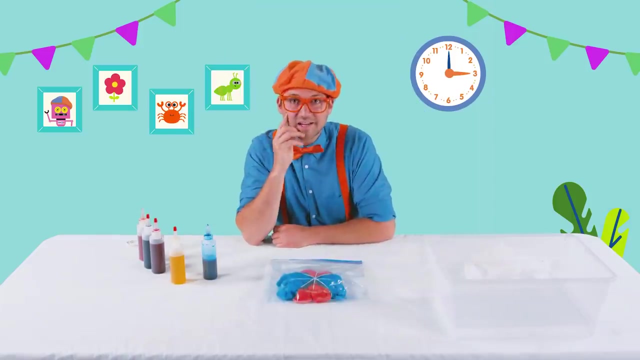 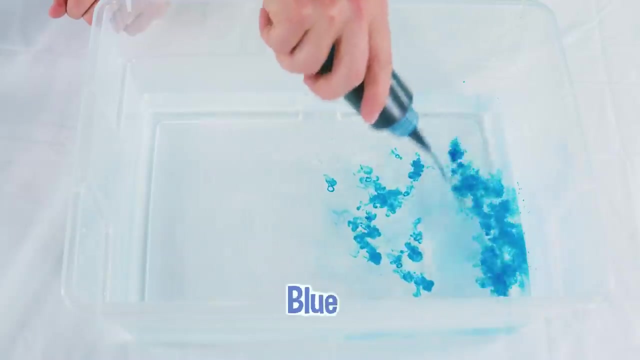 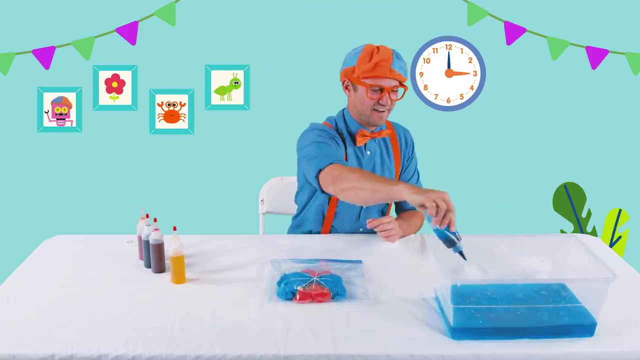 are gonna be. hmm, i think we should probably wait eight hours. so let's wait. hmm, we're almost done waiting, but i think what we should do is mix two colors and see what color it is makes. first, let's take our blue whoa. do you see that? whoa? that's awesome. wow, blue water then. 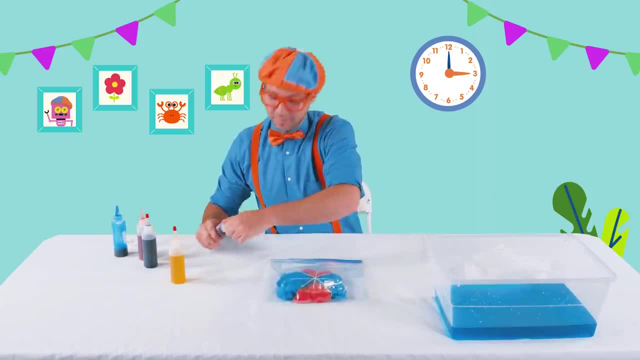 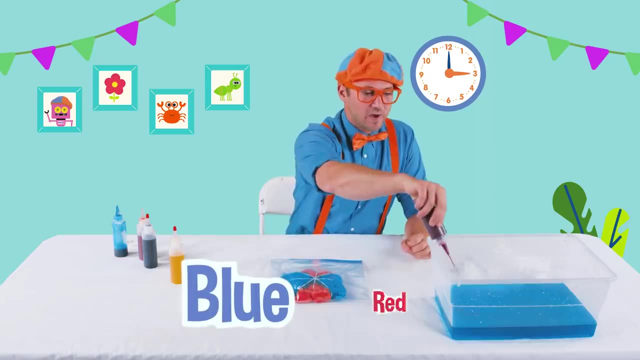 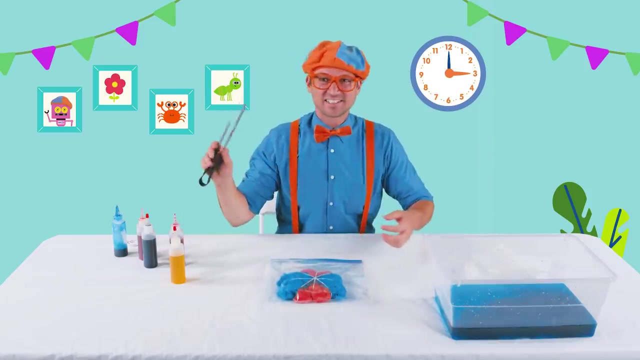 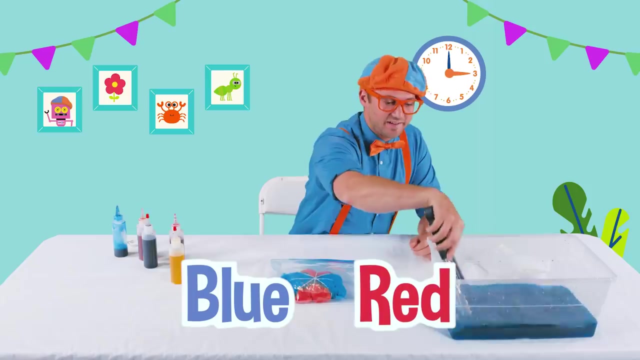 let's take how about red? hopefully it doesn't spill on me, because i don't have my gloves on anymore. all right, here we go. blue and red. whoa, what color is that? i have my mixing tongs? blue and red make the color purple. wow, let's put a little bit more red in there. 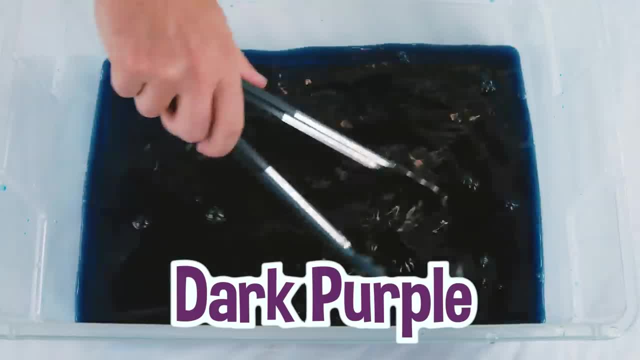 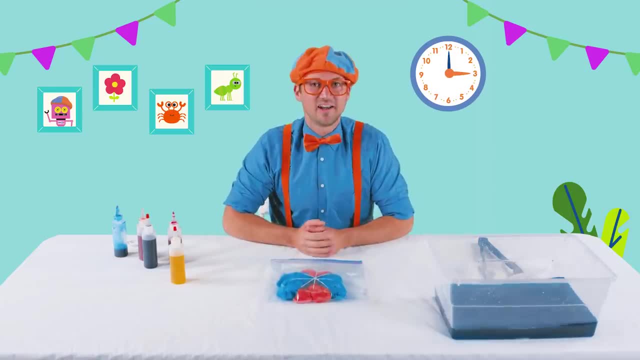 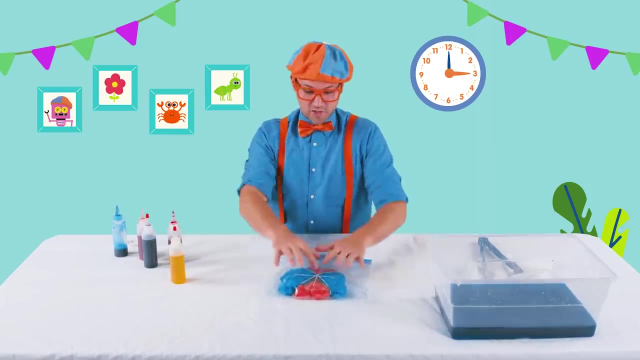 wow, now it's a dark purple. whoa, that's fun, okay. well, i think our t-shirt has been in here for long enough. it's been about, yeah, multiple hours. so now i'm gonna go take this t-shirt and put it in there- wow, the sink- take the rubber bands off and rinse it off, and then i'm gonna go put it in the dryer. 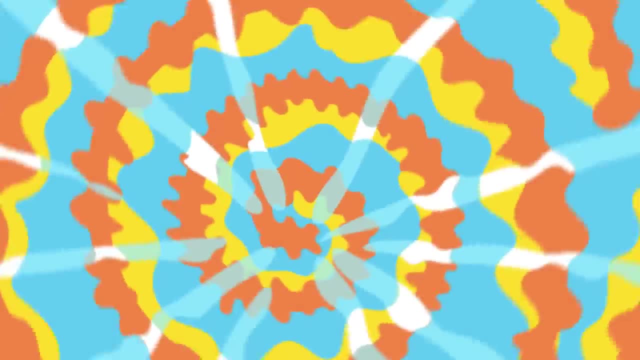 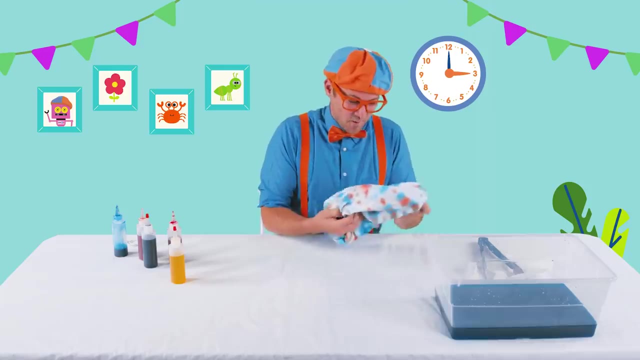 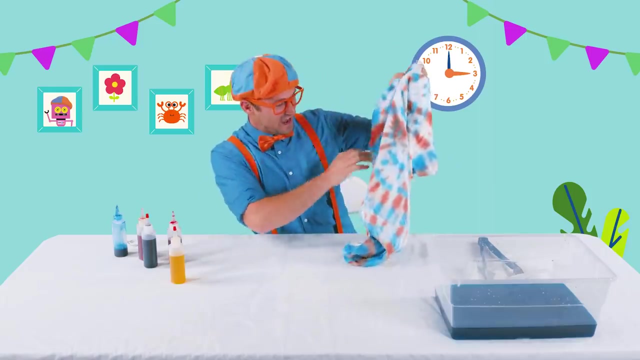 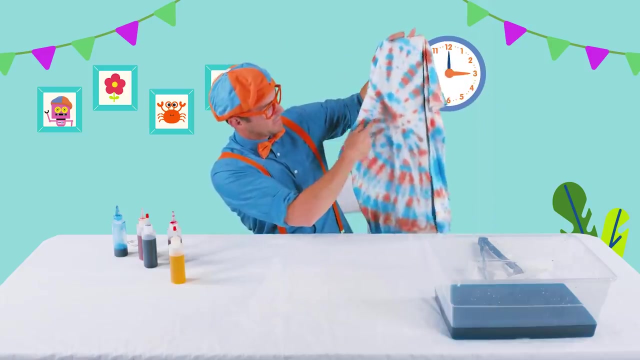 i'll be right back, okay. wow, this is awesome. our shirt is complete. wow, all right, here it is. do you see it? wow, yeah, it's blue and orange. can you see how it where? i swirled it right about there? whoa, it's so cool. time to try it on. 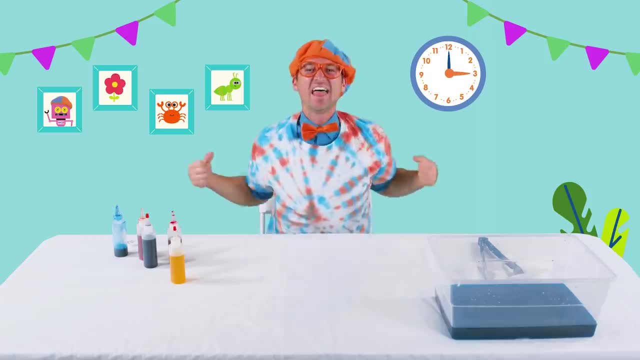 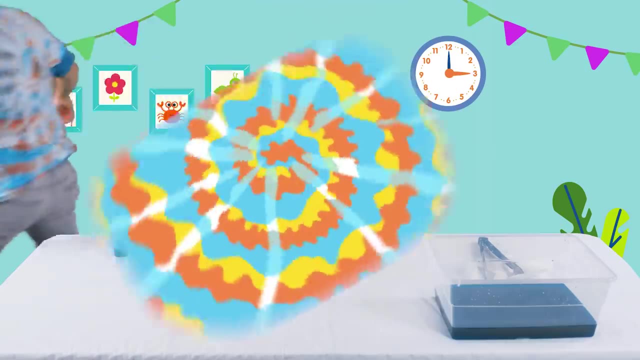 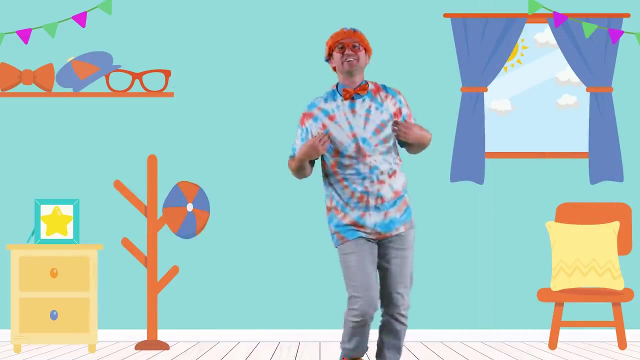 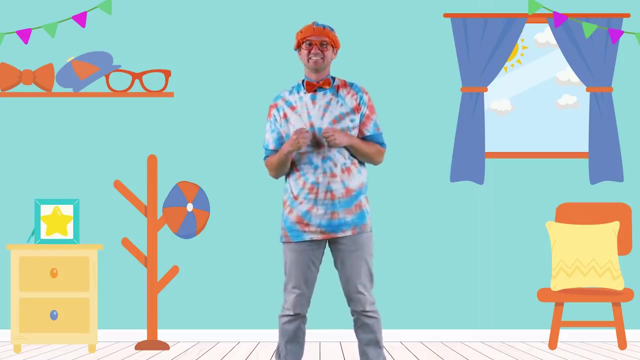 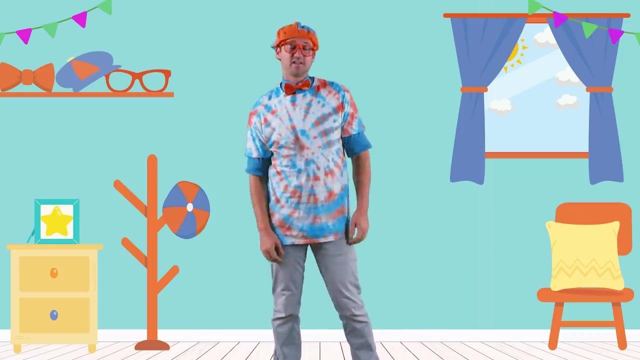 wow, how do i look? that was awesome. i love making tie-dye shirts. yeah, i sure do love tie-dye shirts. whoa, maybe now at home, you can make your very own tie-dye shirt. i am so excited to see the creation that you make. all right, well, this is the end of this video, but 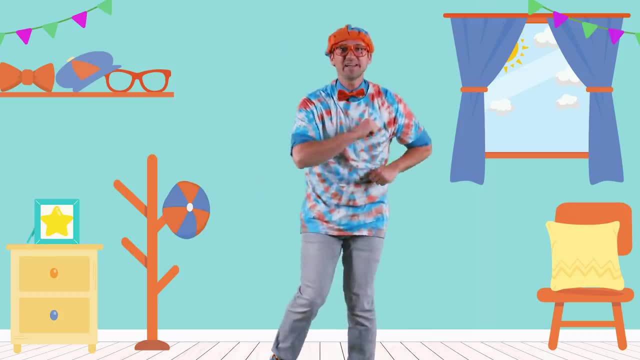 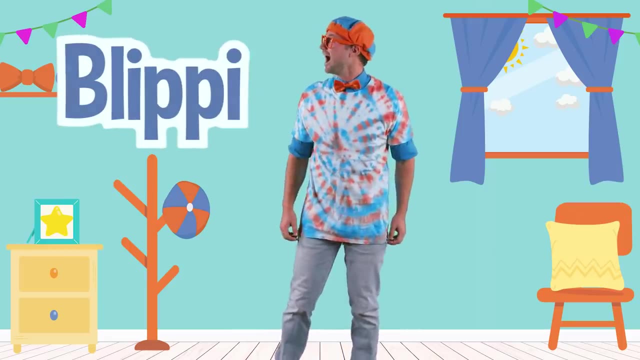 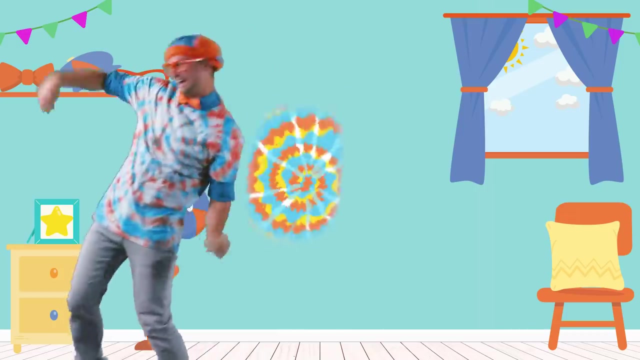 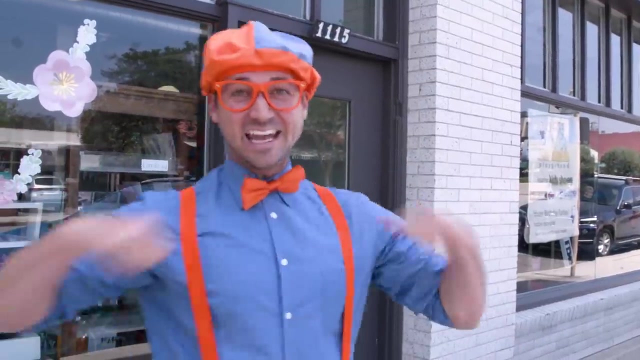 if you want to watch more of my videos, all you have to do is search for my name. will you spell my name with me? b-l-i-p-p-i, blippy, good job, all right, see you later. so much to learn about it'll make you want to shout: blippy, hello, it's me blippy, and today we're. 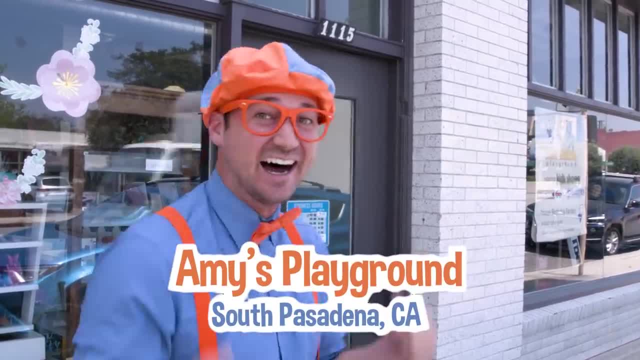 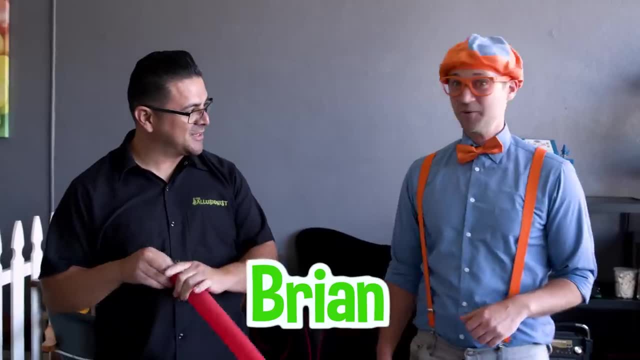 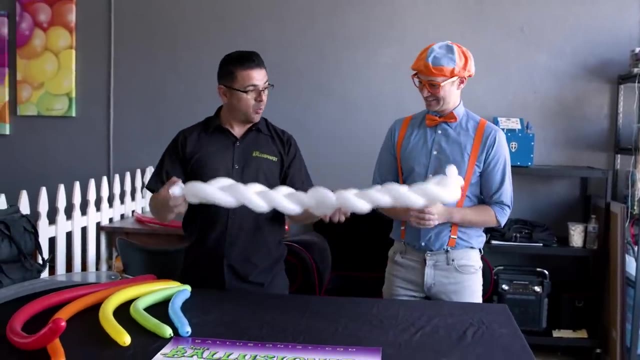 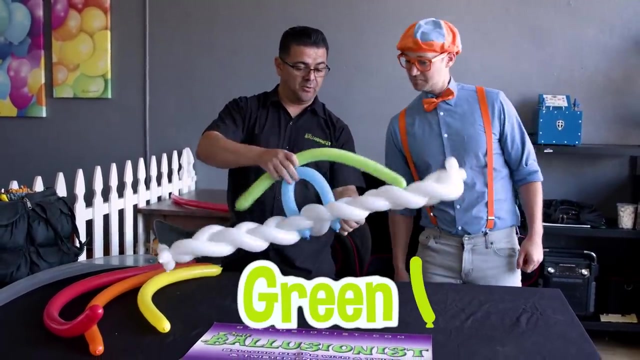 at amy's playground in south pasadena, california. come on, hey, who are you? i'm ryan the volusionist. oh, that's cool. what are you doing? i'm building a rainbow, oh, a rainbow. first thing we need is a white cloud- okay, a blue. i don't know what you call it a green one. okay, blue, green. 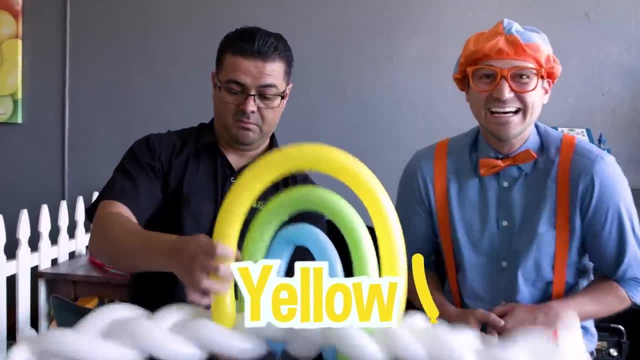 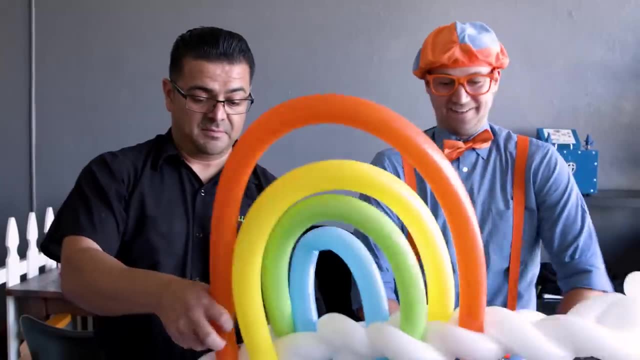 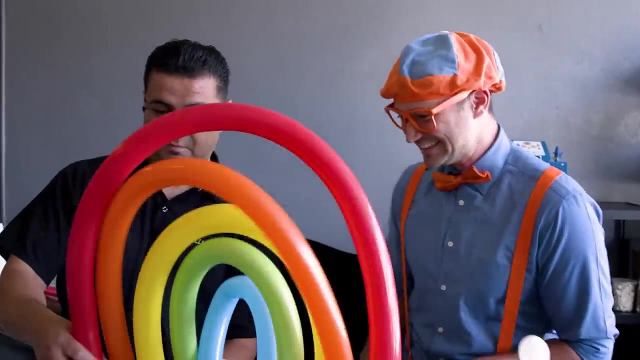 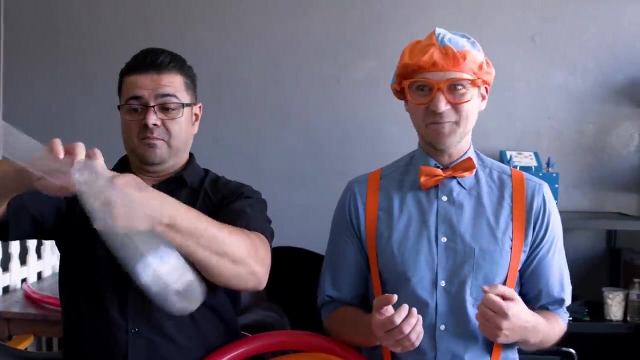 yellow, okay, yellow, just like the color of the sun. orange, orange, one of my two favorite colors, see red, red. i love the color red too. and then we need clear for this extra special move right here. oh, what's he gonna do? i don't know. i'm so excited. we'll find out, won't we? yep. 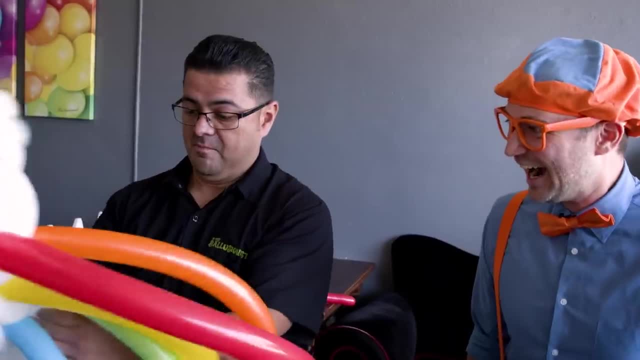 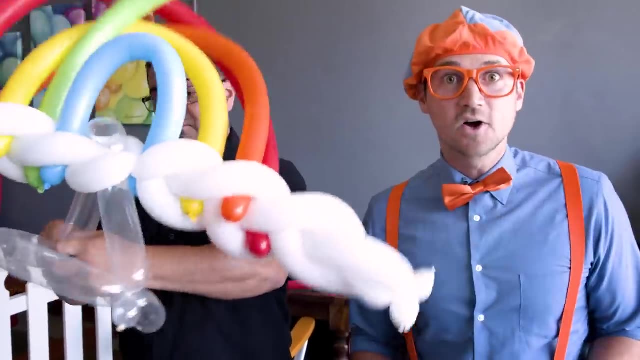 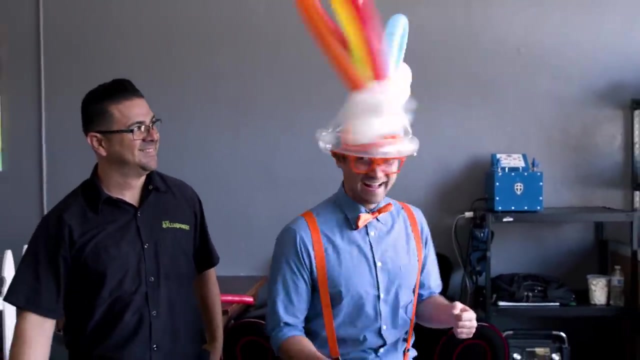 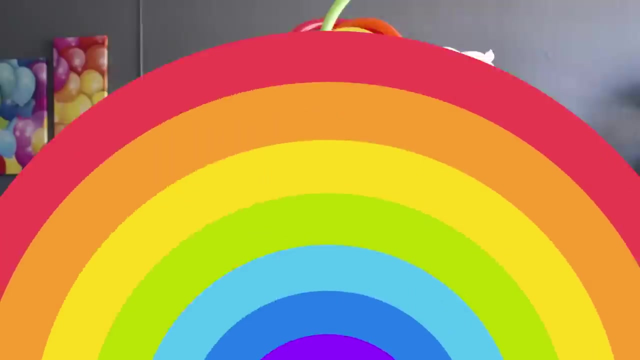 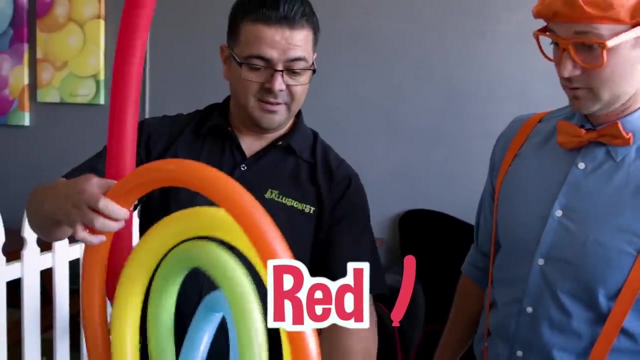 wow, i love learning my colors. cool, this is the hard part. okay, here we go, looks almost like it's complete, and there we have a rainbow. oh, look at that, that looks so cool. whoa, hey, well, thank you so much. rainbows are fun. how many colors does this rainbow have? let's see red, orange, yellow, green and blue. 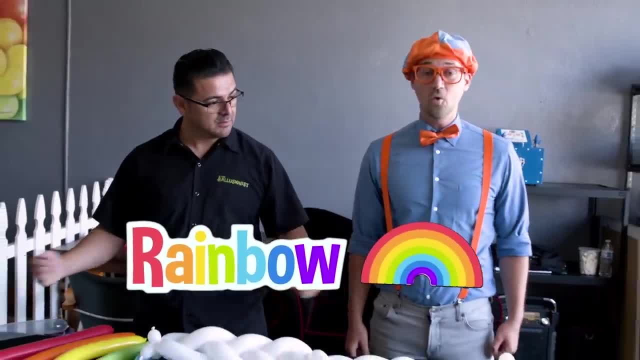 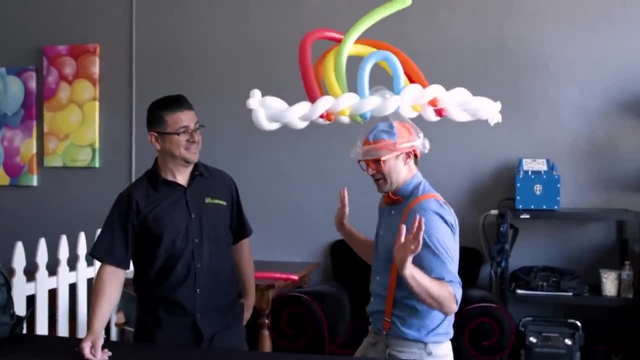 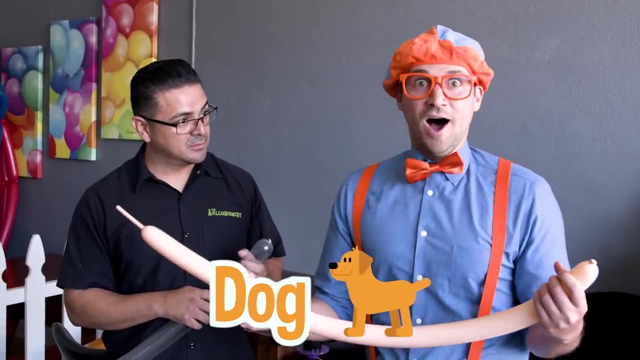 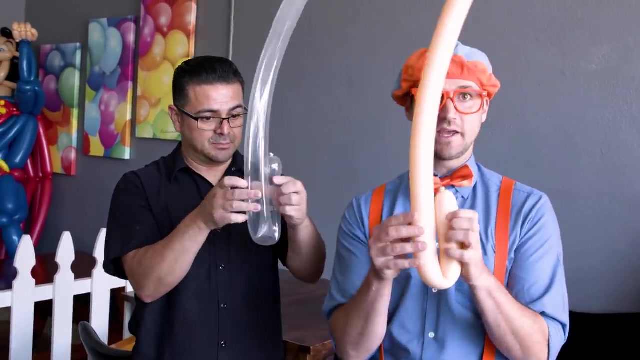 so colorful, colorful rainbow, so colorful, colorful rainbow, so colorful, colorful rainbow, so colorful, colorful, colorful rainbow, so colorful, colorful rainbow. would you like to learn how to make a balloon dog a dog? i love dogs. all right, start from here. okay, create sort of a u-shape, okay. 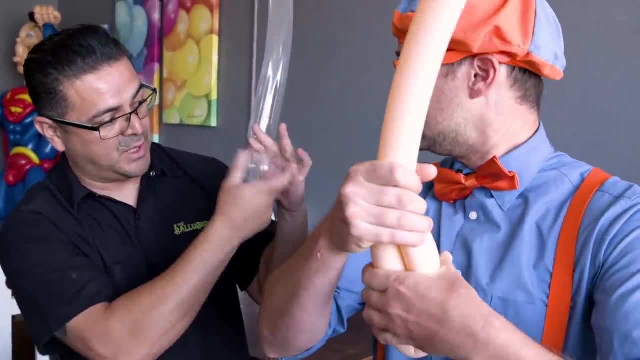 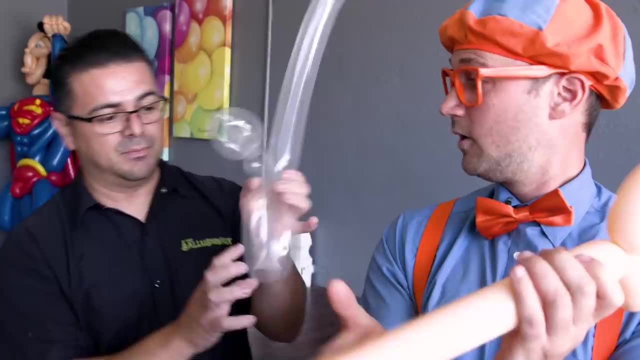 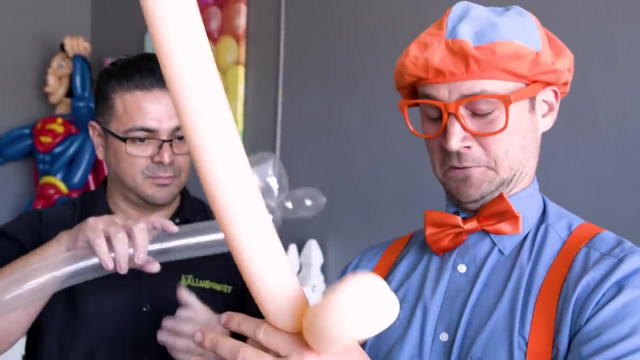 and then tightly squeeze. the tighter you squeeze, the easier it is to twist. okay, whoa, now we are going to create another u-shape. all right, tightly squeeze, leaving a bubble for a neck. okay, this is fun. and then we're going to fold the tail towards the neck. 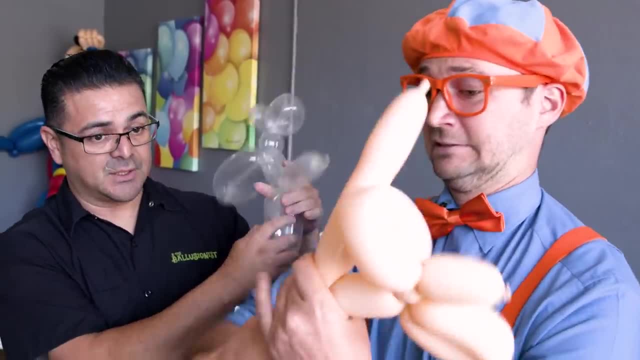 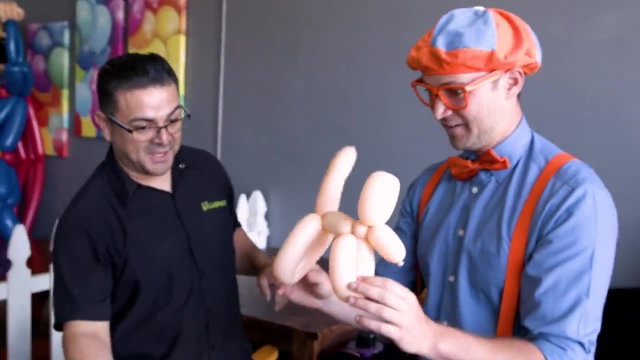 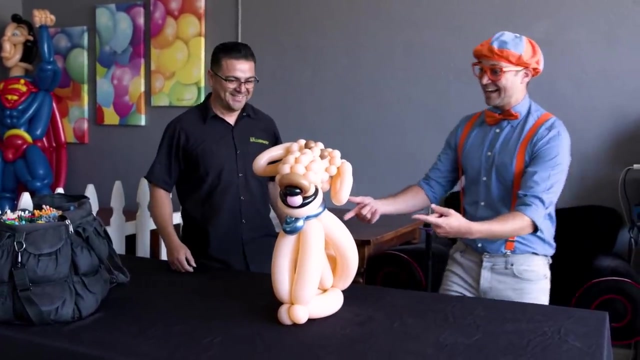 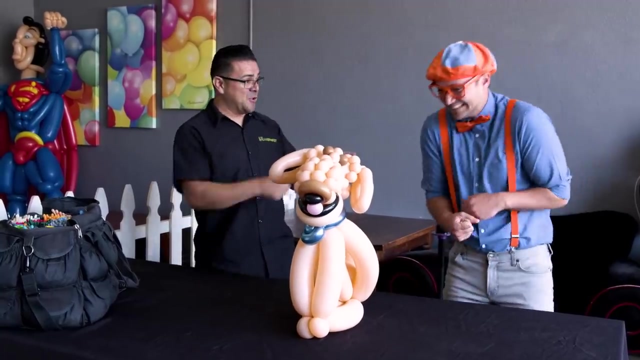 create another u-shape and tightly squeeze. all right, i'm doing it now. if you thought that was cool, why don't you place it on the table? okay, awesome, whoa, look at it, that's my dog, lino. hey, lino, that is so cool. if you think that was cool, what's this? 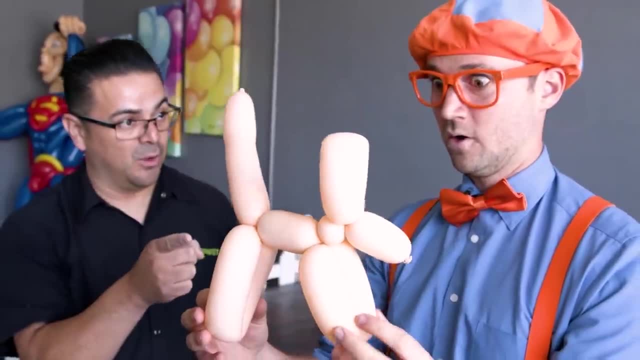 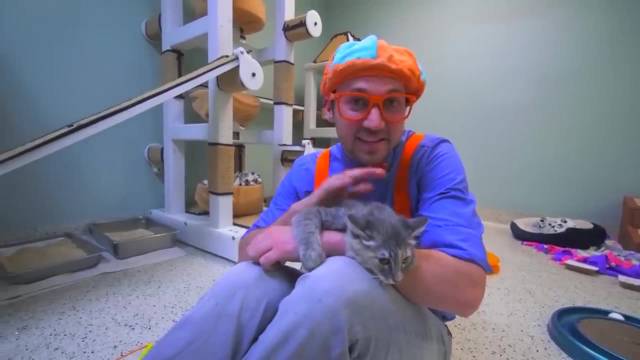 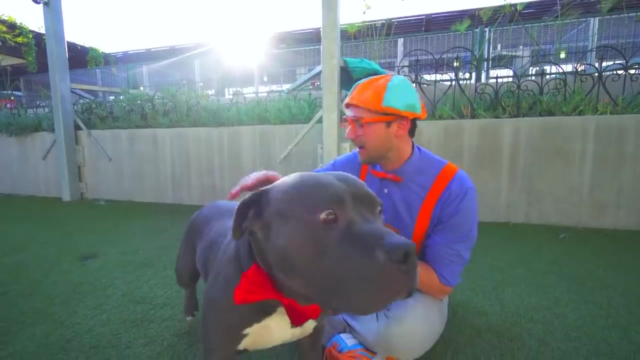 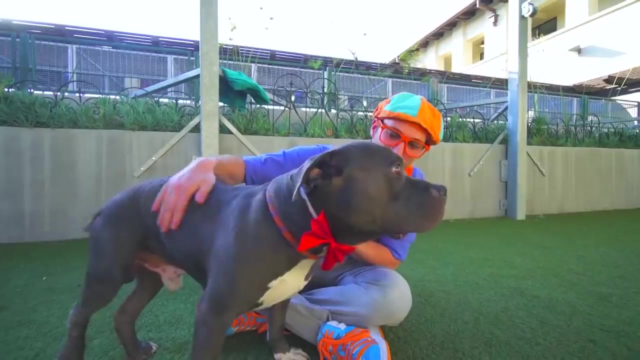 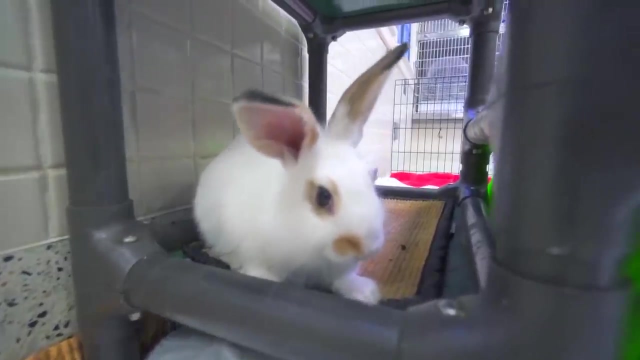 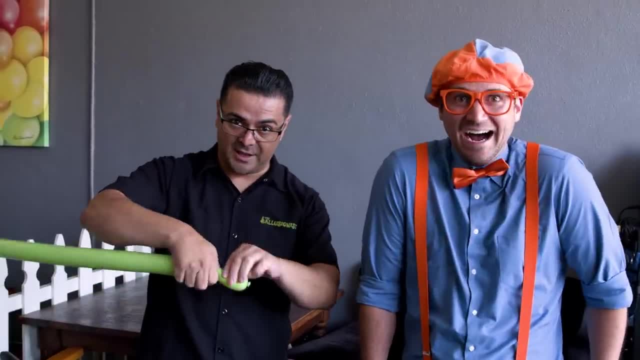 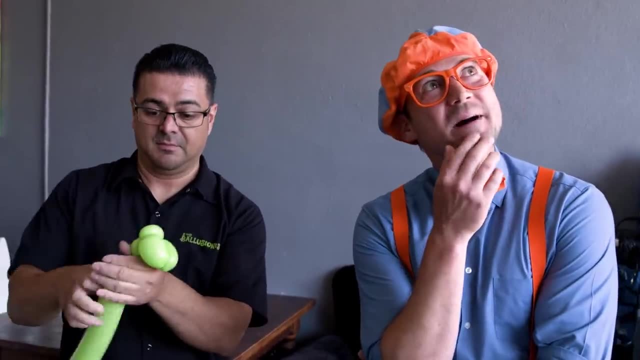 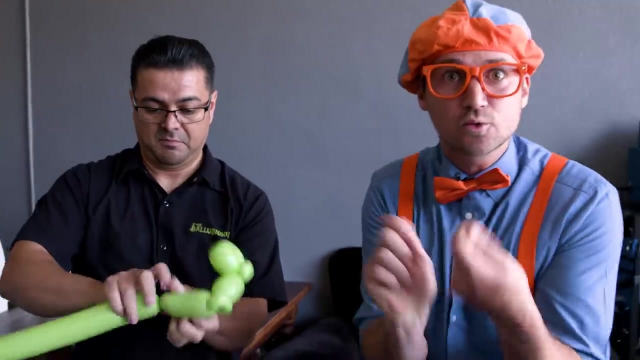 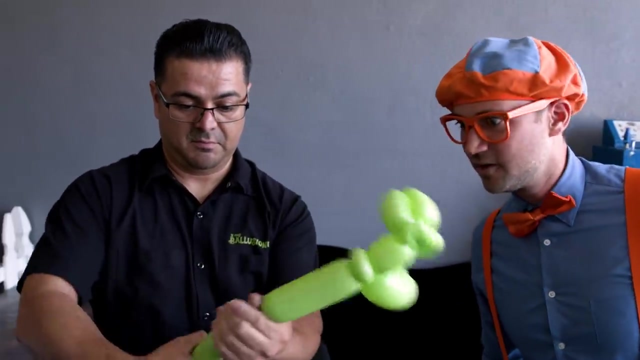 right now is just a balloon, but with a little imagination we can create a dinosaur balloon. oh, dinosaur, i love dinosaurs. wonder what one? my favorite dinosaur is so silly? whoa, look at just twisting it. whoa, do you know what color that is? yeah, a green dinosaur. 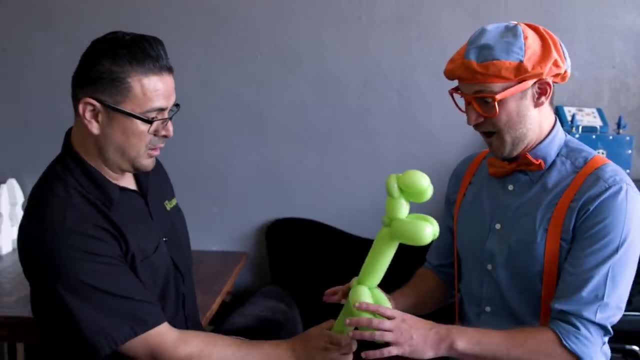 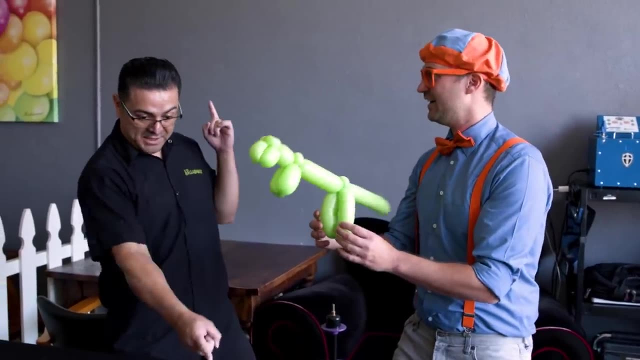 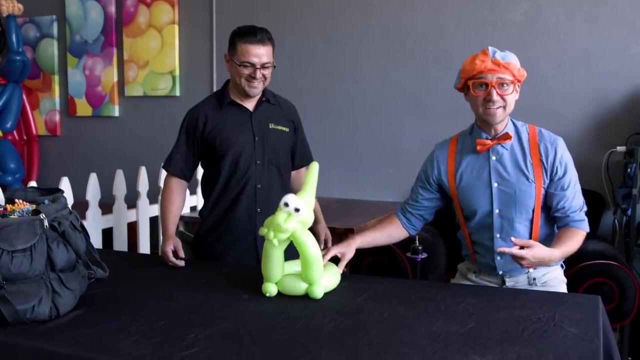 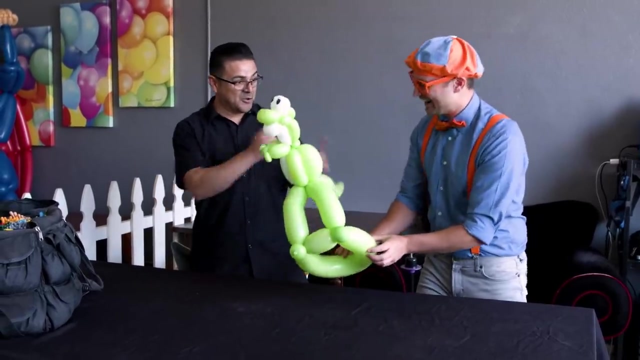 whoa, there you are. whoa, it's a t-rex. now, if you thought that was cool, place it on the table, okay, whoa? oh, look a bigger t-rex. that is so cool. now, if you thought that was cool, check this out, whoa. 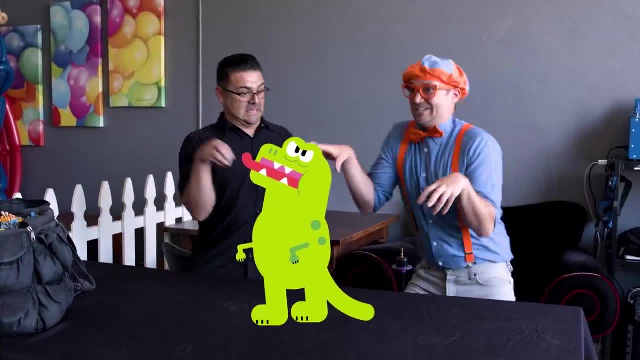 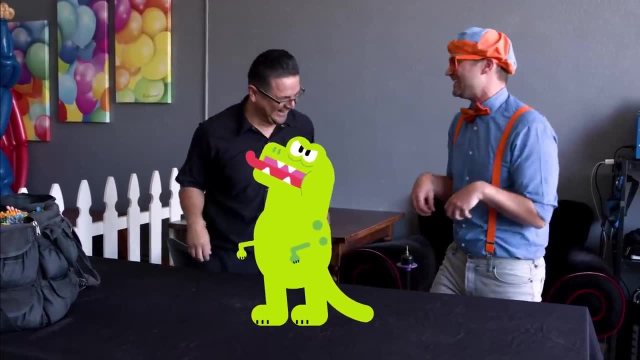 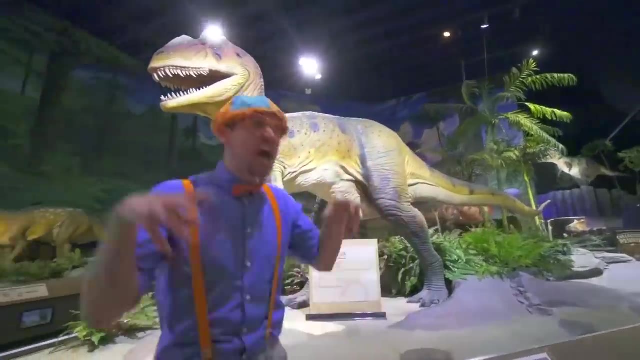 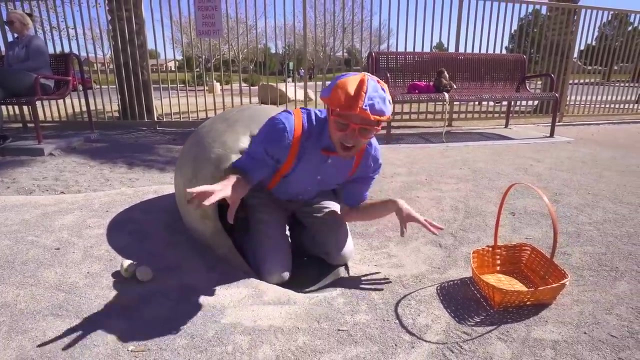 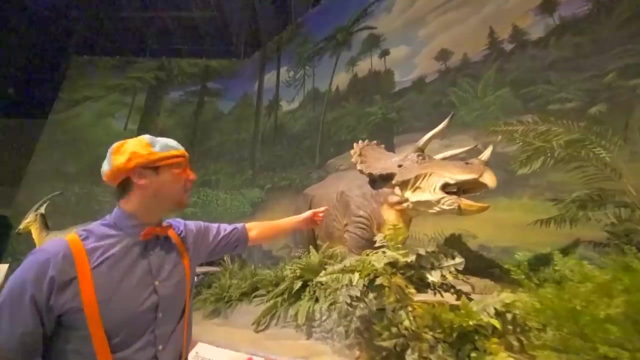 let's act like t-rexes together. ready, that was so cool. thank you so much. whoa, what a scary t-rex. let's dance to this dino song: scary scary Camila. scary scary dinos raptors and t-rex. scary dinos raptors and t rex scary dinos. 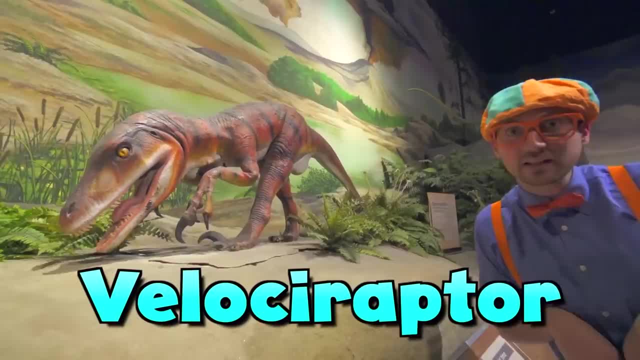 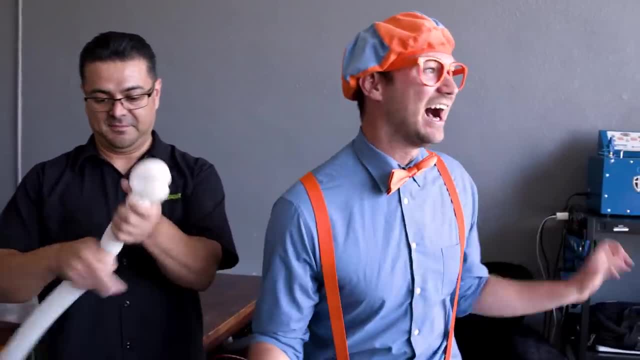 scary dino's raptors and d-rexậ� scary dinos. scary dinos. scary dinos raptors and t-rex scary. today i'm making a parrot. yeah, a parrot is a bird. i love birds. They just fly in the sky. 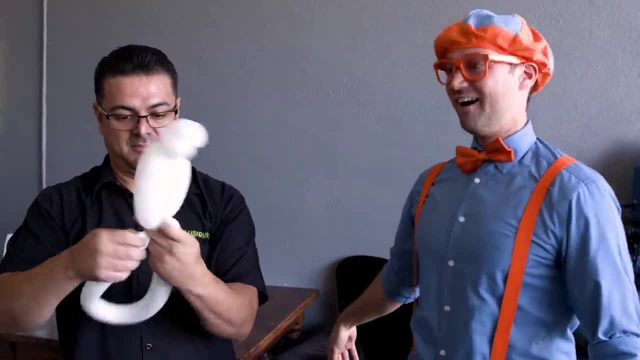 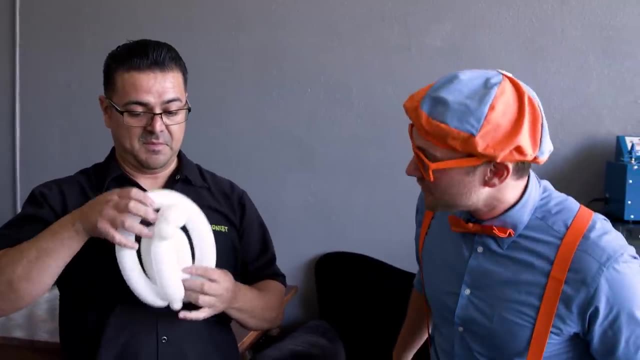 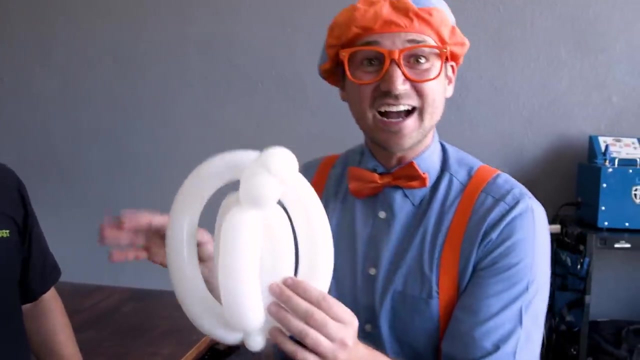 Cool, Cool. And this parrot is the color white. That is so cool. Oh, whoa, look, It's a parrot in its cage- Caw, caw. That's so cool. Now, if you thought that was cool, place it on the table. 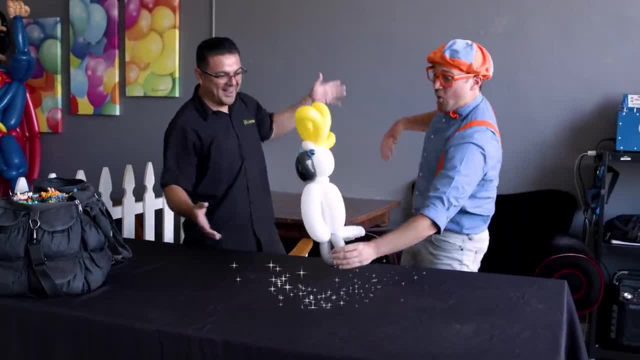 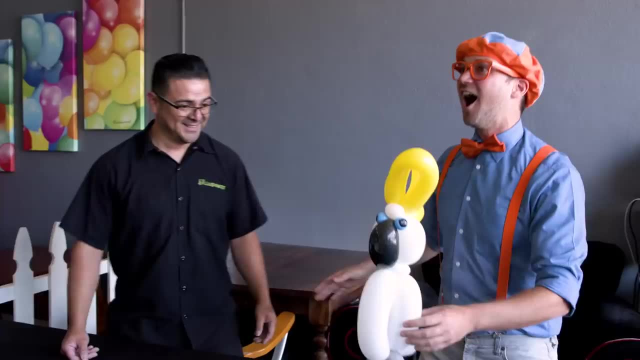 Okay, Okay, Whoa, look, It's even a bigger parrot now. Caw caw, Caw caw. Will you act like a bird? Of course, Caw caw, Caw caw. 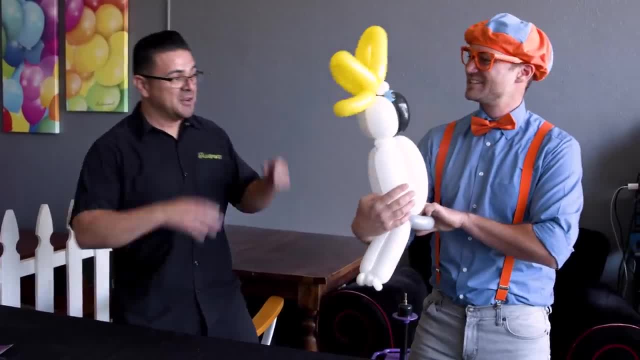 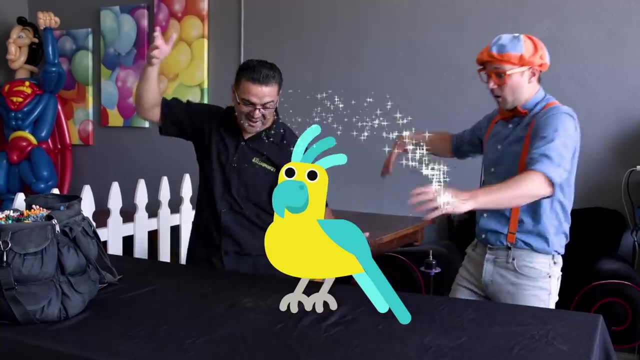 Oh, you want a cracker. That's funny. Wow, this is so cool. Well, if you thought that was cool, round two: Okay, Whoa, Whoa. look, It's a bird Caw, caw. 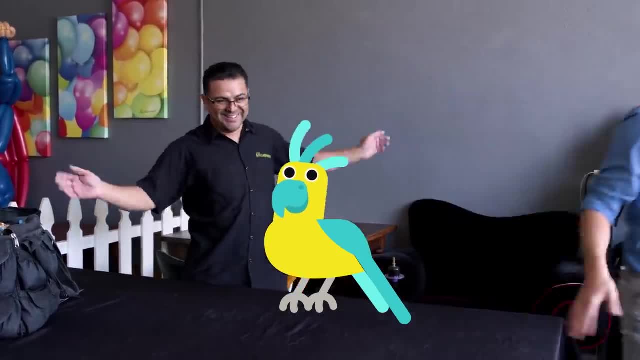 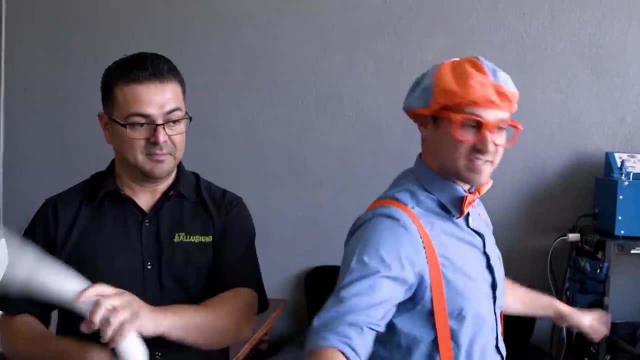 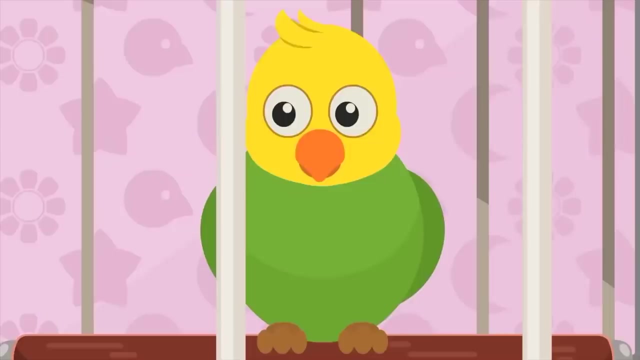 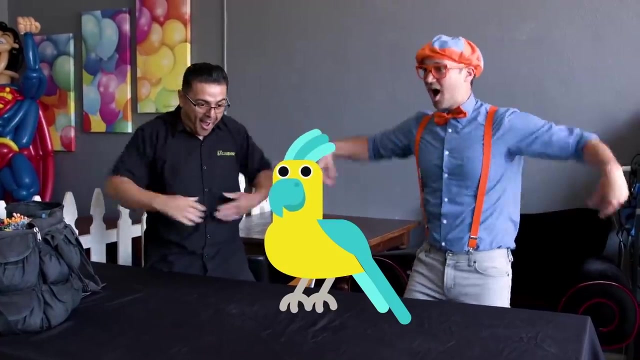 Caw caw. See you later. Caw caw. There are so many types of birds. They are so cool, They fly, and do you know what They also sing? Yeah, they sound like this Caw caw. 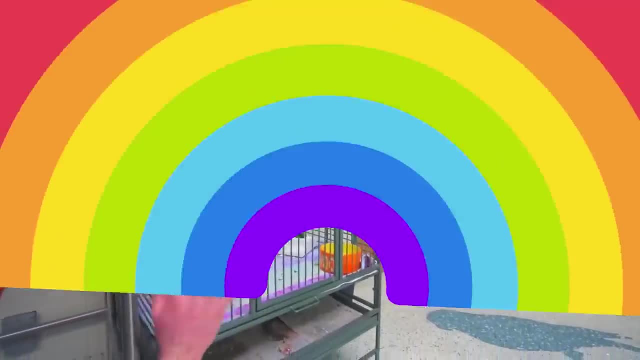 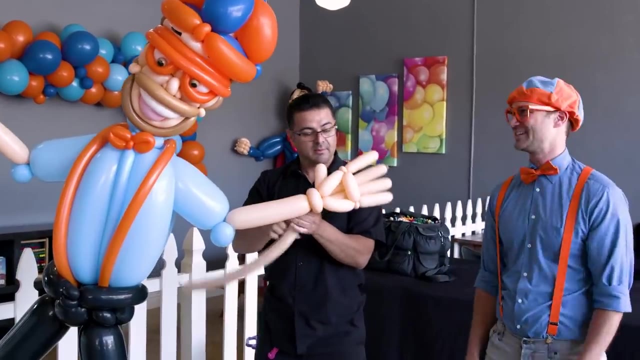 Caw caw, He is a bird- Caw, caw, Caw caw And he is a fan. Yeah, he likes to sing. Look at that thing, It's a bird, A bird, A bird. 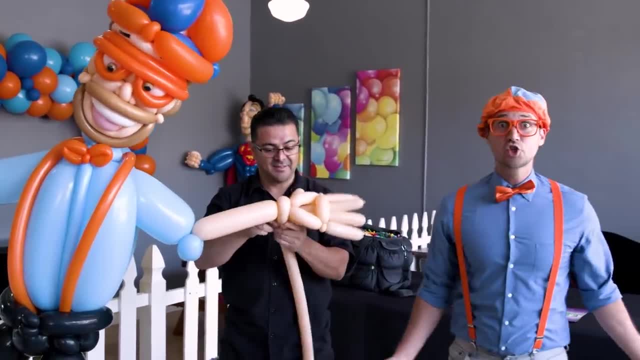 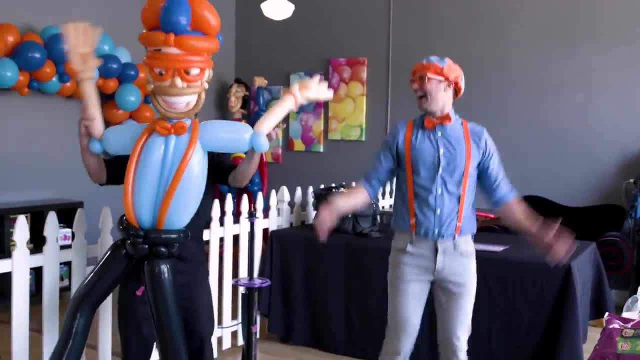 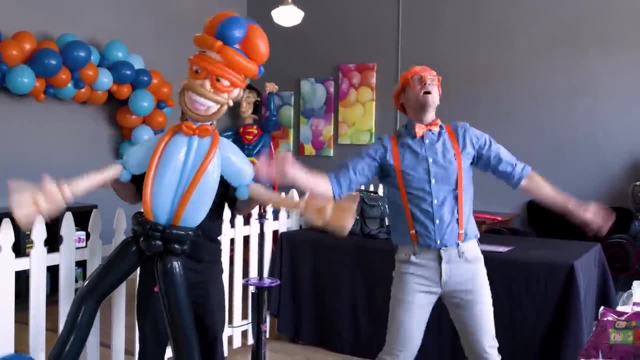 What was I doing? Jumping jacks, Jumping jacks. Really, Will you do some jumping jacks with me? Ready, Here we go. Yeah, Whoa, look at me, go. Keep it up, I'm getting tired. 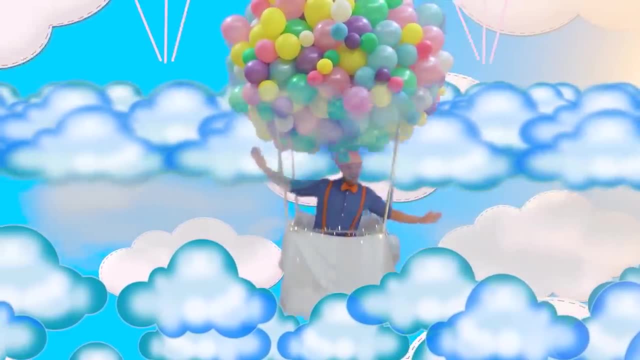 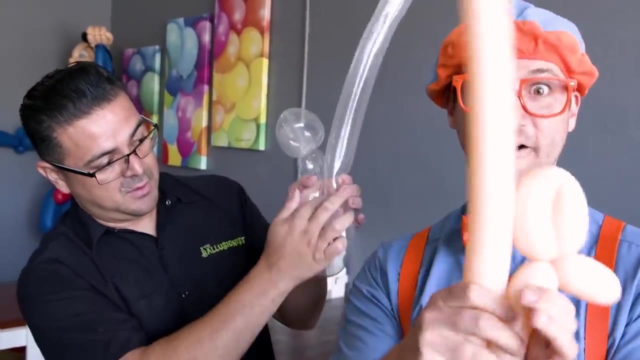 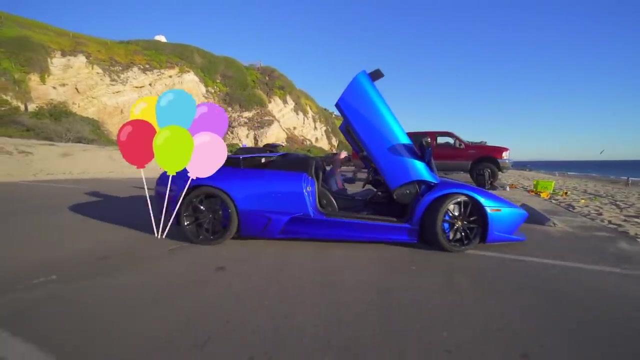 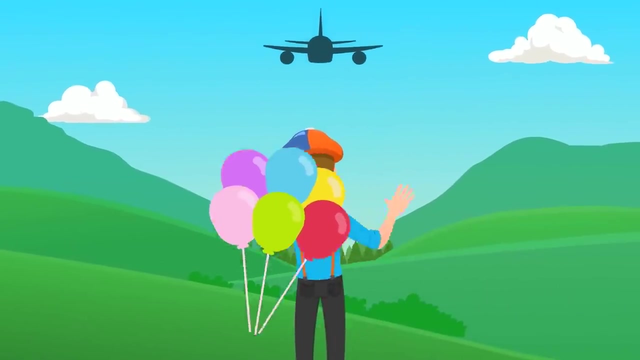 Flying high, flying everywhere. Colorful balloons are all around. Don't bop em, they'll make a loud sound. Flying high and flying low- Let's see how far they're gonna go. Flying left, flying right, Flying far and out of sight. Colorful balloons flying high. 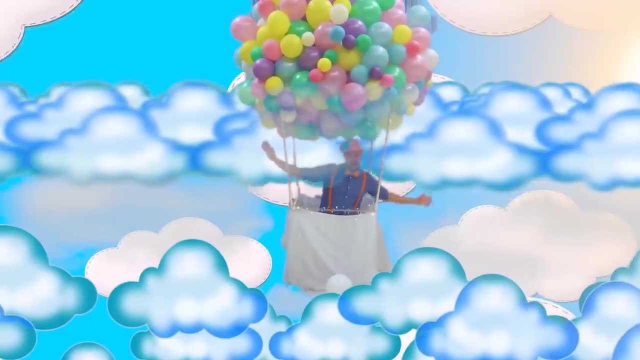 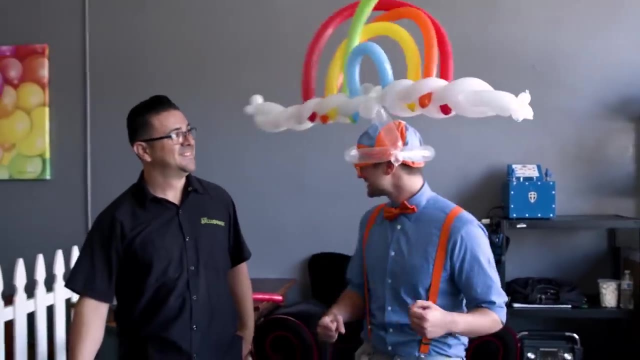 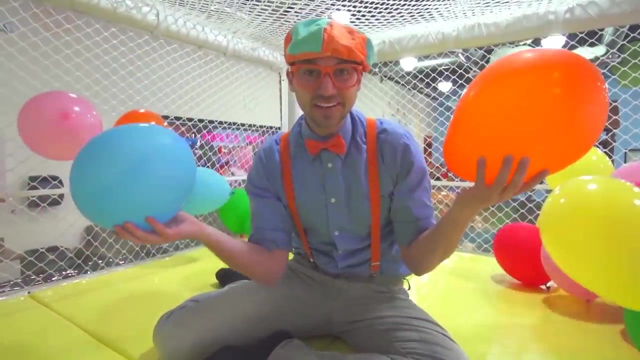 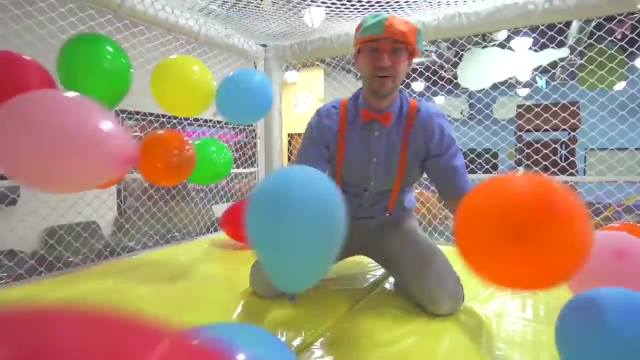 Colorful balloons up in the sky. Colorful balloons, so many colors. What is your favorite one? Some are red and some are blue, Some are orange. my favorite two In the air: flying free Balloon fun for you and me, Flying high and flying low. 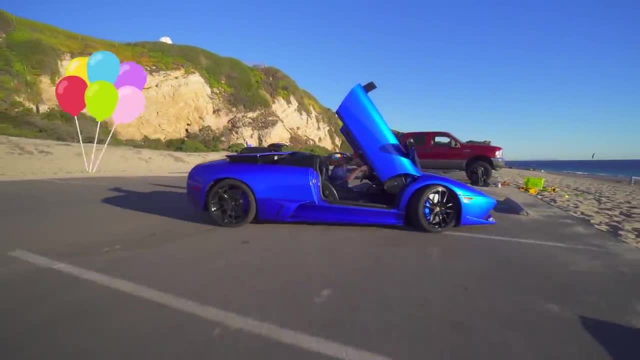 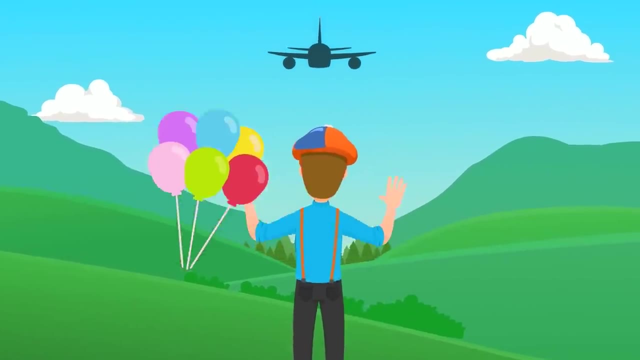 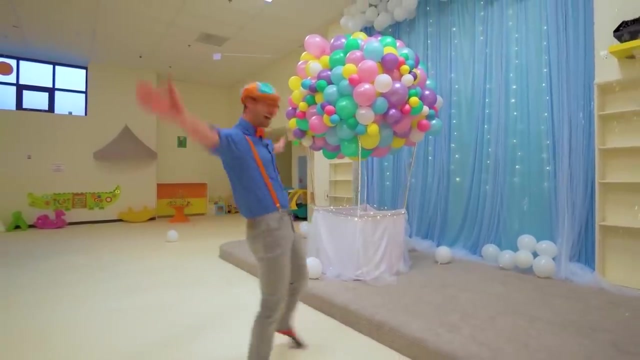 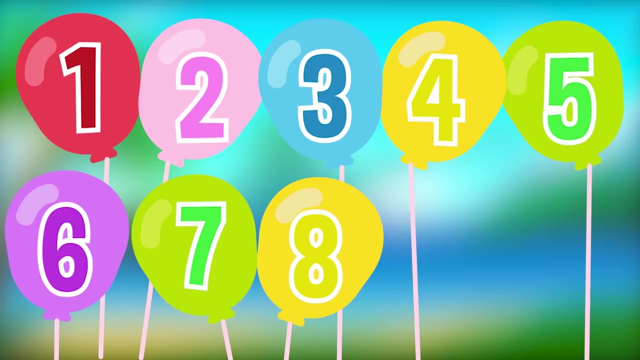 Let's see how far they'll go. Let's see how far they're gonna go, Flying left and flying right, Flying far and out of sight. Now, how many colorful balloons can you see? Here we go. One, two, three, four, five, Six, seven, eight, nine, ten. 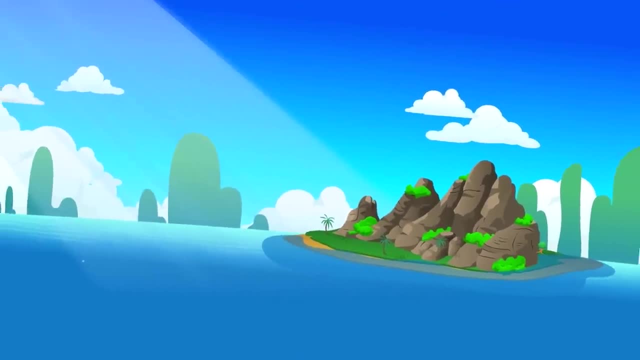 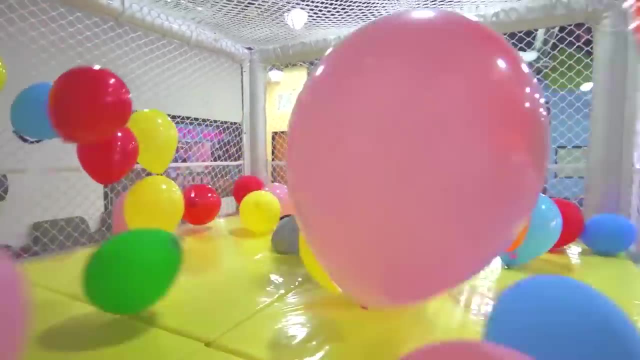 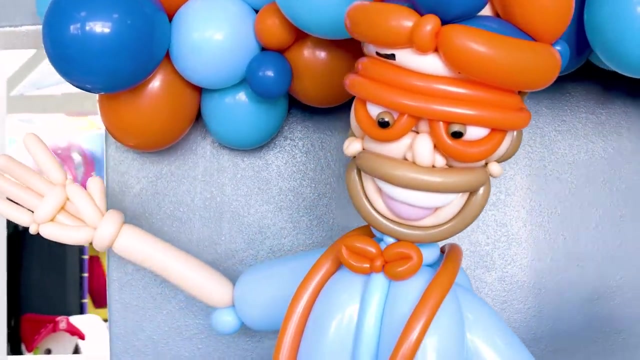 Colorful balloons flying high. Colorful balloons up in the sky. Colorful balloons- so many colors. What is your favorite one? Whoa, That was so much fun playing at Amy's Playground in South Pasadena, California. Well, this is the end of this video. 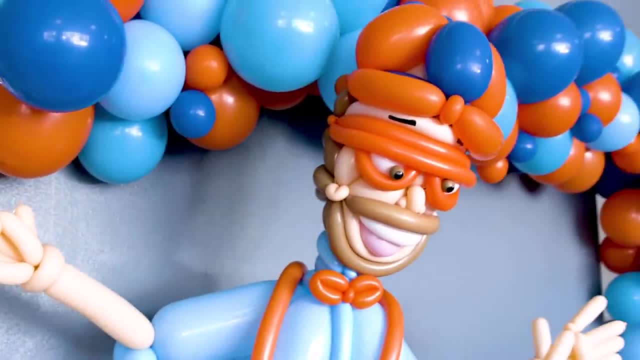 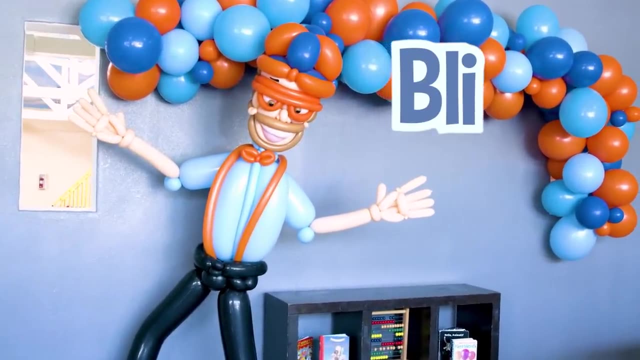 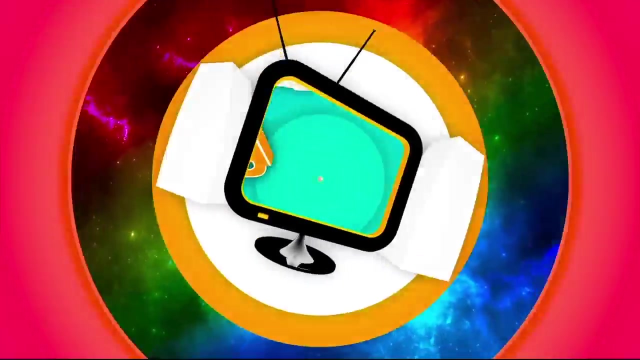 but if you want to watch more of my videos, all you have to do is search for my name. Will you spell my name with me? B-L-I, P-P-I, Blippi, Good job, Buh-bye. So much to learn about. 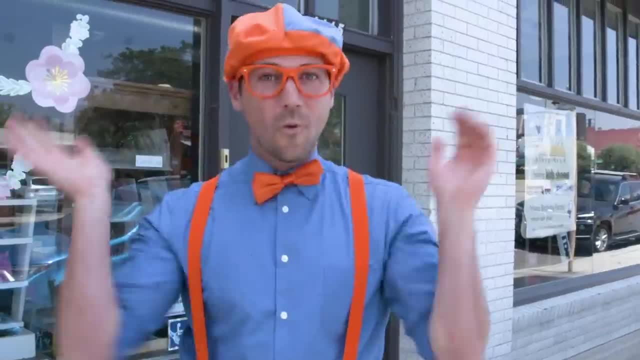 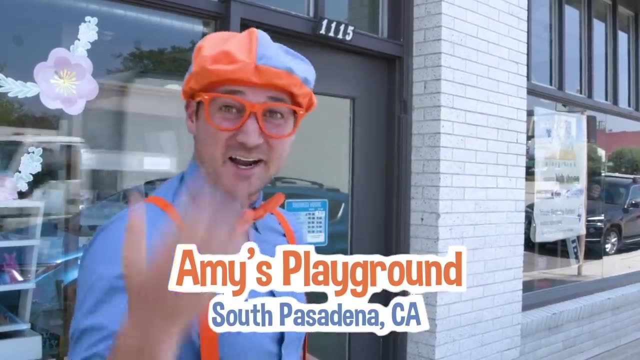 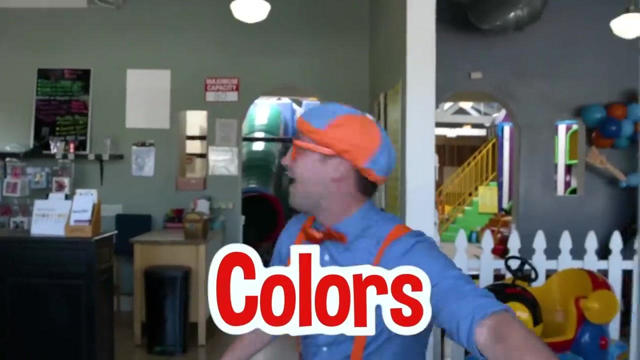 It'll make you want to shout: Blippi, Whoo, Hello, It's me Blippi, and today we're on Amy's Playground in South Pasadena, California. Come on, We're going to learn our colors. Whoa, Oh. 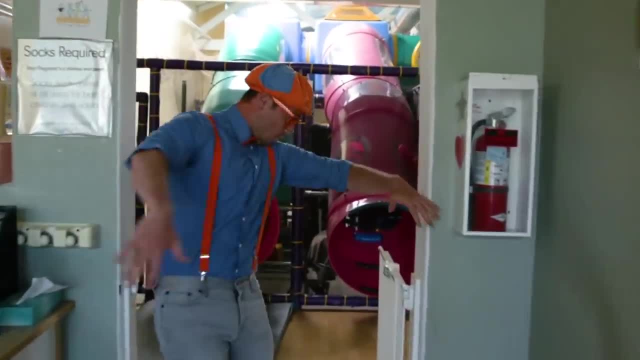 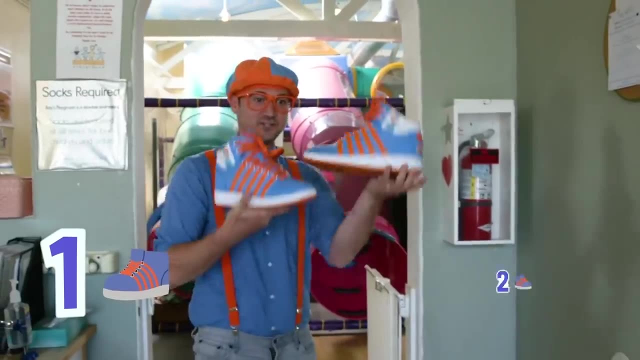 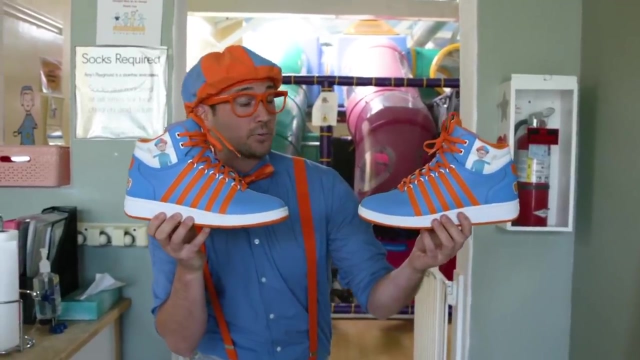 Wow, This place is so cool, Whoa, We can't go past here without taking off our shoes. Here's one shoe and here's two shoes. Hey, What color are my shoes? It looks like there is blue orange. 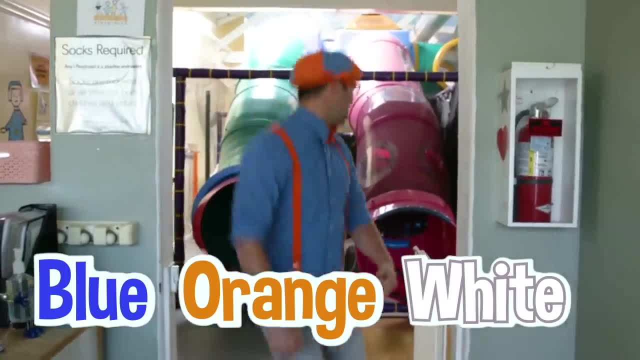 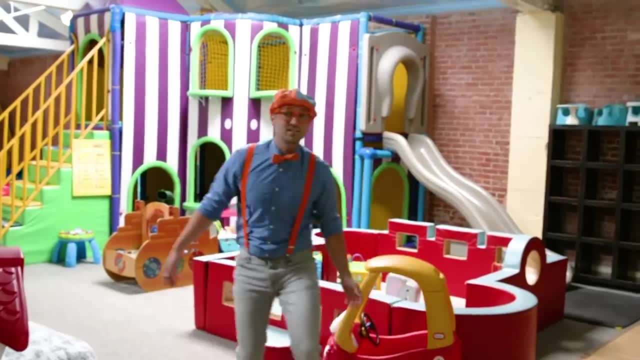 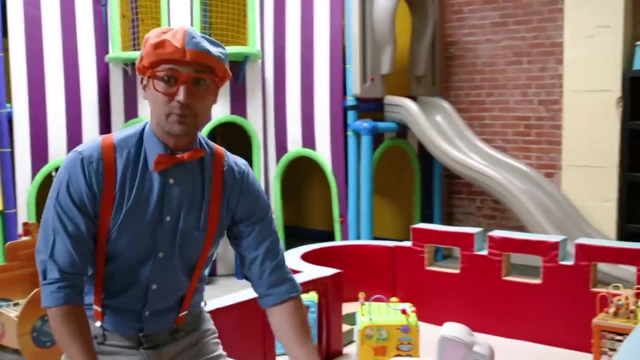 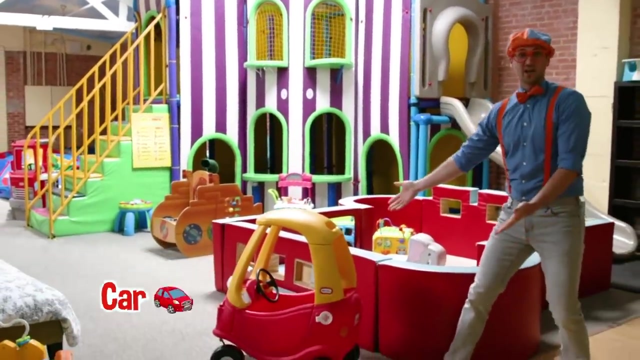 and white. Woohoo, Let's go. Whoa, This place is so colorful. Oh, I love playing around here. Oh, This is pretty colorful, Whee, Whee. Look at this car. This car is the color yellow. 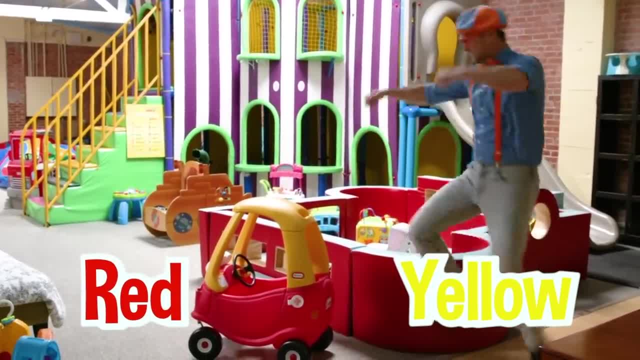 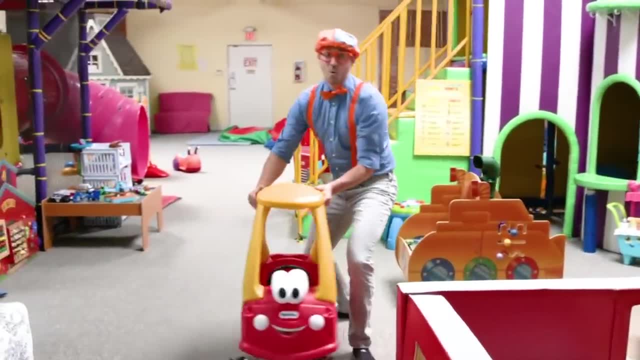 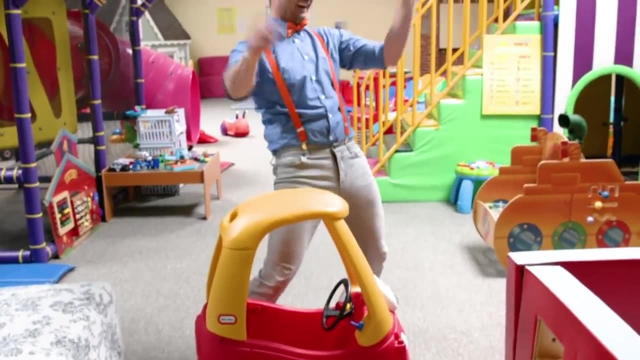 and the color red. Here we go, Whee, Whee, Whoa, Whoa, Whoa, Whoa, Beep, beep. So silly. What's in here? Whoa? It's so soft in here, Whoa. 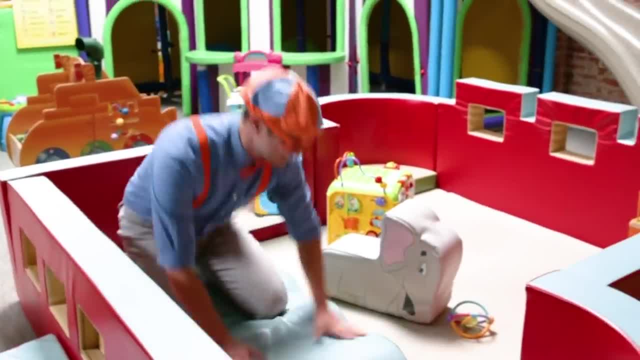 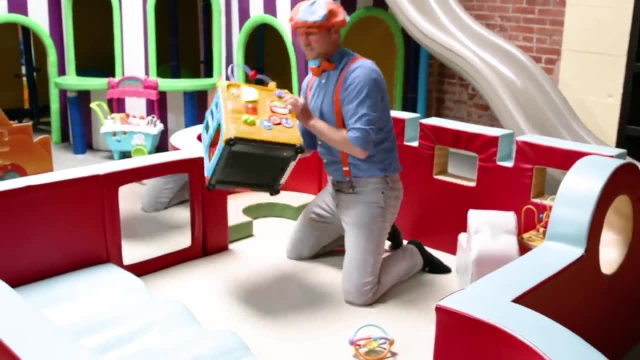 Whoa. Hey, Look at this. This box has so many colors on it. There's so many colors to name. Let's go continue to explore. Whoa, Whoa, Whoa, Whoa, Whoa, Whoa. 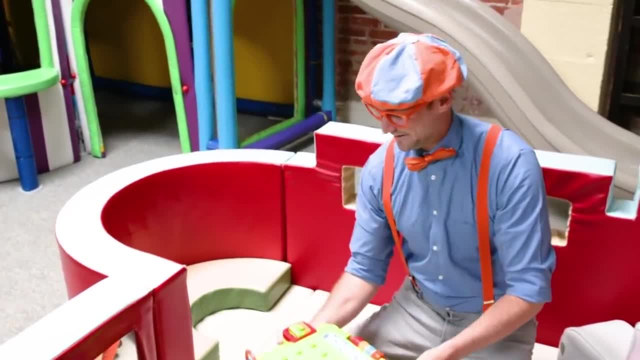 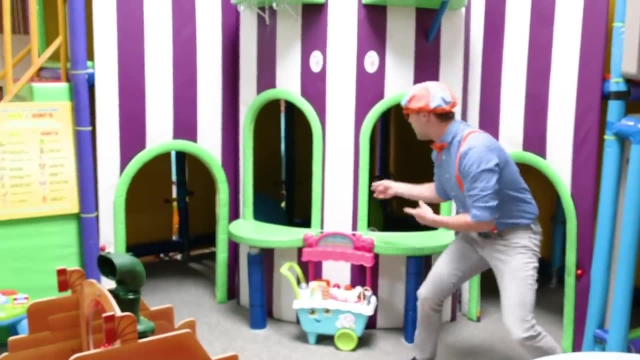 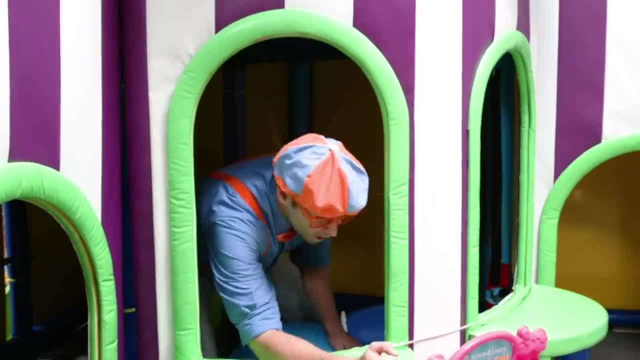 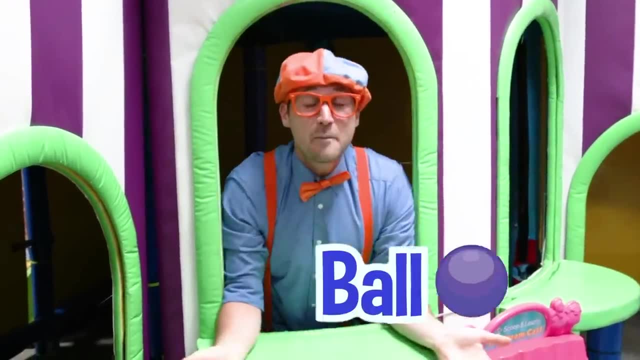 Whoa, Huh, Look at that, Whoa, It's like a castle. Let me go inside. Hello, Whoa, Check this out. That ball was the color blue. Hey, Here's another one. Whoa, That ball was the color blue. 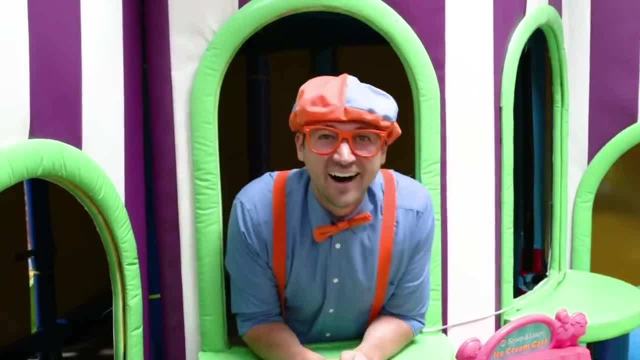 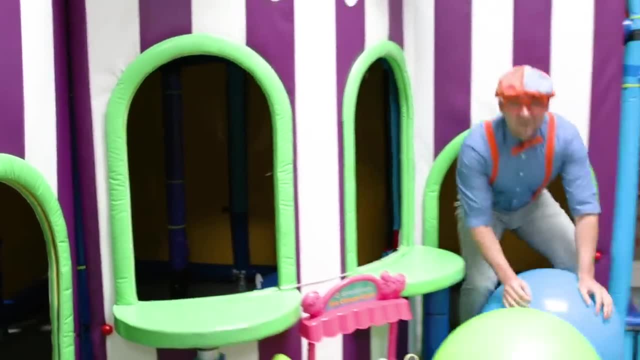 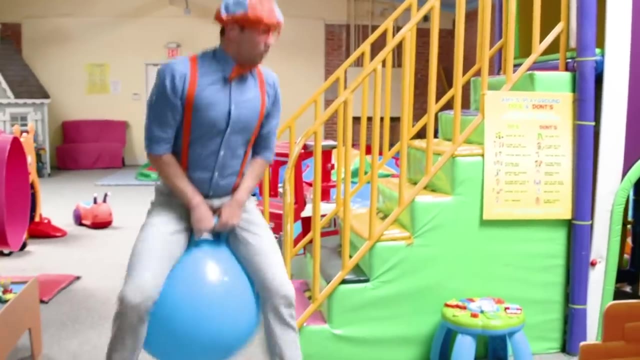 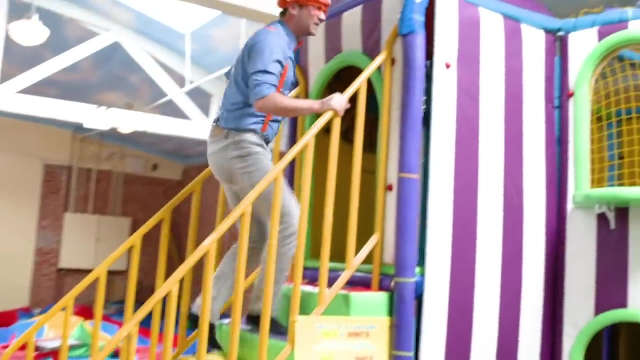 Hey, Here's another one. Whoa, That ball was the color green. Good job, Whoa, hey, Boing. Whoa, Whee, Whoa, Whoa, Wow, The castle is so tall, Whoa. 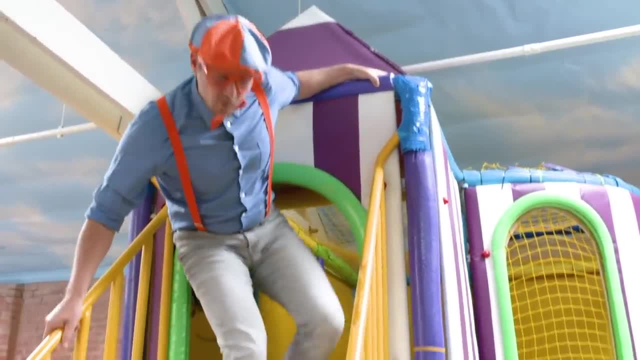 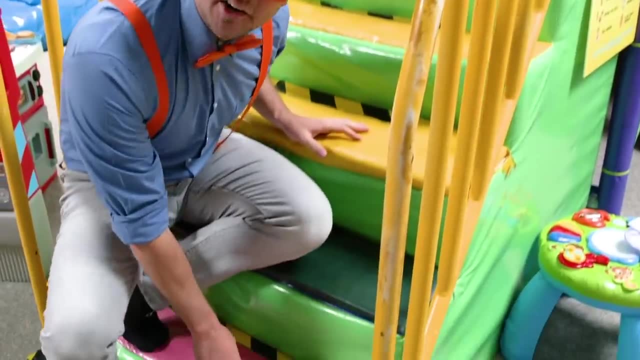 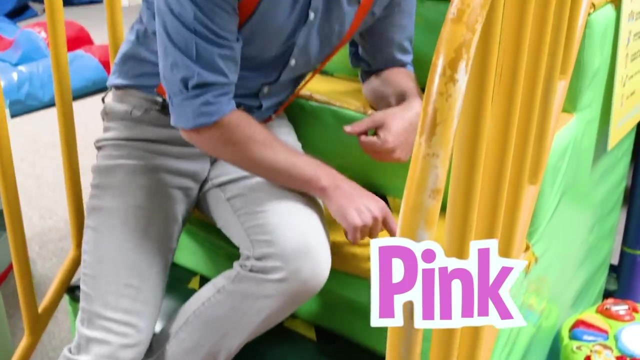 Hello down there. Hey, Whoa, look at these steps. Wow, Do you see the colors? Look at this color. What color is this? This is the color pink, This color right here. Yeah, the same color as the railings. 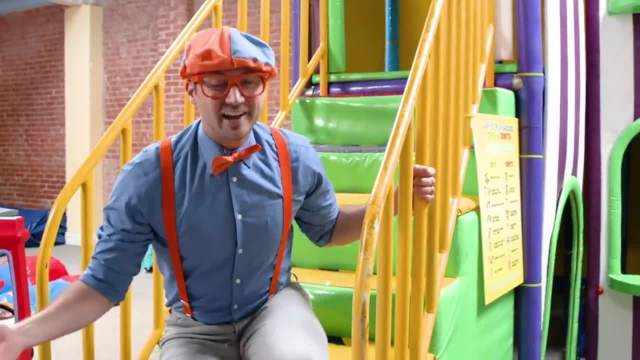 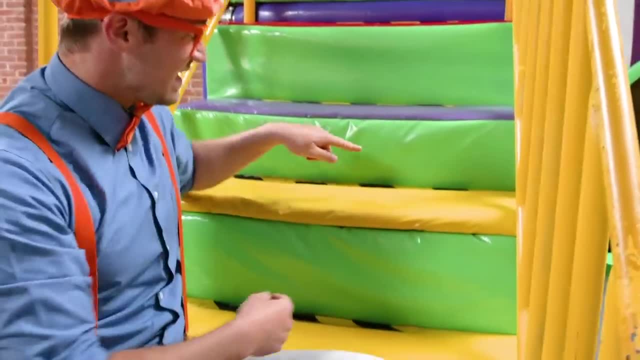 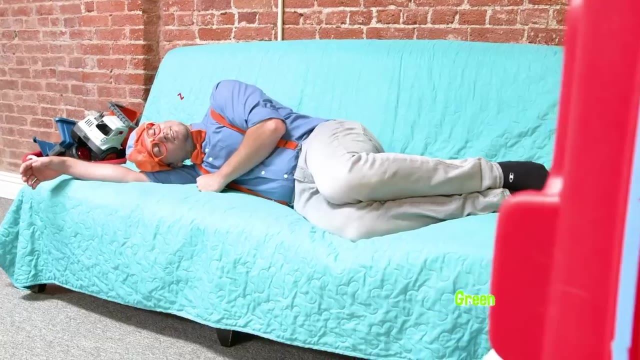 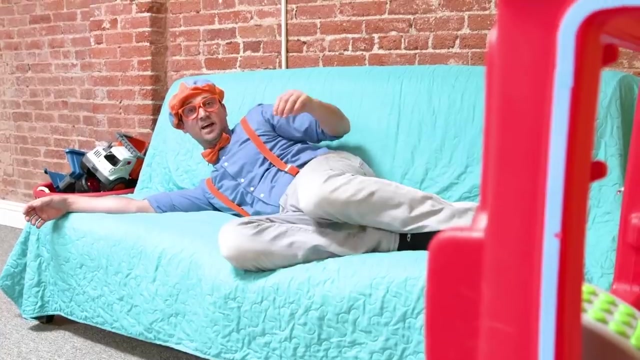 What color is this? Yeah, the color yellow. And right here, we learned this one already. This, this and this- Yeah, these are all. the color green, Green. Wait a second. No time for napping, But this is a nice comfy couch. 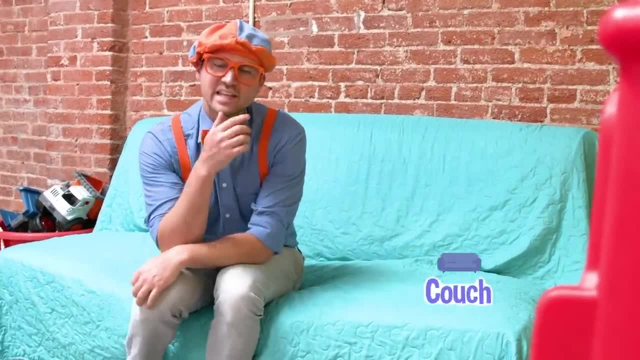 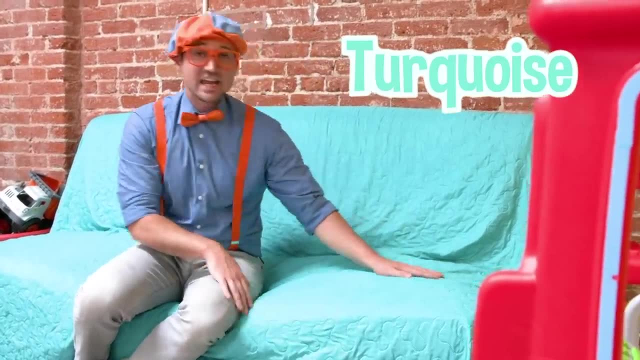 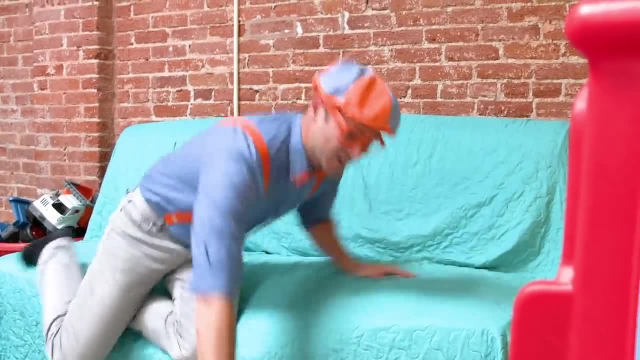 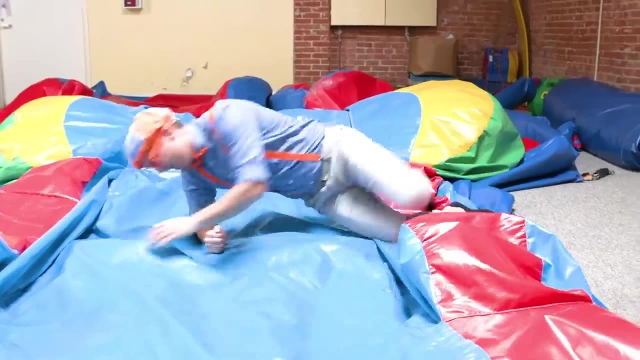 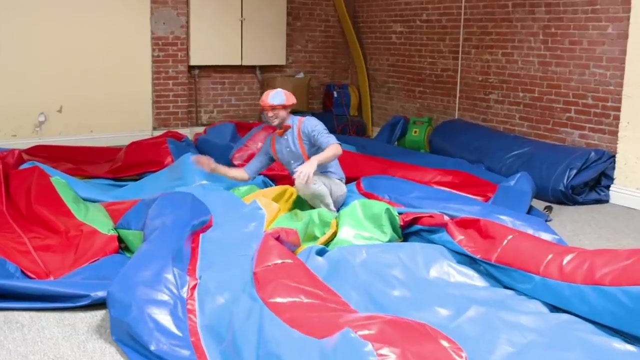 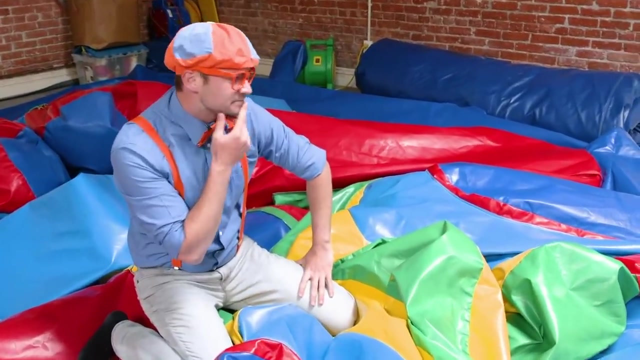 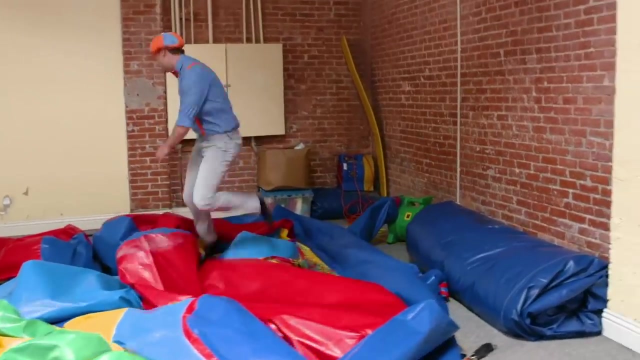 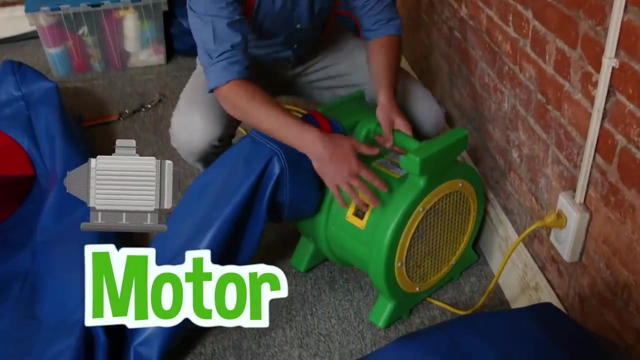 But no time for napping, It's time to do some rollin. It's so colorful and I think it's deflated. Hmm, How do we inflate this? Wait over here. This is the green motor. Yeah, this is green and yellow. 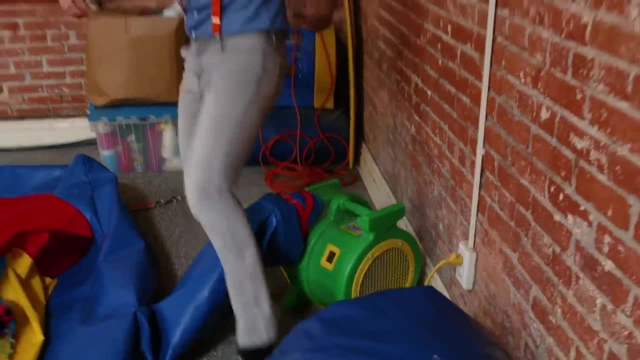 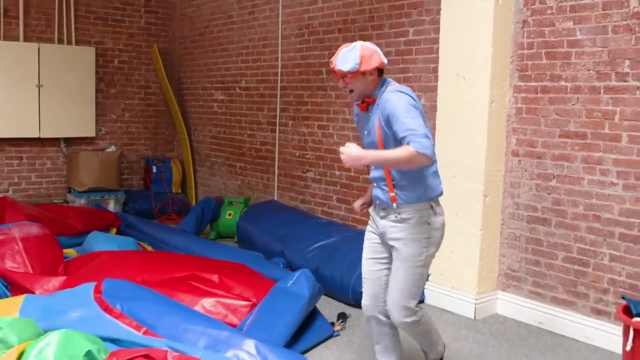 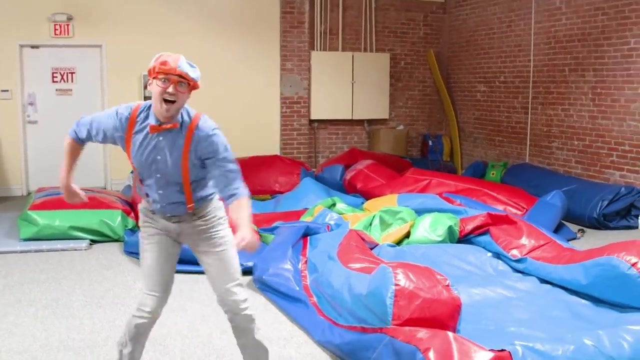 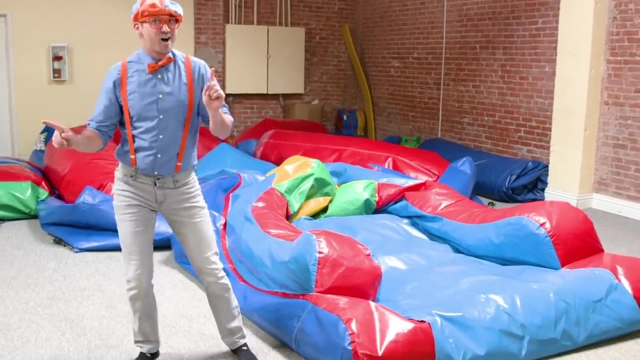 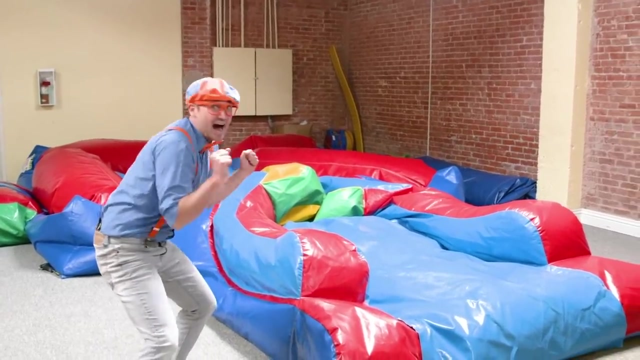 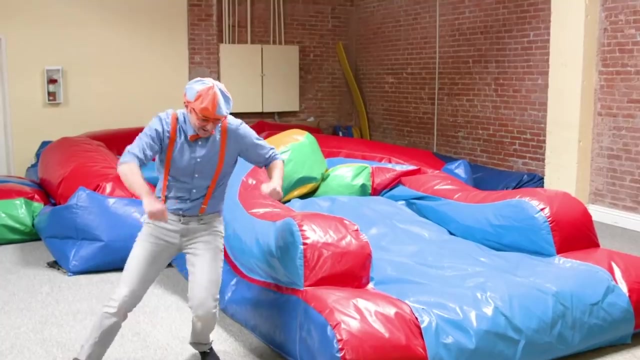 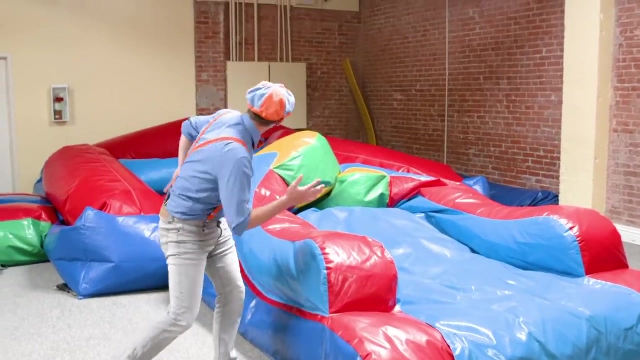 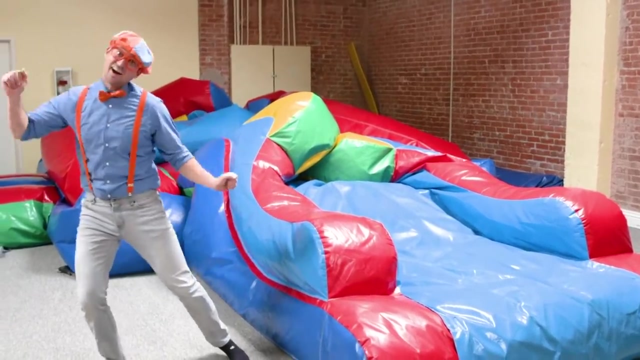 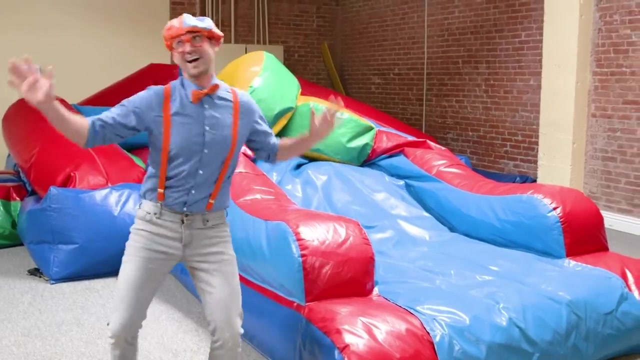 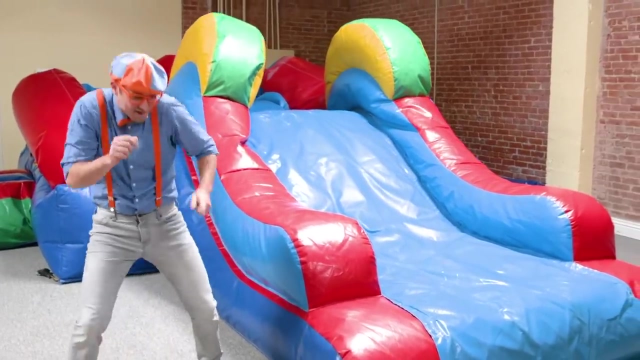 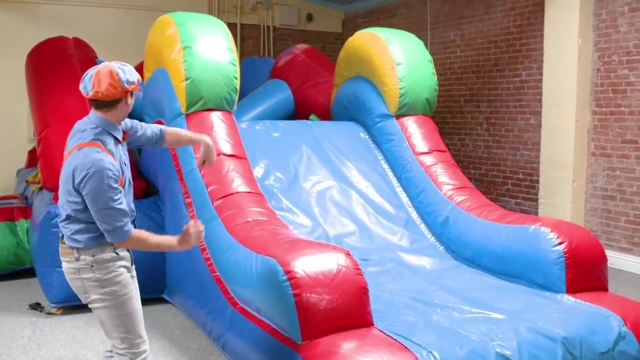 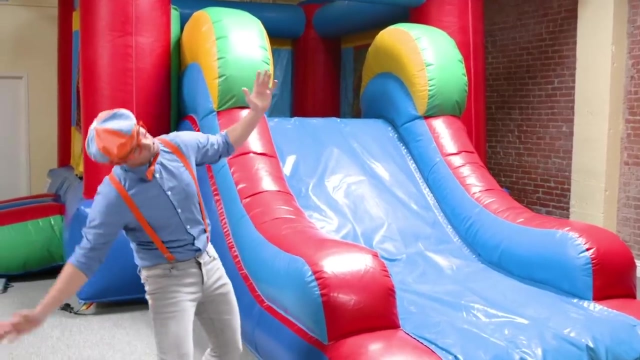 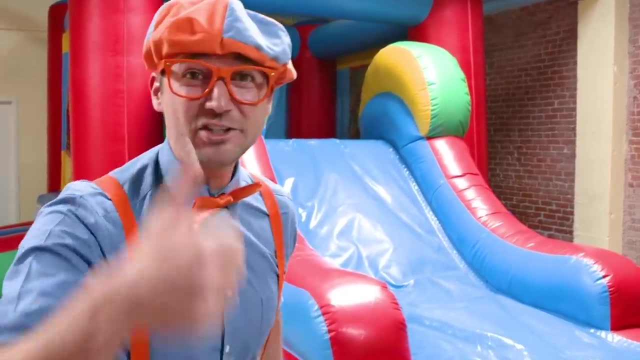 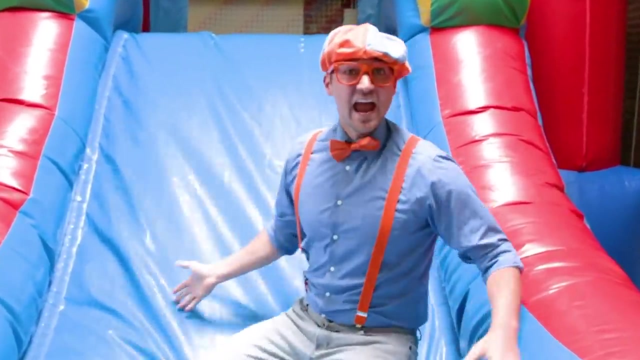 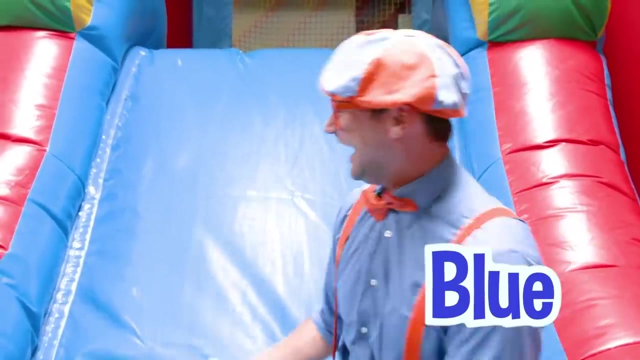 Here we go. Oh Oh, Oh, Yeah, we did it. Good job. Woohoo, Woohoo, Whoa. What color is this? Yeah, it's one of my two favorite colors. Yeah, and it rhymes with two Blue. 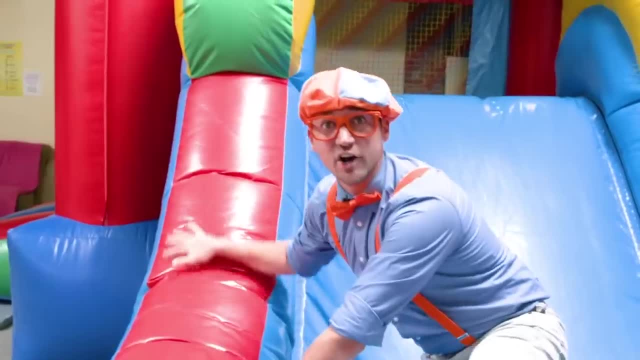 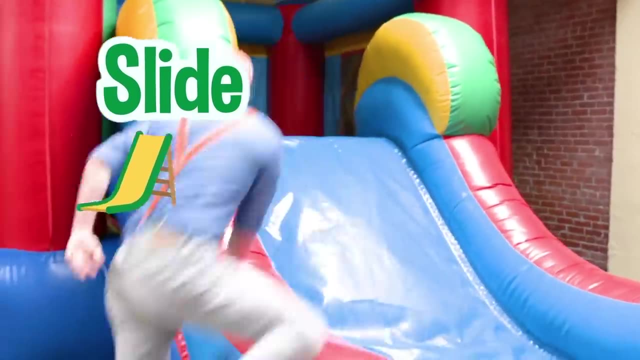 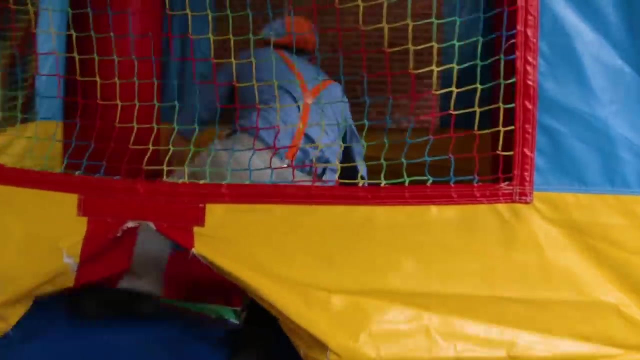 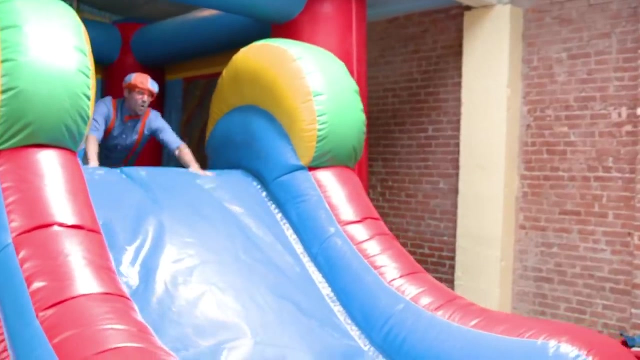 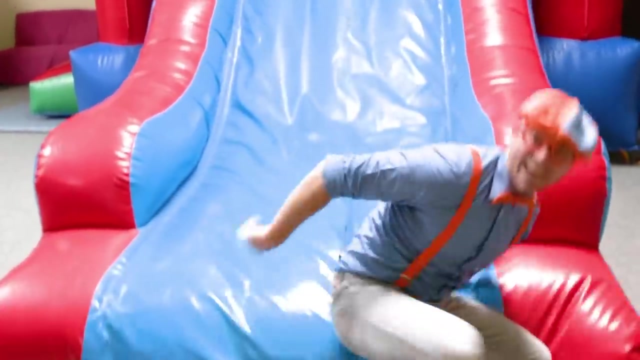 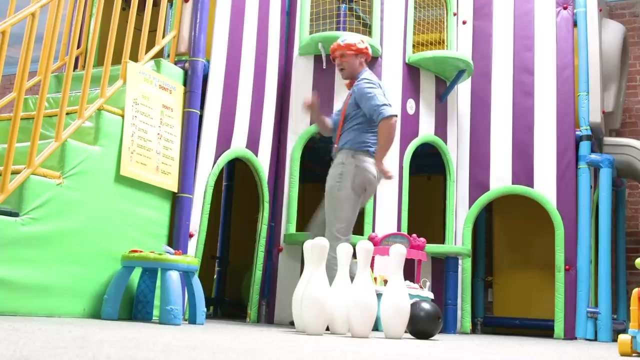 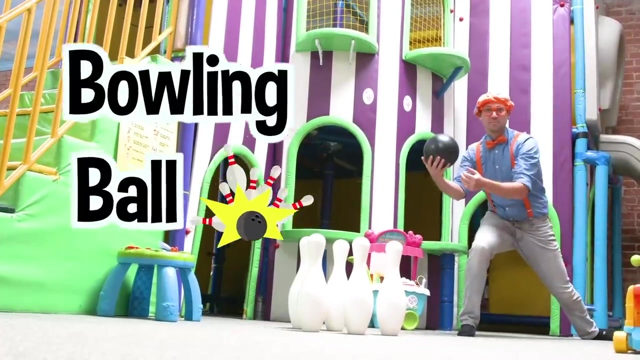 And look at this. This is the color Red. Alright, time for me to go down the slide. Woohoo, Whoa, Here we go. Woohoo, Woohoo, Yeah, Hello, Hey, Woohoo. Black bowling ball. 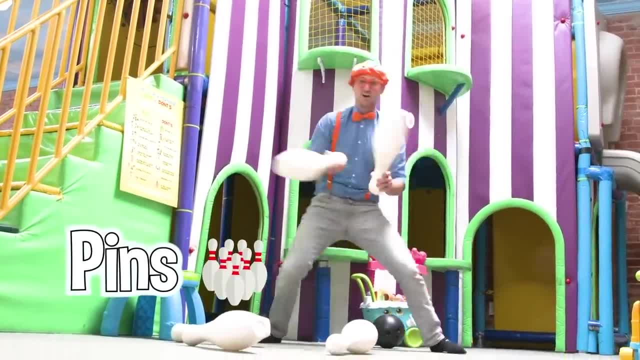 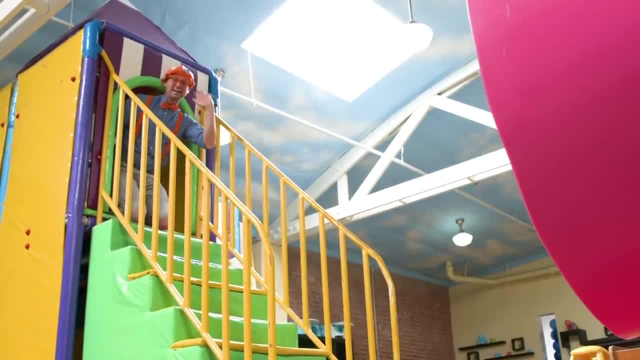 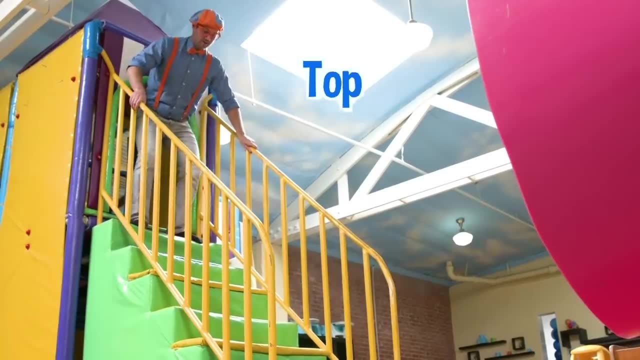 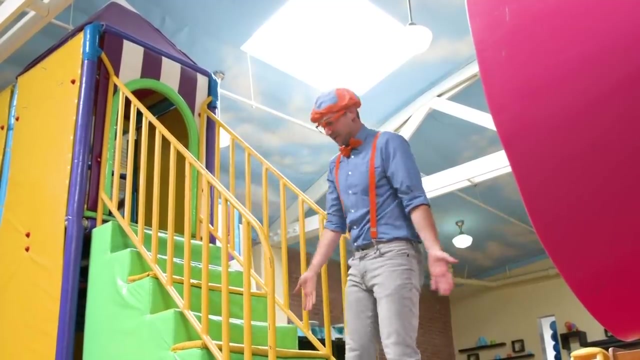 White pins: Woohoo, Haha, Hey, Hello down there. Haha, Look, I'm at the top of the stairs. Now I'm going to climb down. Whoa, Whoa, Now I'm at the bottom of the stairs. 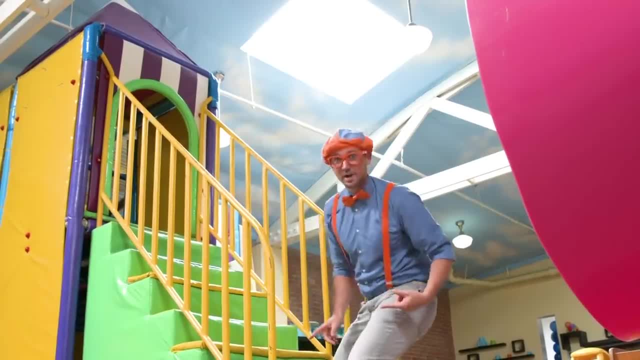 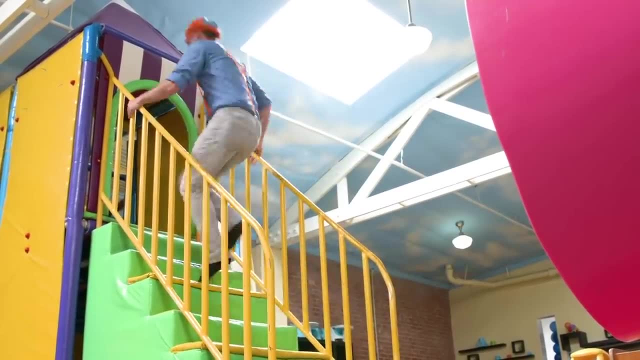 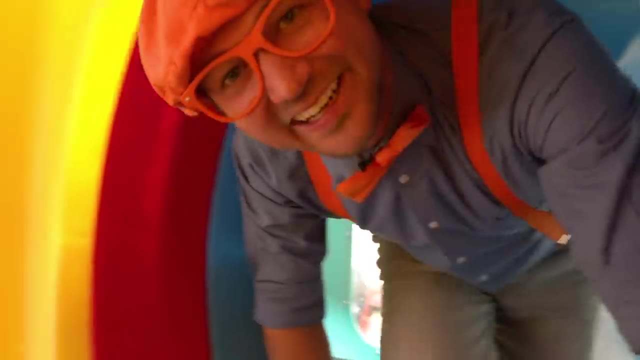 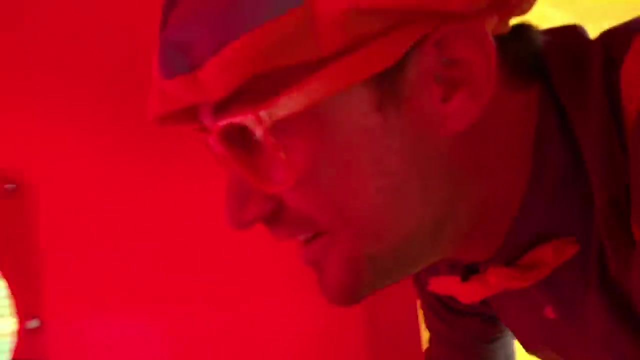 I should probably climb up to the top of the stairs. Woohoo, Bye-bye, Whoa, It's so colorful in here. Wow, I love crawling through these tunnels. Wow, Ooh, Okay, Oh, A slide. 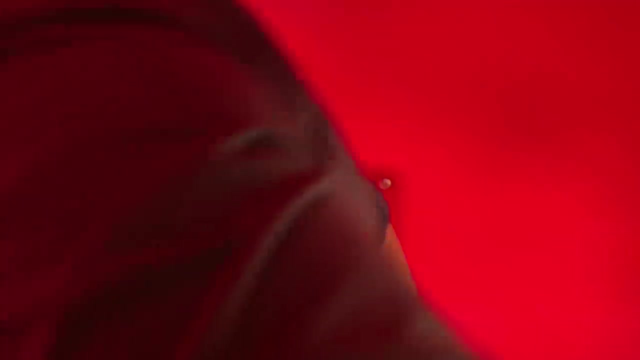 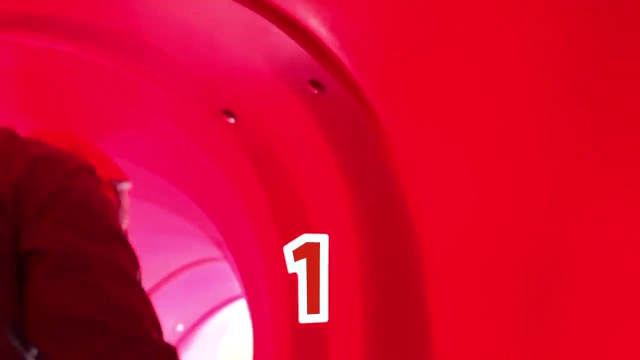 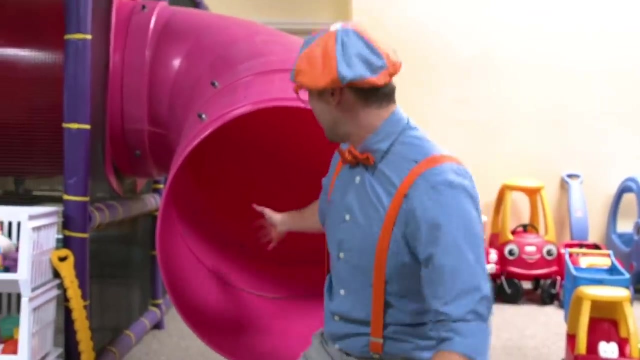 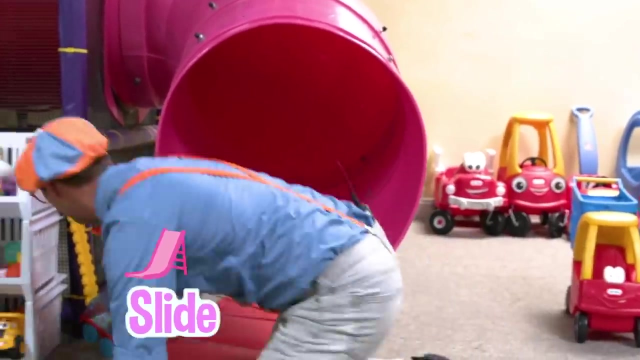 Haha, I'm excited. Woo, Okay, Okay, are you ready? Three, Two, One, Whoa, Whoa, Hello, Haha, Woo. The slide was so much fun And it is a pink slide. Whoa, What is this? 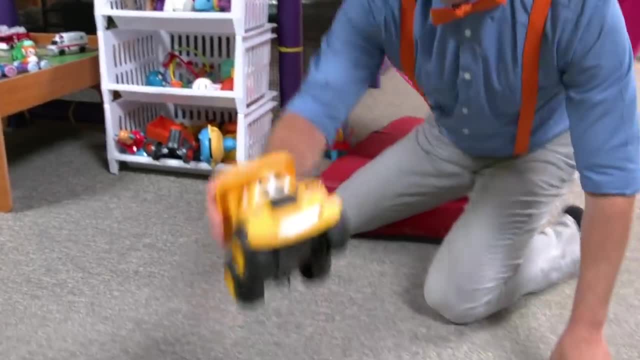 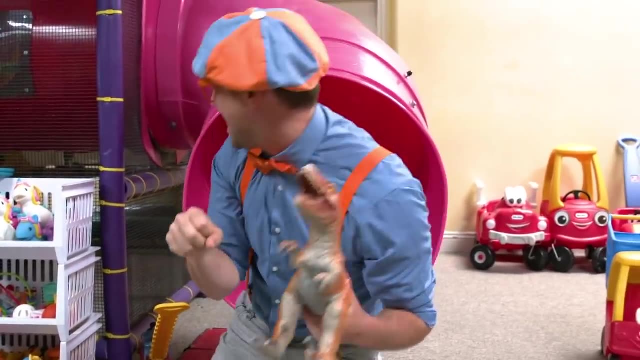 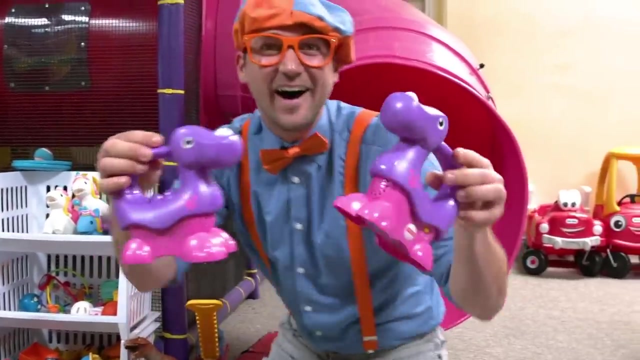 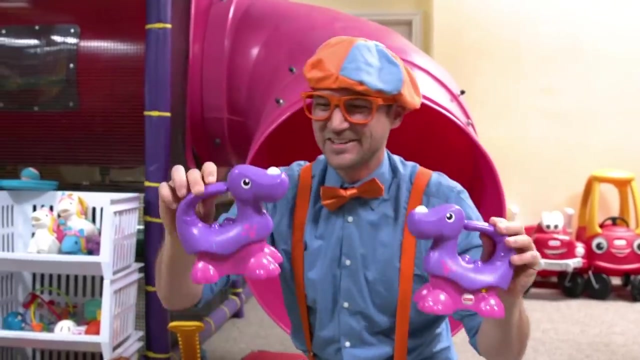 Whee, Whee, Whoa, Rawr, Rawr, Rawr, Whoa. I love dinosaurs. Woo, And look at these toys. Oh, They're so cute. Hello, Hello, Hi. How are you? Haha, So silly. 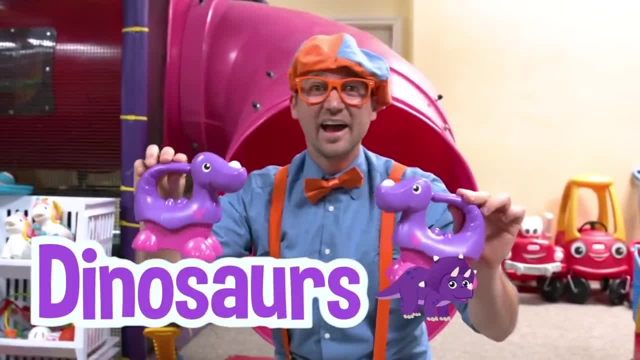 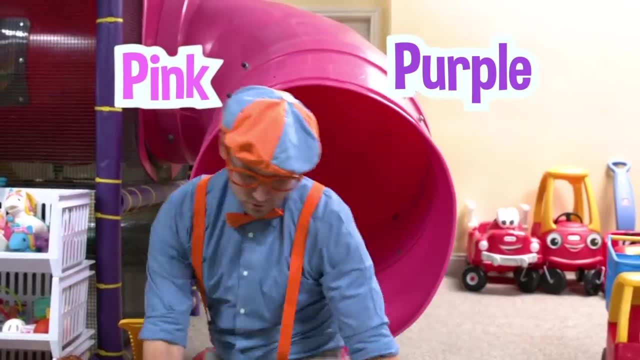 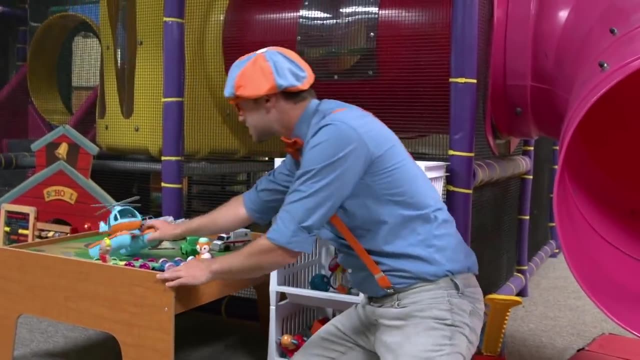 What color are these dinosaurs? Yeah, They are the color purple and pink. Whoa, Whee, Whee, Whee, Whee, Whee Whee Whoa. Look at this, It's a helicopter. Wee. 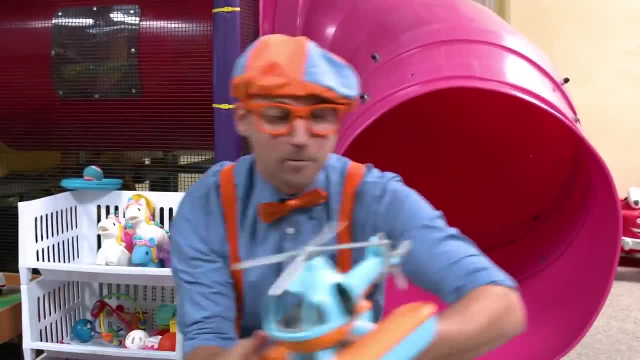 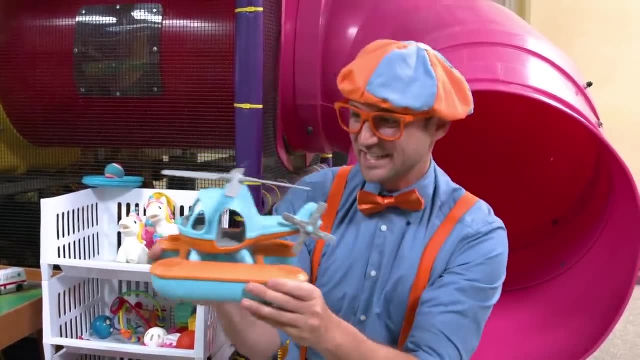 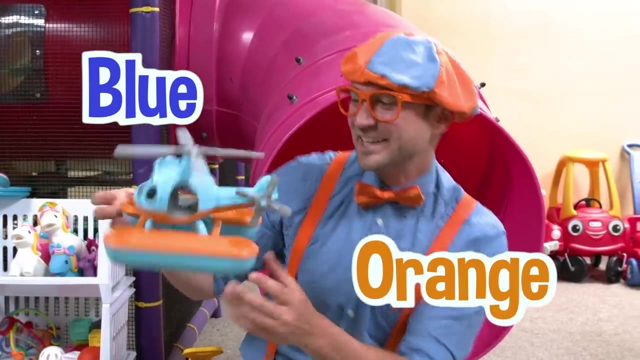 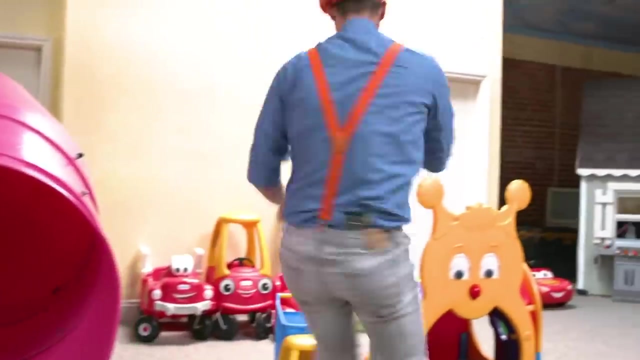 And it is my two favorite colors. Yeah, What color is this helicopter? Yeah, there's two colors: Blue and orange. Woohoo, We'll set that back and go explore. Whoop, Whoop, Whoop, Woohoo. 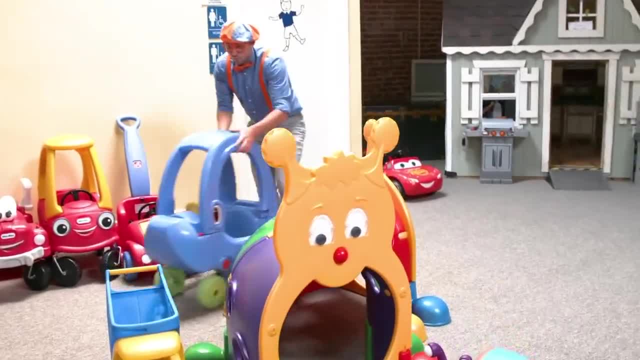 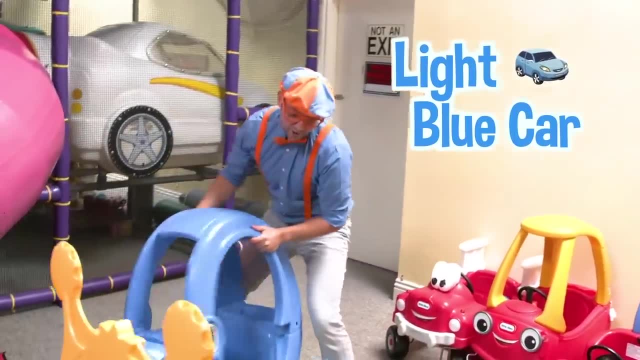 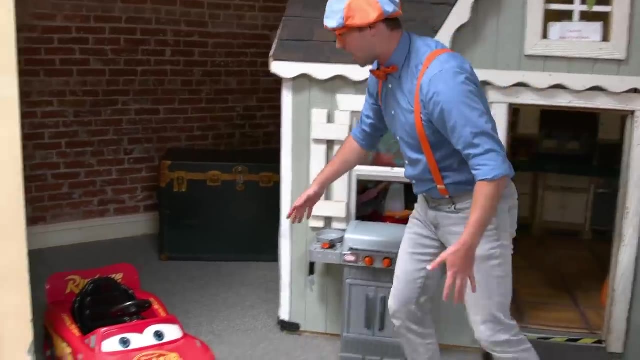 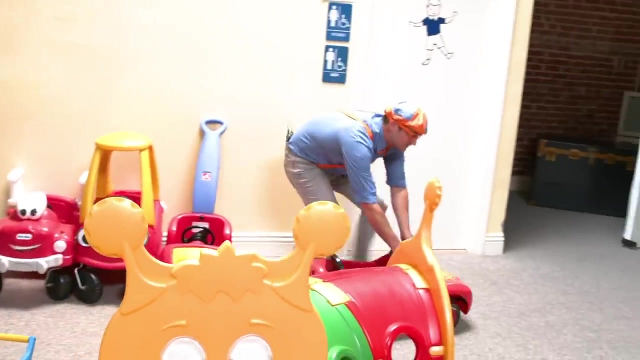 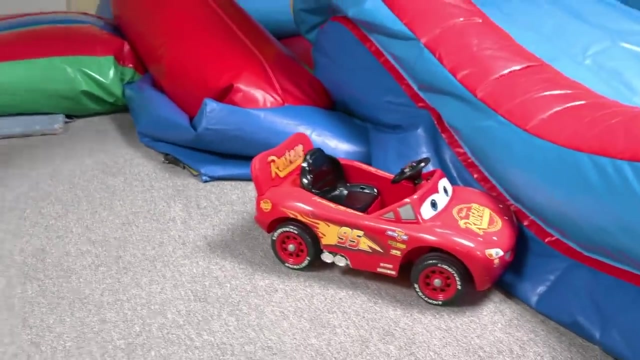 Whoa. Look at this light blue car And look at this car. This car looks so fast. Meow Meow, Meow Meow, Oh Meow, Ha, ha, Woohoo. I love learning my colors with you.